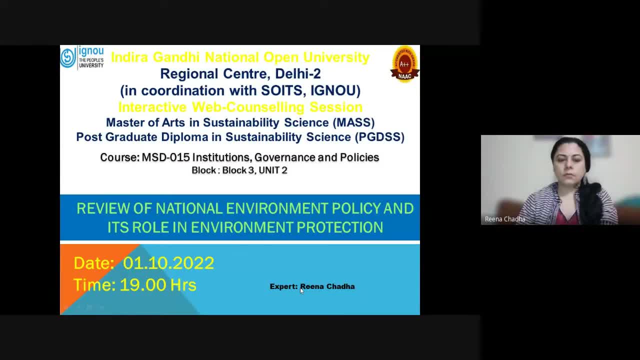 okay, shall I start? yes, okay, so today we'll be discussing regarding the national environmental policies and how those policies are ingrained in our environmental rules and guidelines and what is their role in role in environmental protection. okay, so earlier before this section session, we had attended and we had discussed about the international environmental governance. 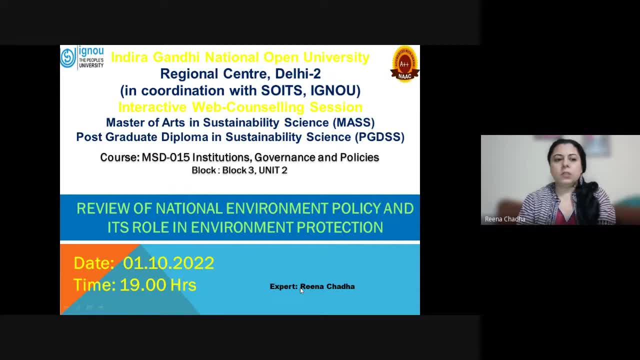 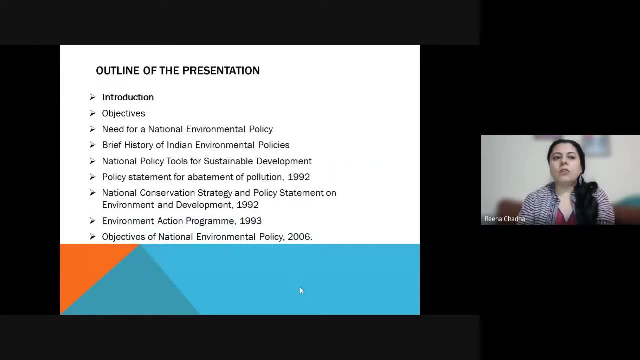 and water, but other policies, how it came into picture, how, what was the historical perspective of international environment governance and how it framed different kind of international environment policies. so our national environment policies are basically a reflection of international guidelines and policies which have been framed and which India is already a signatory to. those 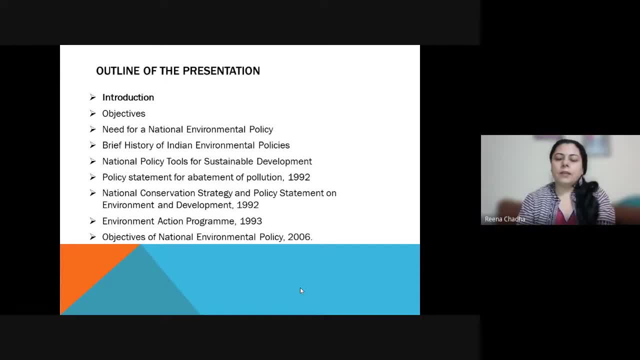 international guidelines and platforms, and that's why we have already started introducing new concepts in our national environmental policies. so in this presentation we'll be discussing about the objectives of this presentation. what are you going to learn? what will be your learnings at the end of this session? then the need of environment policy: why do we actually need to study about? 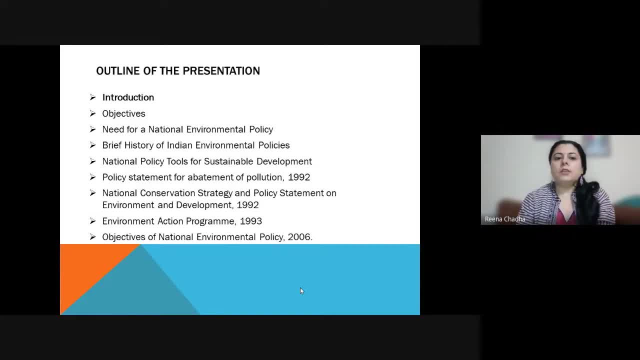 environment policies. brief history of environmental policies. national policy tools for sustainable development. policy statements for abatement of pollution, environment action program. national conservation strategy of and objectives of, national environment policy. again, principles of national environment policies: regulatory reforms, standards, Technologies, awareness, education, information. what is their role in actually actual implementation of these policies? 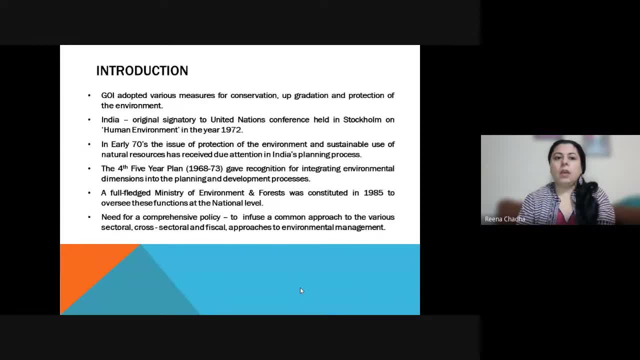 at practical level, on ground, in field. okay, so basically, due to introduction of these policies by government of India, we have to regularly adopt some measures for conservation, Upgradation and protection of environment. so again in, as India is an original signatory to United Nations conference held in Stockholm in 1972, so it is our prior mandate. 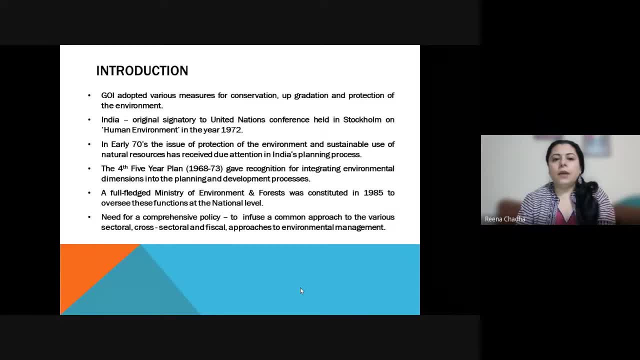 as well as our responsibility to abide by all the commitments we have made as an original signatory to this conference. and in early 70s, the issue of protection of environment and sustainable use of natural resources came into picture due to different kind of pollution related problems. we 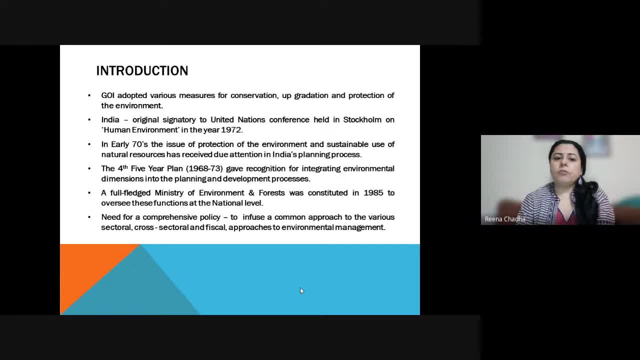 started observing in our environment and before fourth five-year plan in 1968-73, there was a special, specific recognition which was given to integration of environmental concepts into our complete overall planning and development process of our country. so that's why a specific, a specialized Ministry with which was defined. 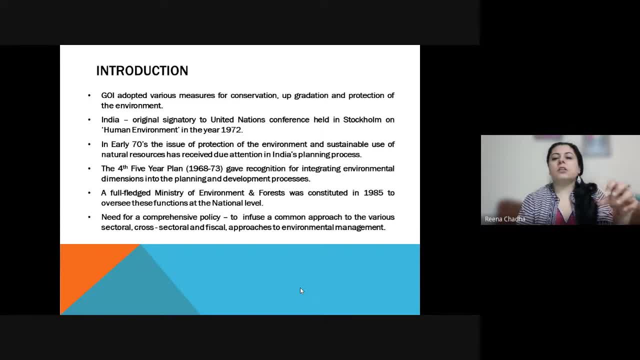 and it was given a task of oversee all those functions of integration of national environmental dimensions into planning process. so, apart from the planning Commission, apart from the five-year plan, this responsible, there was a full-fledged environmental Ministry which came into picture in 1985. so before that there was no single body in our country which was responsible. 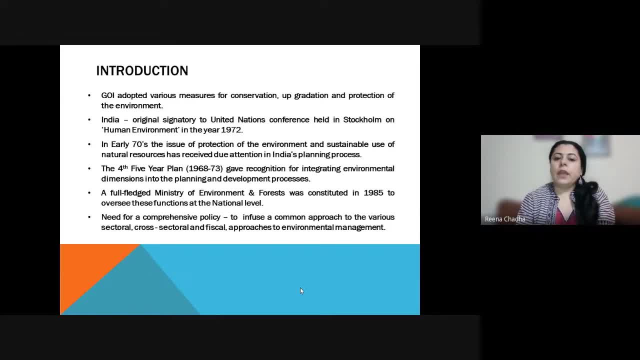 for overall management of environment related issues and thus, as this Ministry came into picture, a need for comprehensive policy was identified so that where all the sectors across the country, be it agricultural sector, be it MSME, be it large scale industry, be it aeronautical industry, be it nuclear industry, be it mining industry, so 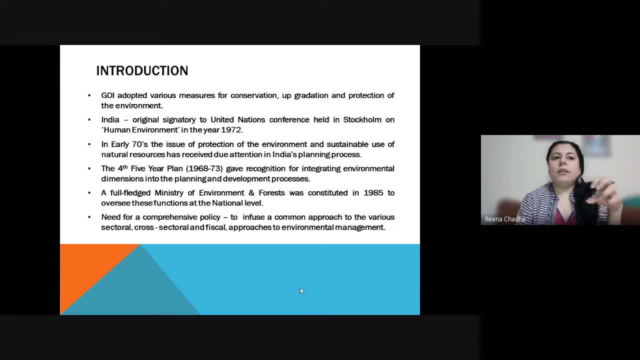 all those different sectors should be integrated and different kind of approaches, uh say, uh economic subsidies related approaches, or monetary, monetarial uh benefits that can would be accrued by Industries sectors and uh the kind of rules, regulations, as well as the fines and fiscal opportunities which can be given to different sectors for control of environment pollution and for introducing better 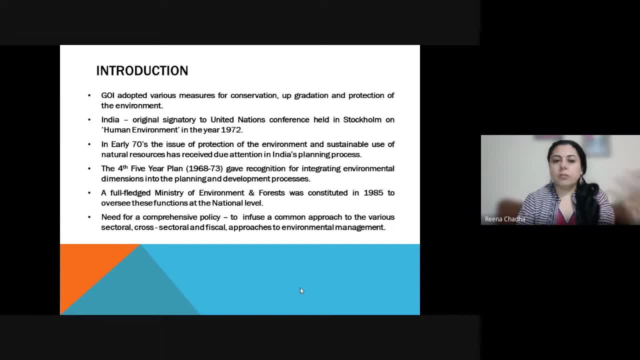 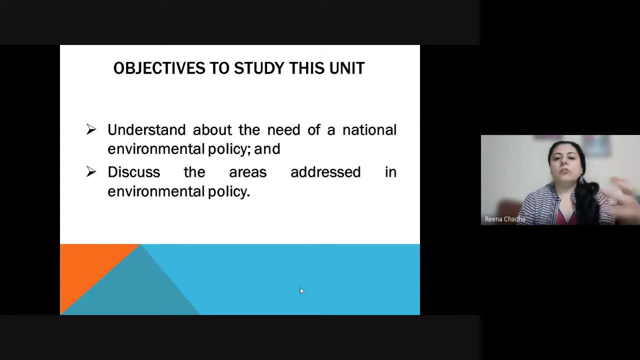 Technologies so that all could be done if there is a comprehensive policy. so that need was identified. so after completing this unit, you will be able to understand what is the need of a national environment policy and how different sectors are interested in this policy. so there was need, because we need to conserve environmental. 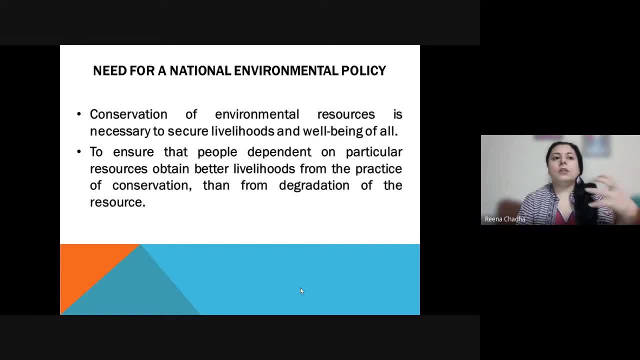 resources. we need to ensure that the people who are directly dependent- the people who are living in rural areas, the people who are living in tribal areas or we who are directly dependent on forest resources for their livelihoods- they should be able to get these resources without any degradation. 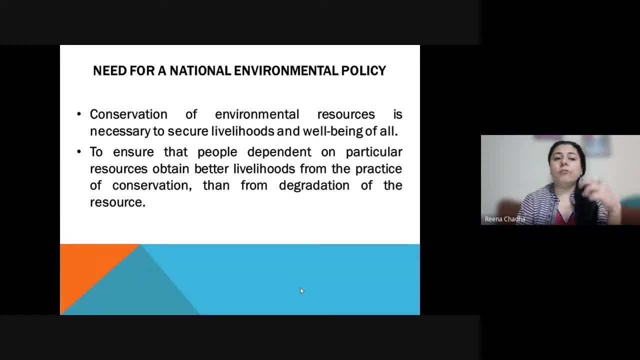 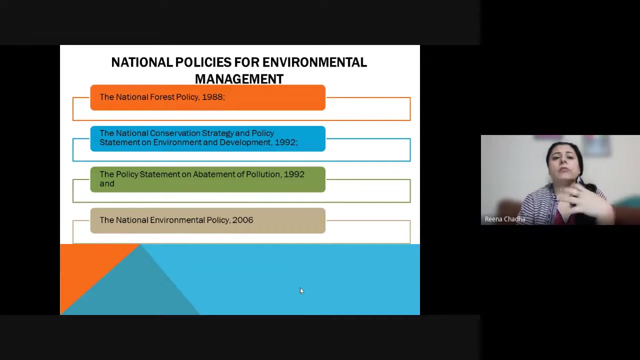 to that resource. okay, so what is the optimal level of utilization of these resources so that there is no extinction of biological species, of medicinal plants, or animals or flora, fauna? so all that need to be regularized. that's why a need for environment policy came into picture. so how this Advent of National policies was done in 1988? National Forest: 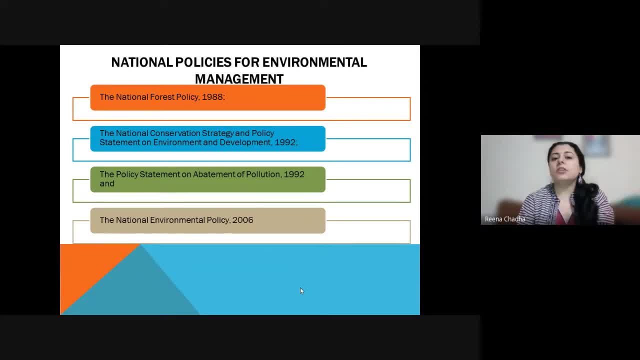 policy came up after that: 1992 National policy and policy statement on environment and development. so other. if you see the names of these policies, then you will be able to understand the objectives and the uh need for those kind of policy statements which which came up in different areas starting from 1988 till now, if you see 2002.. so uh, coming from National. 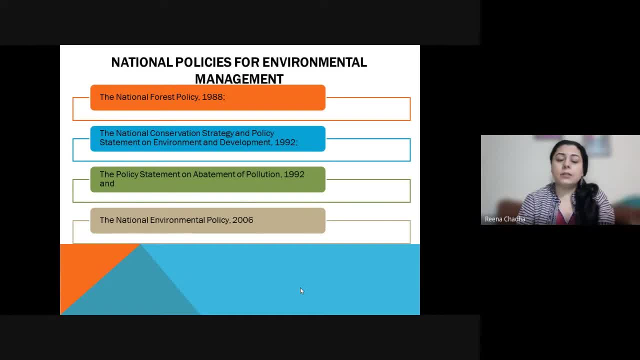 forest policy because in the last lecture we discussed that first national uh forest act came in british era, so at that time there was- the objective was different because british rulers they didn't want it- that these areas should be open to all the fighters or freedom fighters who can find a recluse in these areas, and they can. 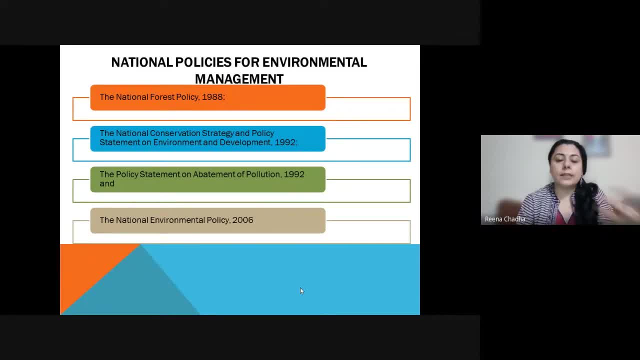 plan, uh, and plan something against them. so, though, for that objective, they wanted that these forests should be secured under their command. but after that, uh come. this boris paul act was again revised to introduce certain measures, so that these- there are some restricted protected areas, reserved areas, 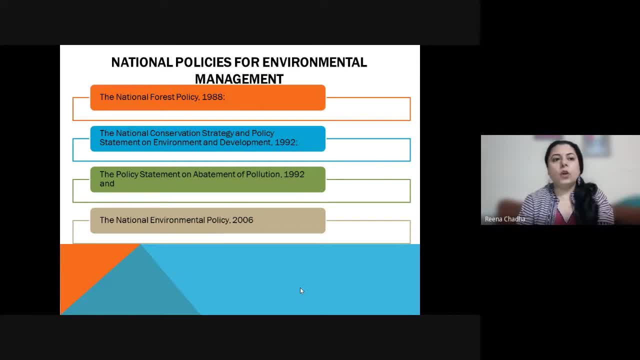 and no land can be declared all of a sudden to non-forest use as well. so all those policies started coming up after 1988, and national conservation strategy was also a part of the national uh platform which was created for environment and development. then came the 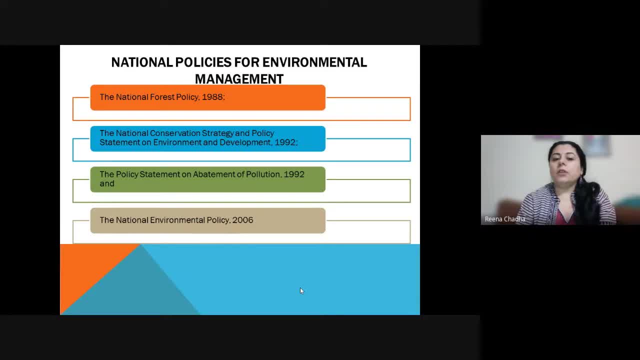 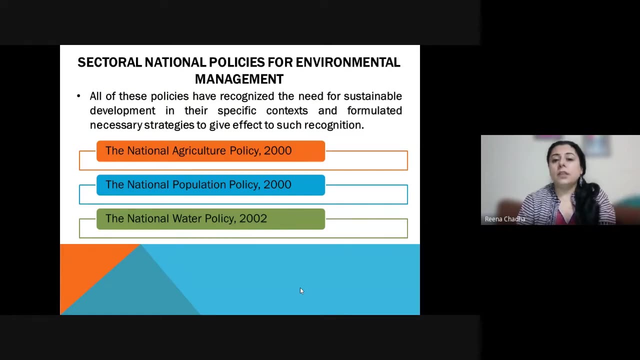 abatement of pollution policy in 1992, national environment policy 2006, which also gave a new uh look to our environment impact assessment notification, which again came in september 2006. again, national agricultural policy was framed in 2000, which is a very recent policy. national. 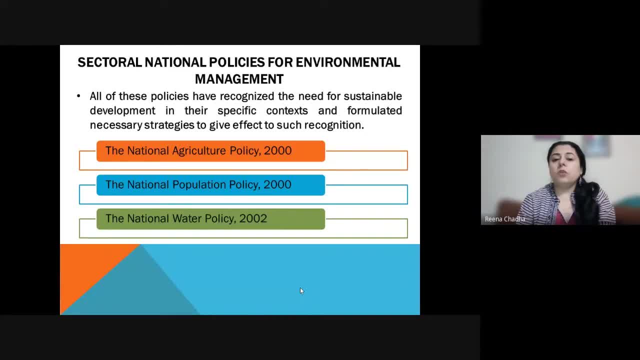 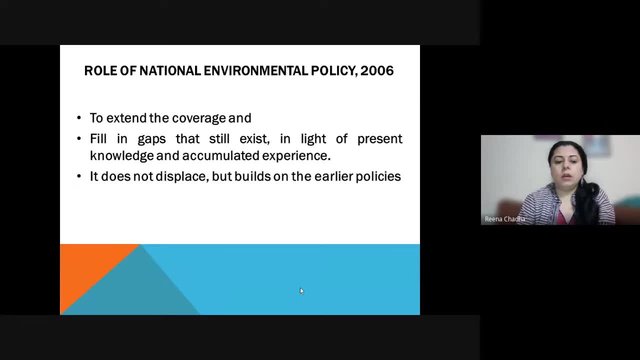 population policy, national water policy came up in 2002.. so, again, the role of these policies is wherever they find a gap in some kind of issue that needs to be resolved, in environmental context, in pollution context, in sustainable development context that needs to be filled up. so whenever we find any gap, we need to. 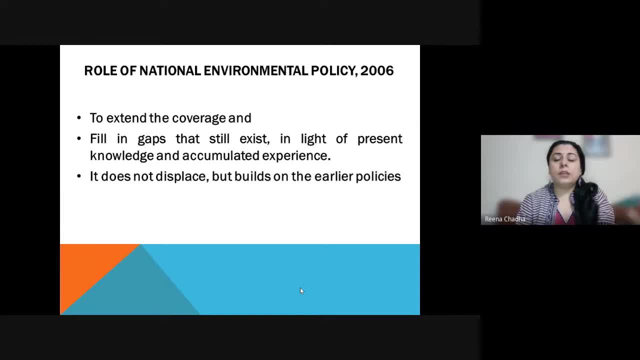 fill it up through a proper policy. policy is basically an an outline of action plan, our principles or our philosophy on which our activities can be based, which can be implemented in ground okay. so it does not always displaces the old policy. so whenever some new policy or some amendment comes up, it is basically 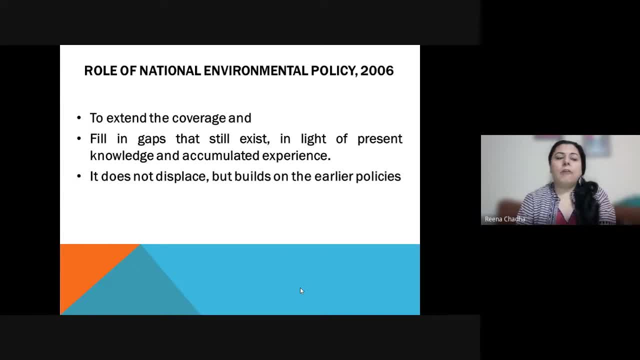 to build upon the earlier policy, to give it a strength and to fill up the gap which has been found during, uh say, for example, our legal dealings of these issues on daily basis. for example, if ngt would have done a different kind of Geo strategy, which would have been a different kind of plan. 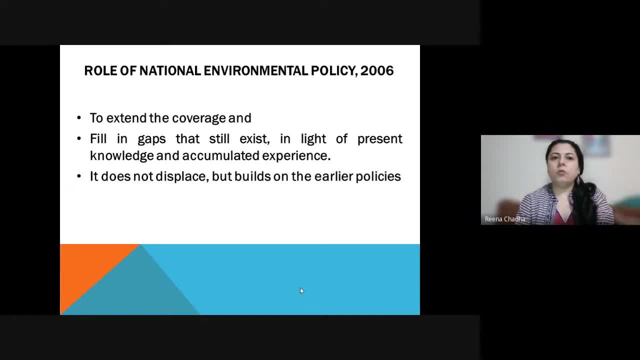 now. these are some of the major things that this district government is working towards, and the reality is north favor Gear bear doing a new policy because they hope that these Rapids gas projects and the current raising levels will ensure that those gas stations will go up into另外 마 mitigation option. um, so that was our crusher. 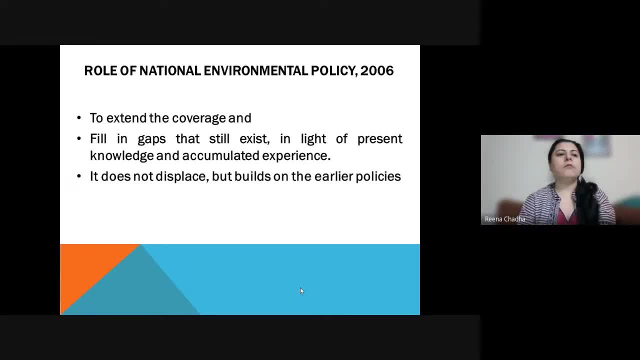 on the related 40 state and the pace sustainable management تم providing their pieces of land on in small sizes so that they can get those clearances at district level. then again, we we identify. okay, this gap needs to be filled up and people should not go. 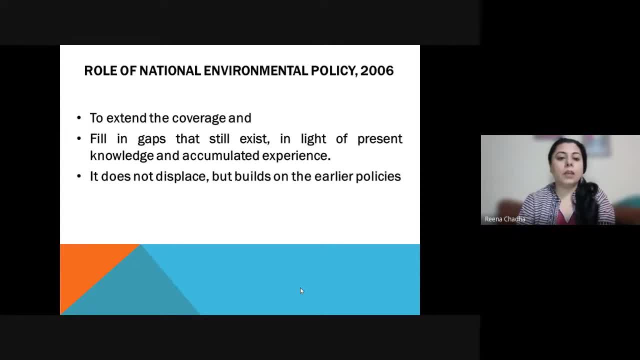 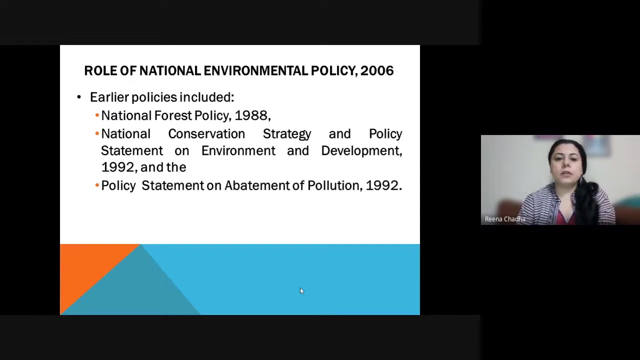 for smaller pieces of land and do mining without getting any clearance. so again that gap is filled up with a new policy or new amendment with better strength of dealing with these kind of cases against control of environment pollution. okay, so earlier policies included national forest policy, national conservation strategy, policy statement of on abatement of pollution and historically, if 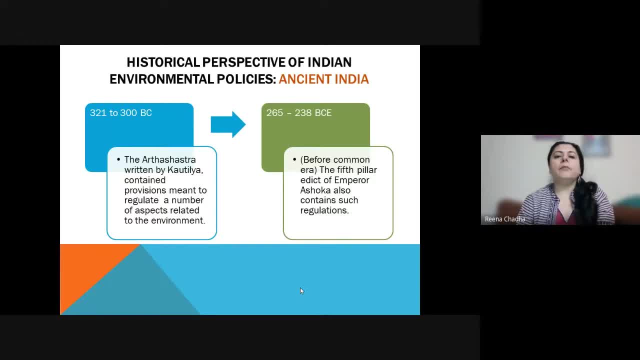 we see, it started with the ancient india period, with 321 to 300 bc and with the writings of art shastra, written by cortelia, and it contained specific provisions which meant to regulate anambulance of the environment and to regulate the environment and to regulate the environment. 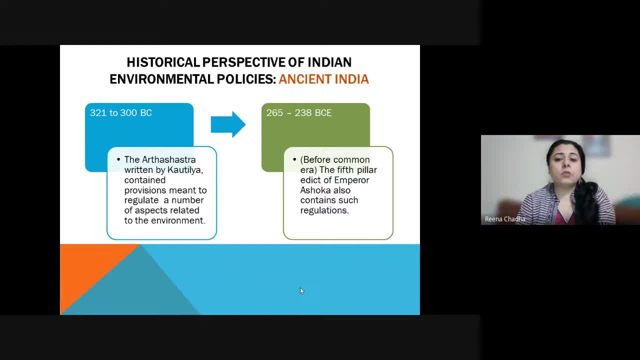 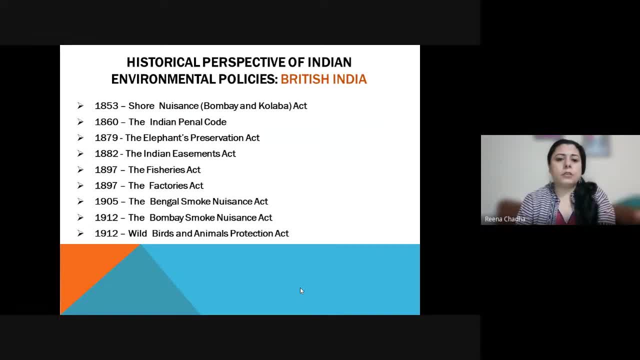 we note down, all those kind of uh acts and policies came into picture in british india era only so, starting from 1853 when we had this shore nuisance act and then in 1912 we had bird birds and animal protection act. so this regulatory provision of environment. 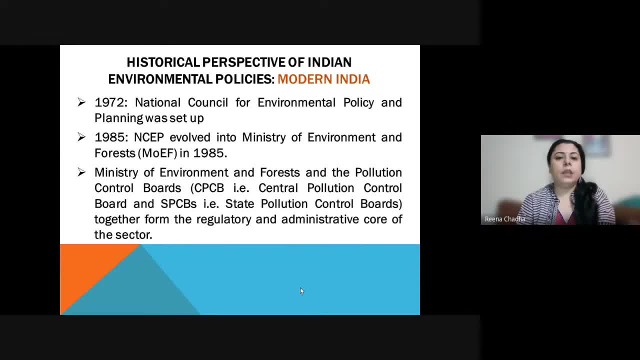 protection came into picture well earlier in india. okay so, but actual implementation and actual bodies which needed to be created for institutionalization of these, uh, implementation activities, that came into picture quite later. so that was the reason why, in spite of having so many environment policies, we were not able to get the get any results on ground, because the implementation. 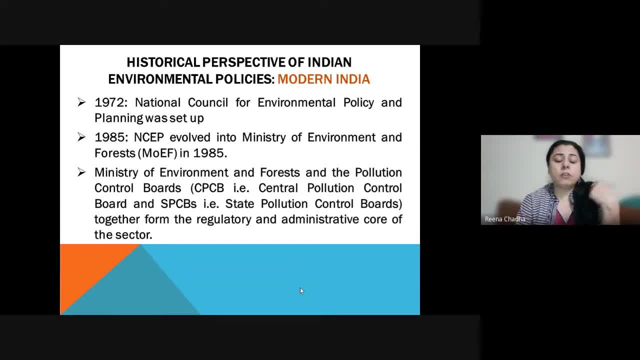 part was lacking: the body which were, which was required to implement these rules, regulation was lacking. okay, so in 1985, when uh, ministry of environment and forest was evolved and then ministry of environment forest further identified central pollution control boards, state pollution control board. and which kind of people, what kind of 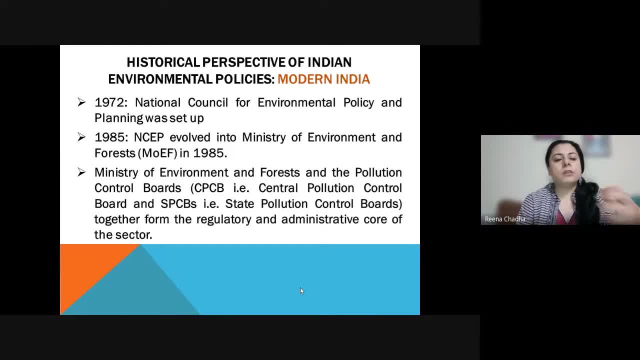 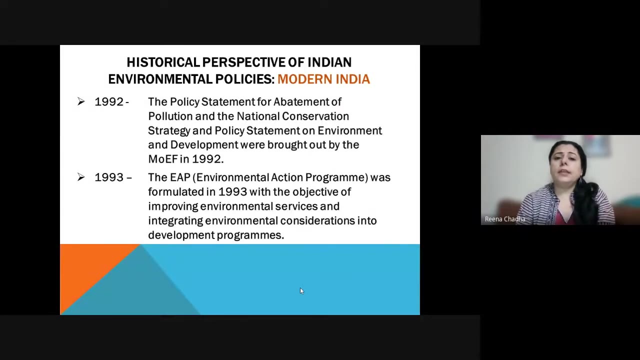 team can be recruited under these boards? what will be their specific designations, their eligibility criteria, their experience of work? those all kind of measures were again given in environment impact assessment notification. so again they together formed a regulatory and administrative core for every sector. okay, so this 1992 policy. it gave a strategy on 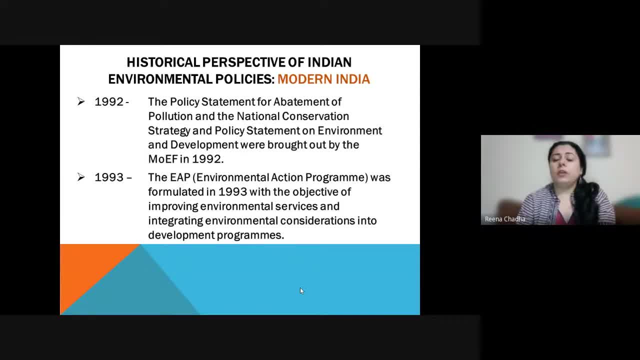 environmental development which can be brought out by moef in 1992, and then environment action program was formulated in 1993 and that program is still continuing. if you see, uh, if you go to school level, if you go to community level, there are national environment awareness activities. 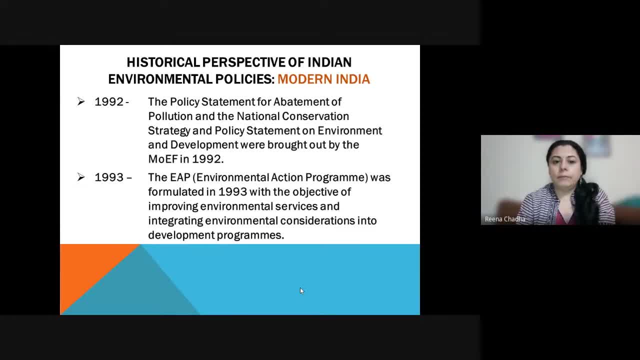 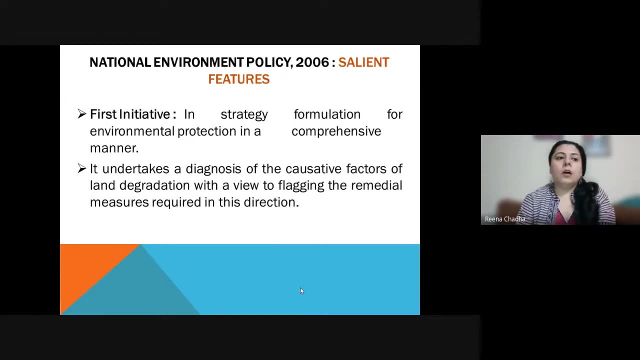 which are going under that program since 1993. okay, so many uh ngos. they are acting as nodal agencies for implementing, actually implementing these programs at local level, at regional level. okay, and i have been fortunate to work, uh, with few of these ngos in the initial stages of my 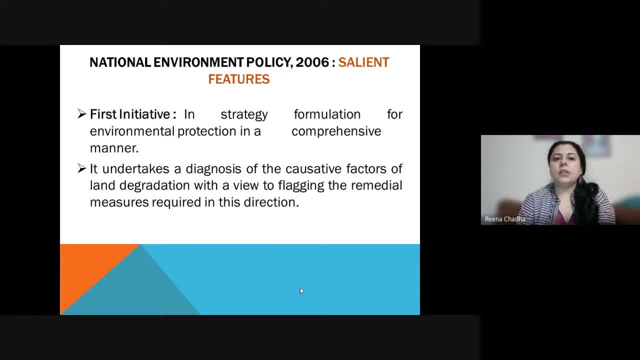 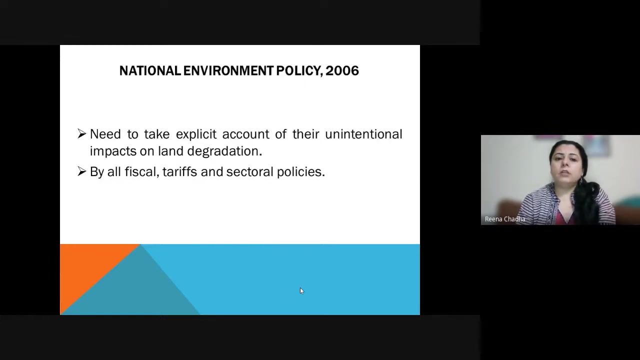 career. so uh again with first initiative was started in strategy formulation for environment protection in a comprehensive manner. again it started national environment policy: diagnosed what are the causes which cause land degradation, which uh which can be flagged so that the remedial actions can be taken. uh, accordingly in that direction. so in national environment policy, 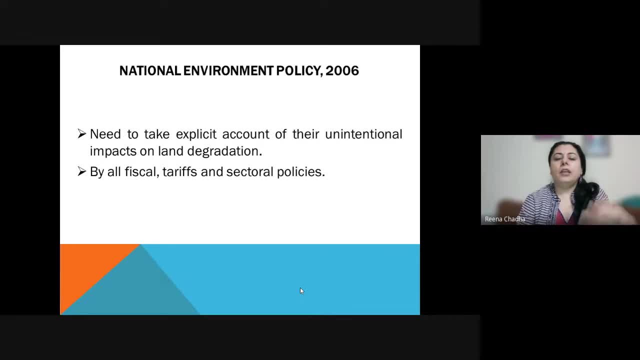 there was an explicit account whether there have been an intentional impact on landing radiation degradation or an unintentional, unconscious impact. so all those uh actions needed to be taken into account so that we can identify specific policies which can give you better benefits if you take care of the environment as well as your development or the industrial. 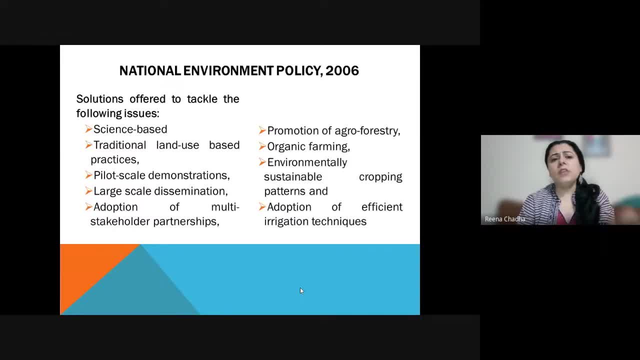 development in your area. so national environment policy. it basically identified solutions which are science based which can be used on to as uh in align with traditional land use based practices which can help us in uh, identifying pilot scale demonstrations which can help us in large scale dissemination of information, like your swashta swachh bharata. 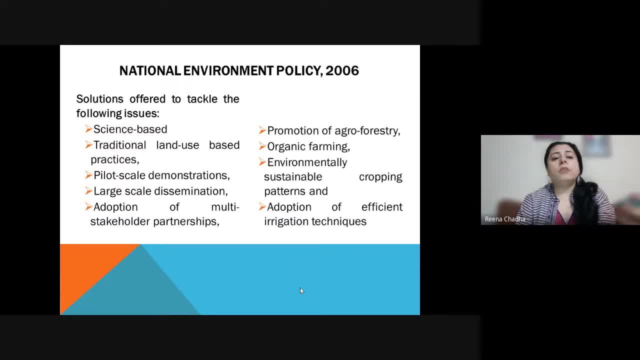 biyan formation at a very large scale, right from the top to the bottom at the local level. okay, so then, adoption of multi-stakeholder partnership, like ppp. public private partnership was introduced, government and geo partnerships were introduced, rnd and scientific development partnership were introduced by dst, and promotion of agroforestry was introduced. watershed management product. 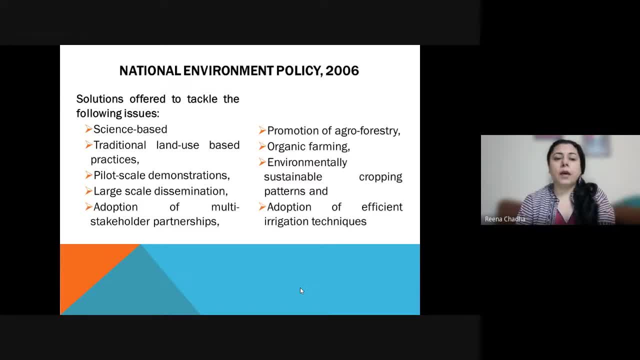 projects were introduced by agencies like kapat. okay so again, organic farming, environment, sustainable cropping patterns like krishi, vigyan, shetra were introduced. okay, so, all those uh different sectors were incorporated and different policies were integrated so that the comprehensive uh objective of achieving environment uh protection of environment. 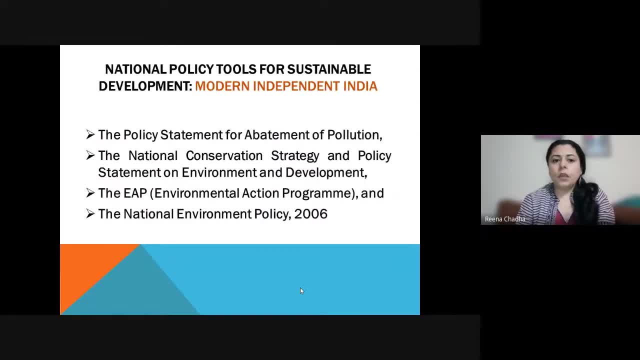 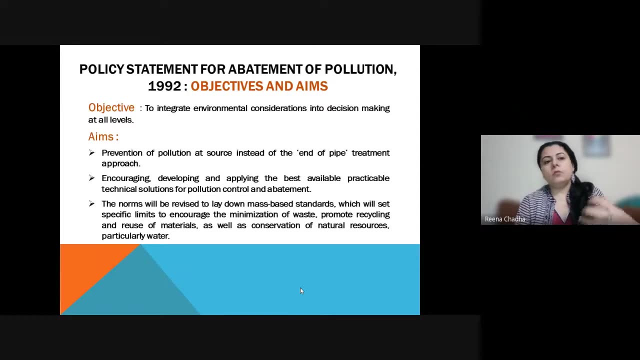 and sustainable development can be done. so in modern india. again, we have already discussed. all these policies came up right from the policy statement for abatement of pollution till national environment policy 2006. so what are the objectives now we come to? we have uh discussed regarding the need of these policies. what were the agendas which were to be addressed? 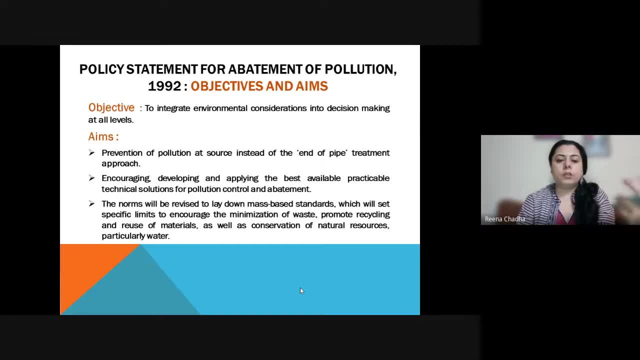 by these policies, how these policies came into picture from the british era till now. so now we'll study what are the objectives and aims. so a objective is to integrate all environmental considerations into every kind of decision making process. we do at every level: local, regional or national level. so we, whenever we define any developmental activity, any kind of 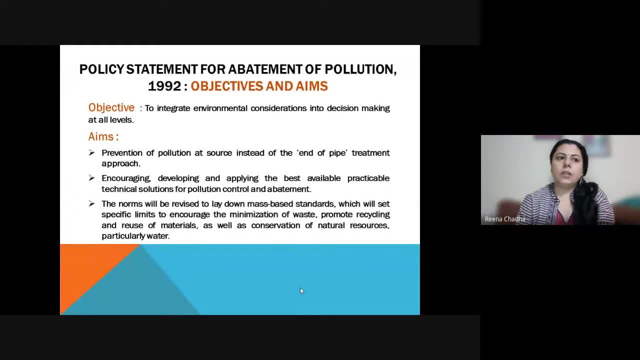 industrial project or any kind of uh project related with agroforestry or organic farming. our key issue- uh issues- are the development of agroforestry and the development of agroforestry are. the projectCTs are the followings: the production of agricultural production in the 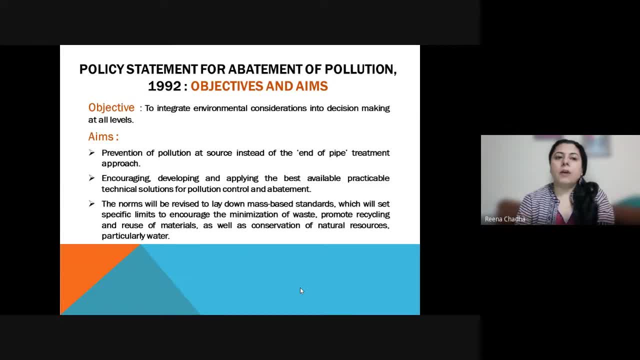 device of the laboratory and the production of the agroforestry system in the fuel and water supply system is an idea. another issue, or our key concern, should be to ensure that it is environment conscious, it is environment friendly and it is sustainable in a longer term. okay, so that is objective. again, if you see aims, what are the specific aims? to prevent and of pipe treatment approach: okay, so we need to stop pollution at the source. that is why we always talk about uh, an installation of effluent treatment plant in the industrial, going to try and address this issue to encourage an evidence funding, goaling that diversity is an issue also. we saw the effort from the issue of environmental systems in particular, large scale and does not account for the objective objective of妨���tment, weifsau or the possible stages of표vement. 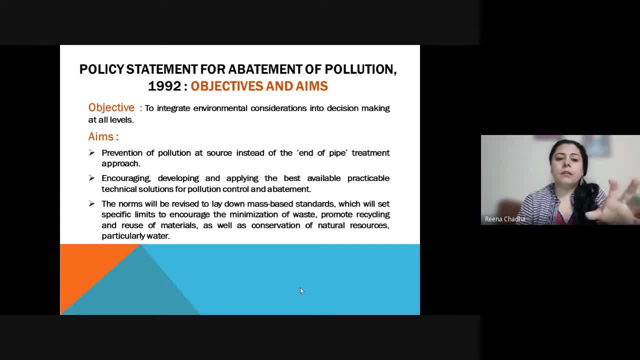 itself to ensure that there is a waste segregation at the household level itself, okay, so that there is no large scale uh problem created which cannot, which is difficult to be resolved, which needs lot of resources. so if we prevent any pollution related problem at the source, it reduces the 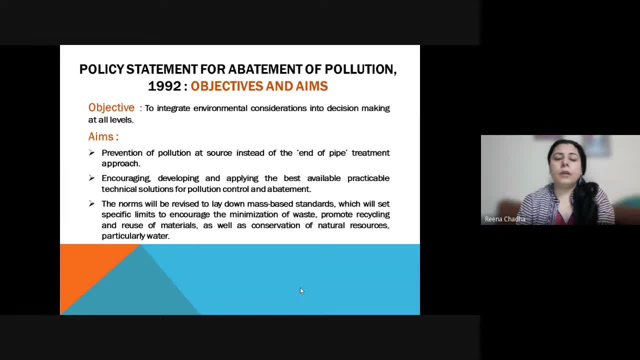 amount of energy, amount of in financial resources, amount of technological uh advancement that is required for resolving that problem. if we do not solve it at us, so at the source itself. for example, if an industry does not employs uh, etp, effluent treatment plant or stp at the industry. 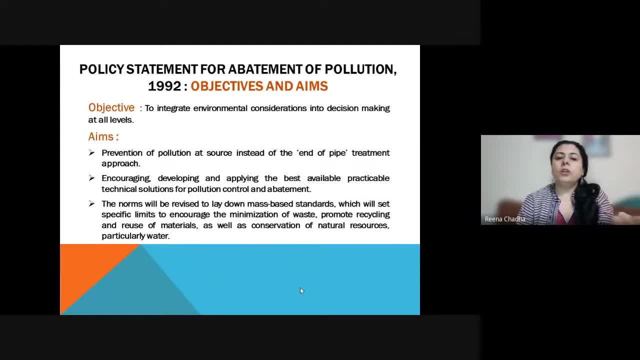 level itself. rather, rather than going for pollution at source control approach, it goes to end of and discharges all of the water into a river stream. so that way it is polluting a large volume of water in a river and again threatening- uh, threatening- and posing a health hazard to the 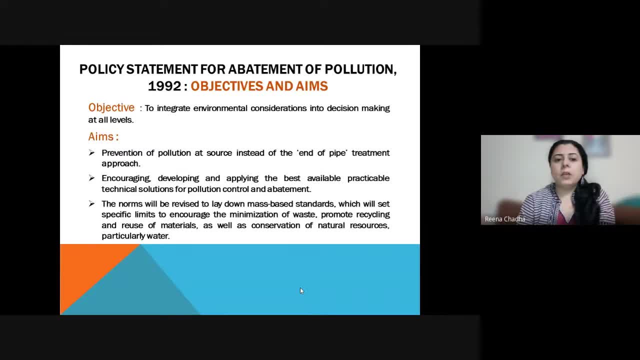 population which is connected to that river stream. so that problem goes to larger dimension if it is not treated at the source. so that needs to be our first aim. okay, then again, encouraging developing the best available practical technical solutions for pollution control. so that was our second aim. 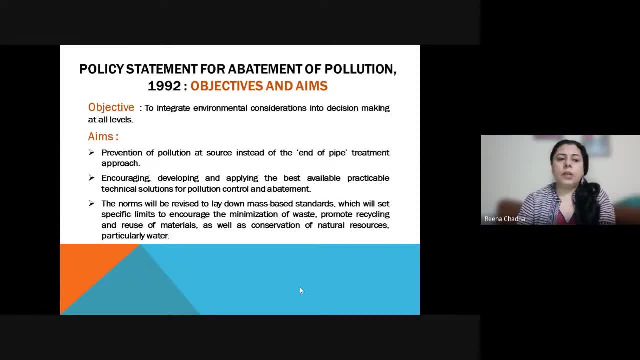 so that nobody should uh deter from taking up some new technological advancement help and introducing it into their industry. for abatement of pollution. again there were mass-based standards which were revised, and then the specific limits were encouraged to minimize the waste, to promote recycling, to use materials and to conserve natural resources, particularly water. so before that water was not. 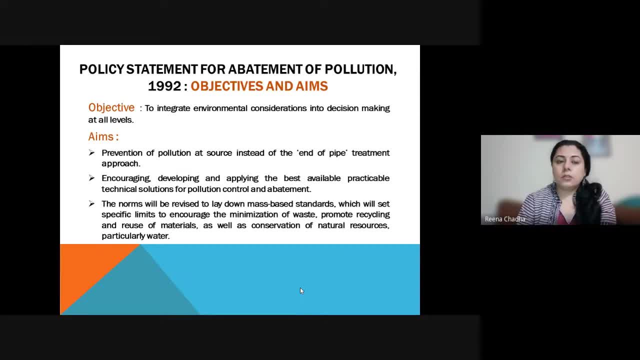 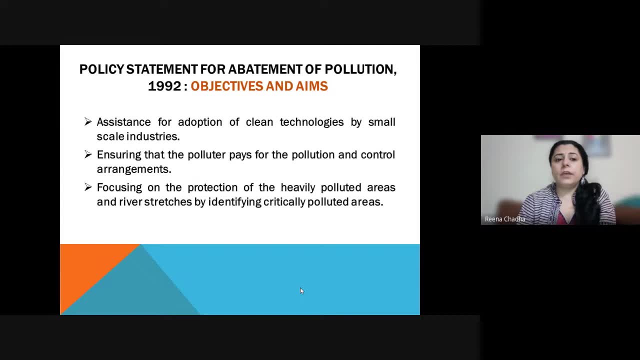 a prime issue which was considered in conservation of natural resources. again, assistance for adoption of clean technologies was one of the aims and ensuring that for all the polluters who are creating pollution in the environment, in the society, they should be paying for that pollution created. they should pay for the 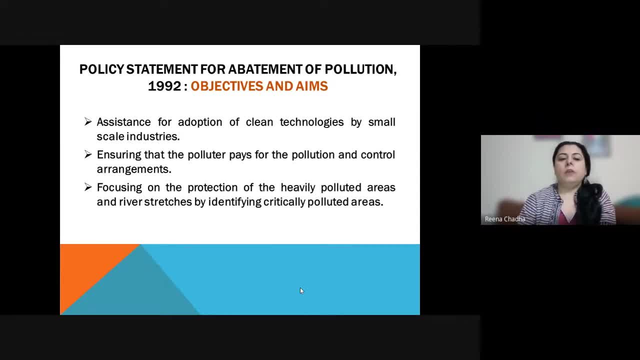 environmental Quality, rise of environmental policy and the community should be paying energy too. they should takehalts or anything people should be paying to rebuild the places which are active in. like yourself, i understand i will have been talking about the ownership change, but i would say that what is being done in the environment for there is, there is no. 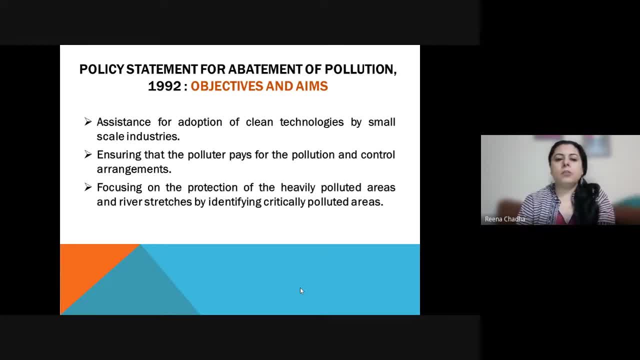 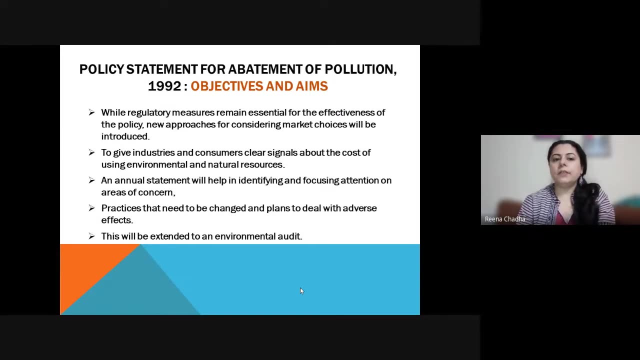 restriction on soil, one doesn't really matter. but that, what is simple and i do want to put into aggression effect. thank you, these objectives and aims, okay. so again, there was a name, that regulatory measures that remain essential for the effectiveness of the policy, and there should be clear signals for industries and 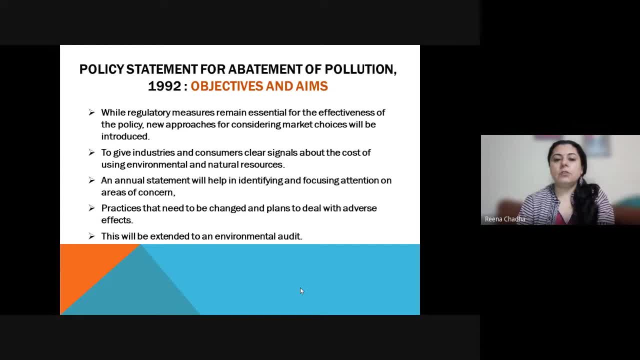 consumers about the cost of using environment and natural resources. they should not feel that any environment resources available free of cost, so that's why specific charges were levied act was created, water sex act was created and there was an annual statement that was required to be submitted in the name of environment audit and in the form of form 5. okay, that form 5 needs. 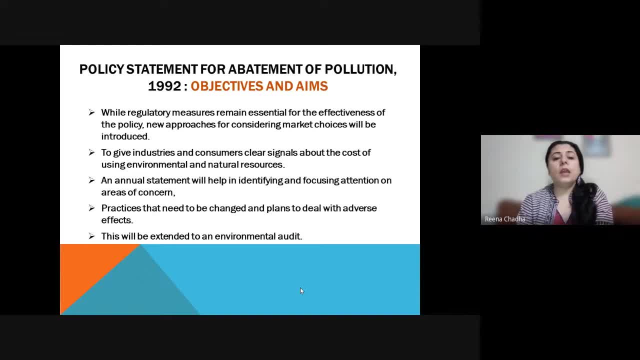 to be filled up under the environment audit requirements so that there is an annual statement of what kind of specific pollution. specific pollution means per for per unit of production: how much pollution is being caused, how much water is being caused being used, how much hazardous waste is being generated, how much sludge is being generated? 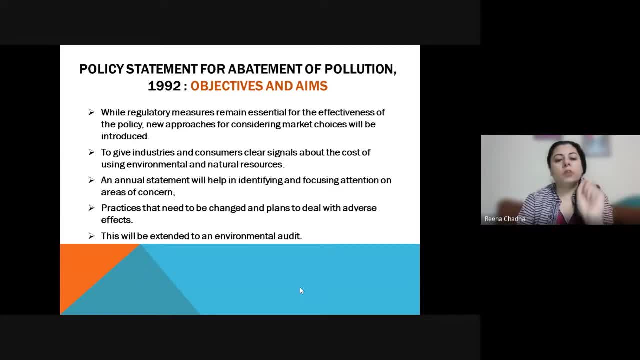 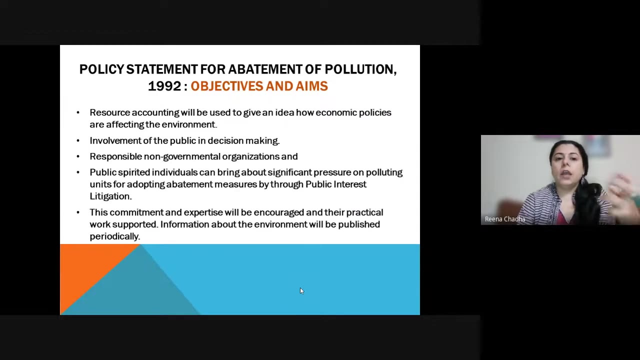 waste water is being generated for every unit of production, for every meter of cloth manufactured, for every kilogram of steel manufactured, for every unit of power generated for any kind of industry. okay, so that is a specific utilization of resources and that annual statement takes care of that in the form of environment audit and again we have to do resource accounting. 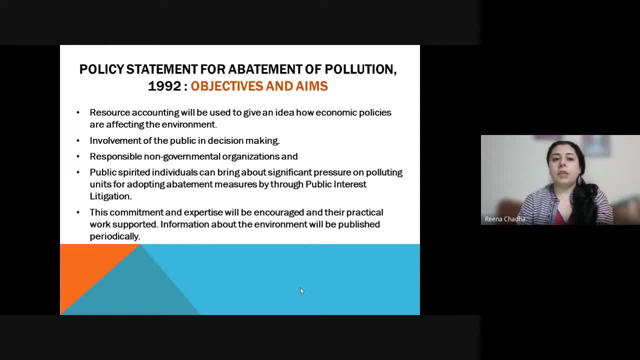 we have to involve people in our decision making process, especially women and children, all who are most of their times. they are deprived of basic resources. they should also be involved in decision making process and this commitment should go to the local level so that all kind of information which has been published in the environment domain, that should 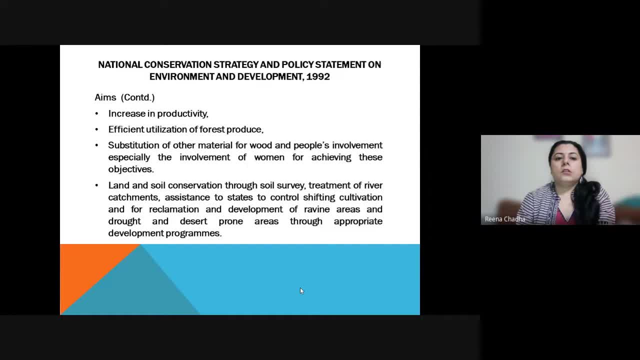 reach to the communities. okay, so again, if you see all these uh aims, they are correlated with each other and if we are able to implement the aims we have discussed, we will definitely increase productivity. we will increase utilization of forest produce in a more efficient manner we can. 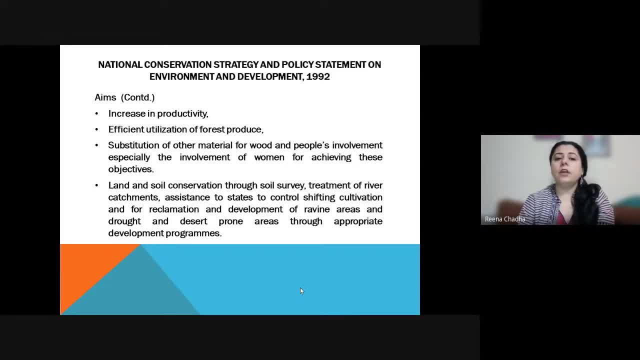 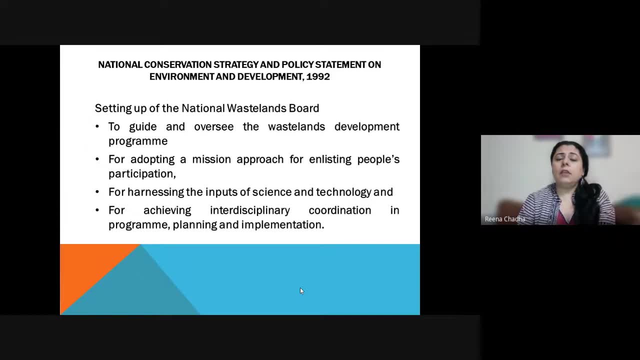 ensure that our land and soil is conserved and we are getting enough resources for our communities. okay, so again, uh, they, they were, uh, there was a at aim of, and establishing national wasteland board under this policy, so that all the wastelands that have been created in the naturally or man-made they should 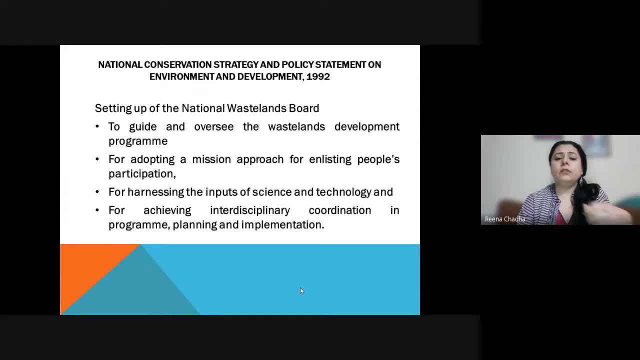 be, uh, remediated, they should be, they should be harnessing of inputs from science and technology to ensure that these wastelands are developed in some manner and they should be utilized for, uh better, uh, environmental resource development. okay, so again, there has to be promote, promotion of. 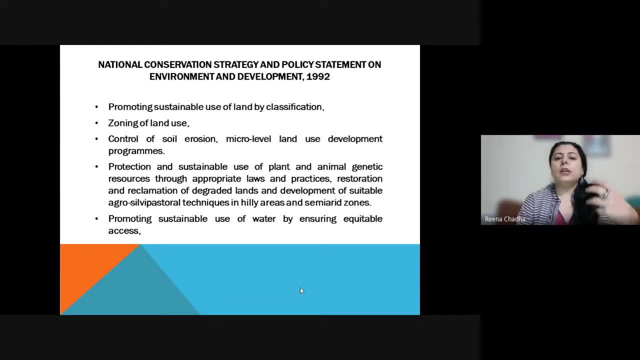 sustainable use of land by classification and control of soil erosion, zoning of land use. so before that, uh, if some industry needs to be established, any kind of land could be used. but after zoning of land use, if you, if you want to construct a building on an agricultural land, you have to take a clu, clearance of land use. or 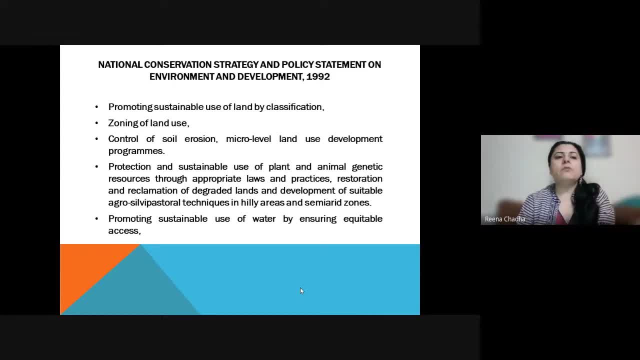 or you have to get the land transferred from agricultural to industrial or construction. uh use of land. okay, so all those uh things can come up now. special economic zones have been created under zoning, even for groundwater also, groundwater mapping has been done for different areas and over exploited zones, and exploited zones and dark zones, as well as safe zones they have been. 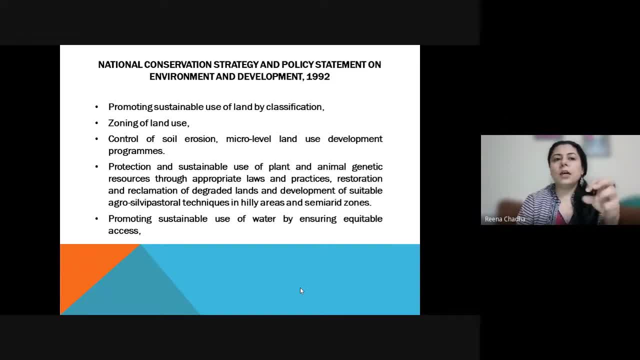 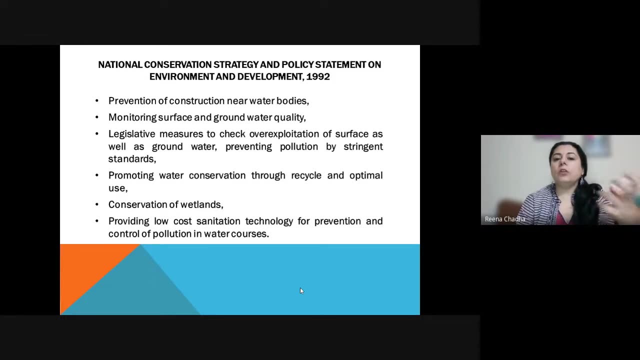 categorized. so all these policies are now in place, so not just for one sector. so all these aims are also not for one sector. they have to be implemented sectorally in all the different sectors. okay, again, we have to prevent construction near water bodies. so again for that: if we don't have a policy statement, we cannot frame laws and acts without. 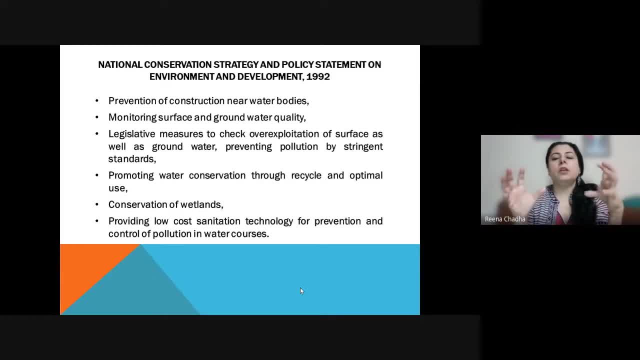 a policy. so if we have a basic framework of policy, okay, this is our aim, this is our objective now, our now, our acts and rules are are all should be aligned according to this policy statement. that is the purpose of policy statement and defining all these aims under policy statement. 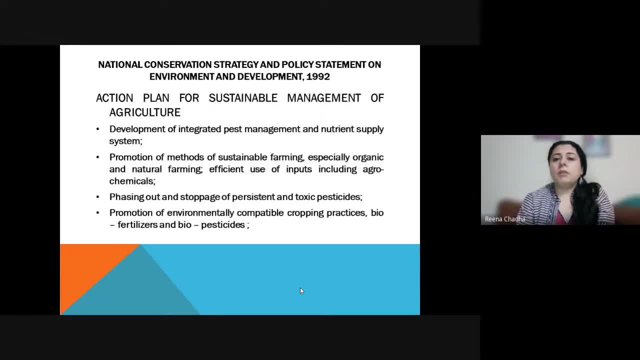 so again, uh, an action plan for sustainable management of agriculture was framed, wherein we have uh identified integrated pest management and nutrient supply system, so for agriculture also the water management system, in order to meet these initial imbalances. there are no й сейфа гранавки зигнинг аль-бана станил цынаада. 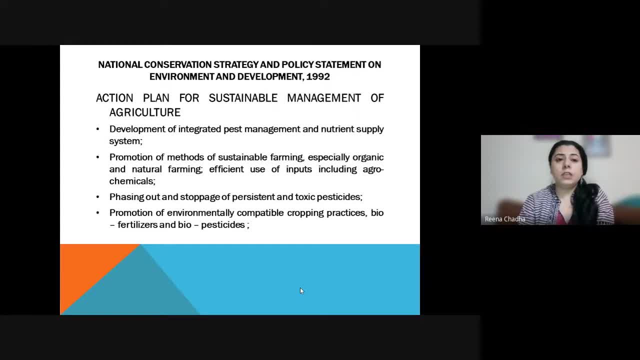 inneh cта-yоєсy, כاؤс cта-yоєсy- in our rivers or in our ponds, at local level or in rural areas. also, all ponds were being converted into lands because of the issues related with eutrophication, so that again is linked with. 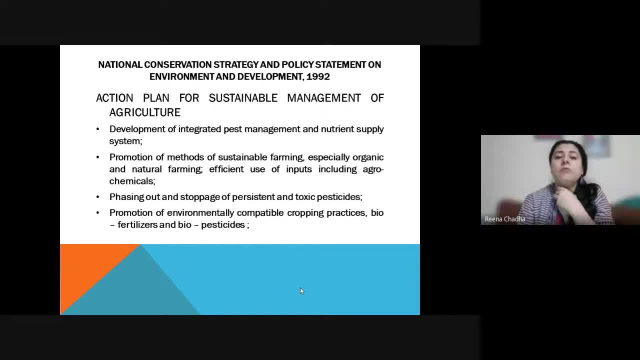 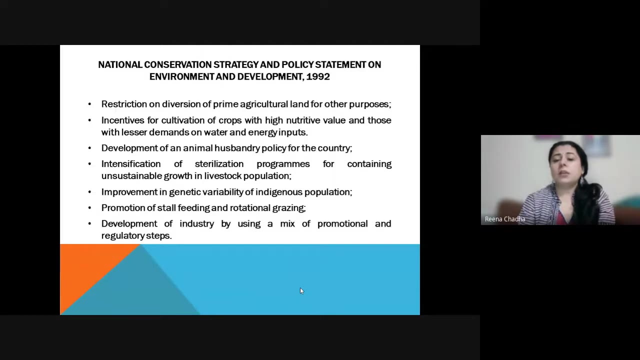 persistent and toxic pesticides which are very much rich in nitrogenous and phosphates, and they are having recalcitrant compounds which cannot be degraded easily through natural environmental cycles and processes. so that was the reason why these persistent and toxic pesticides were phased out again. there was a restriction on diversion of prime agricultural land as per the zoning of 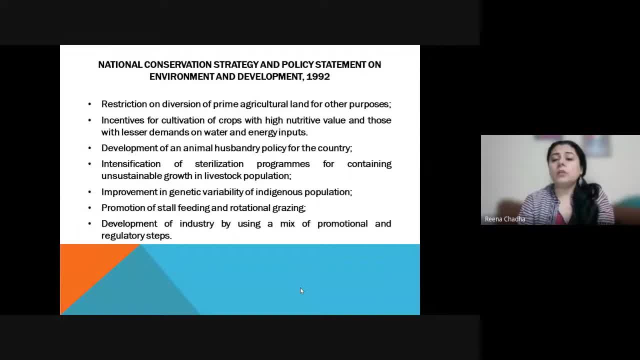 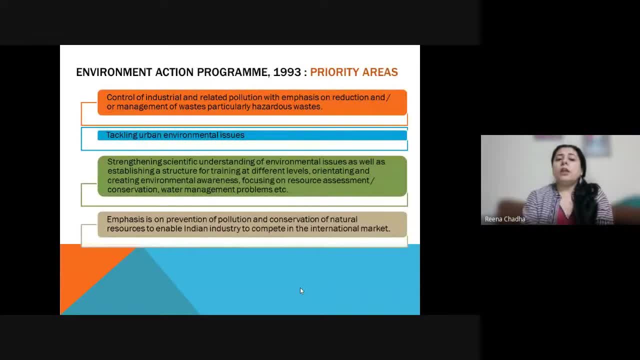 land use and animal has been. husbandry policy was introduced, improvement in genetic variability was introduced. so then comes your environmental action program in 1993. so priority areas: there were four priority areas basically. so the first was the control of industrial and related pollution. then was tackling of urban environmental. 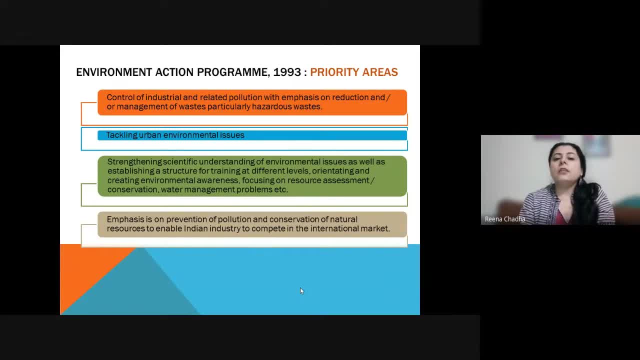 pollution problems. okay then, third was strengthening the scientific understanding of environmental issues, because at that time, in 1993, our scientific understanding of environmental issues was lacking due to lesser r&d done in these areas, due to lesser projects which were implemented for understanding of environmental issues, and 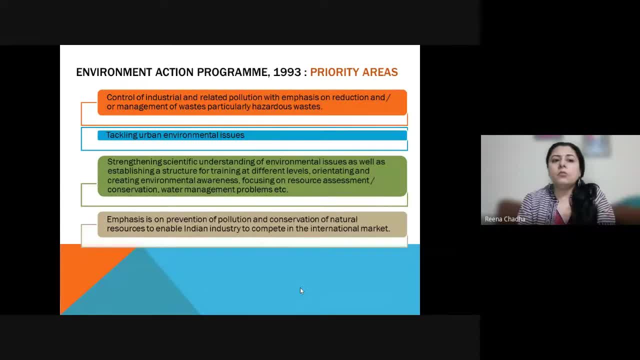 lack of even uh. the courses on environmental programs, like our educational and professional uh courses, were also lacking because there was no specific information or no specific guided structure of curriculum which which could teach how environmental issues need to be tackled. so professionalism was not there here. in scientific understanding, again, there was emphasis uh on prevention of pollution and 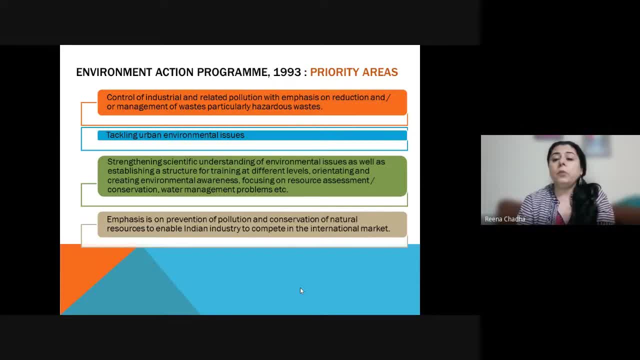 conservation of natural resources so that we can compete with the international markets. for example, if in a pharma industry, if you are not having a who compliance or GMO certification, good manufacturing practices, GMPs are not introduced, then you cannot trade with any. you cannot export your pharma. 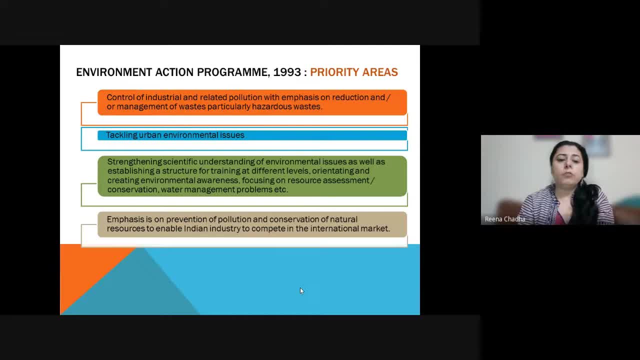 product to any international market. so if you have to grow, then also you need to prevent pollution and conserve natural resources and understand and international environmental uh acts and guidelines and all kind of voluntary standards like ISO 14 000. so what can be implemented? what needs to be adopted to place yourself at an international 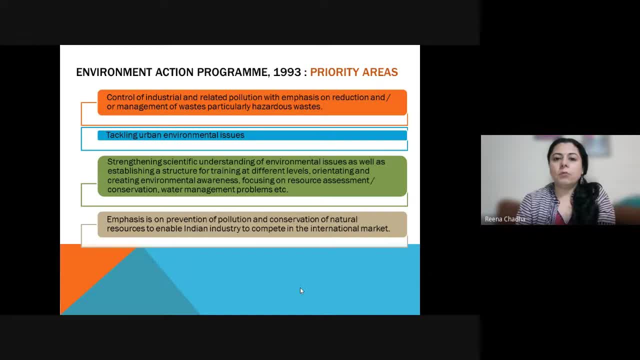 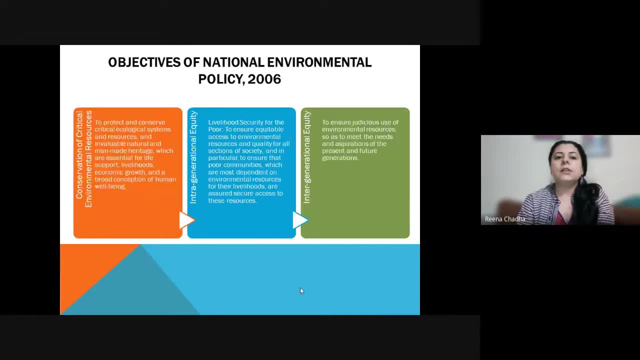 level. that was again emphasized under environment action program of 1993.. so the uh, after discussing the priority areas, we will discuss what are the objectives. okay, so first objective was conservation of critical environmental resources, resources which are restricted in amount, resources which are unreplaceable, resources which can, which cannot, be recovered again in a short period of time. so 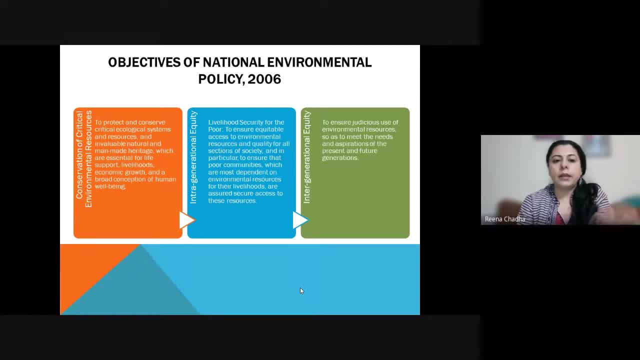 those resources need to be identified and recover or reserved as well as conserved. then intra-generational activity- uh, equity, sorry. so intra-generational equity means you have to have equitable, equal access to environmental resources and quality for all sections of society. it should not be the case that people living in slum areas- they can be. 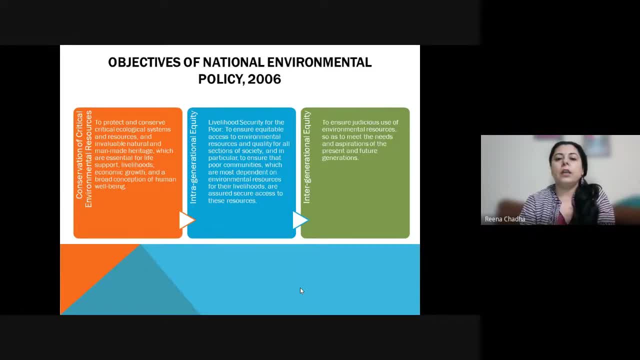 deprived of good air or what good water quality and people who are better, well off and living in poverty and air quality. so there has to be equitable distribution of environmental resources and if some uh and community is being deprived of those resources, uh based on their intra-generational 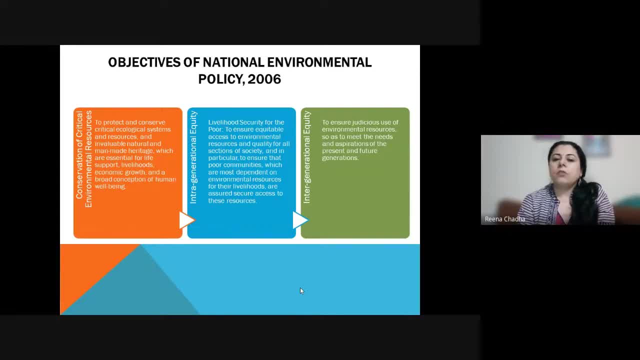 disparity. that should not be the case. so again, intergenerational equity, intergenerational. we have to ensure that our present generation, as well as future generations, are getting equal benefits. there is an equitable distribution between present and future generation. it should not be the case that present generation completely uh utilizes and 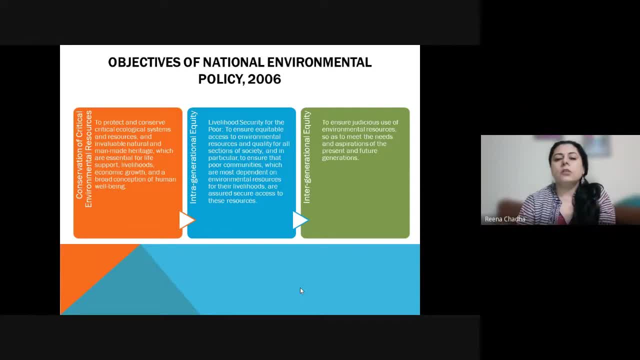 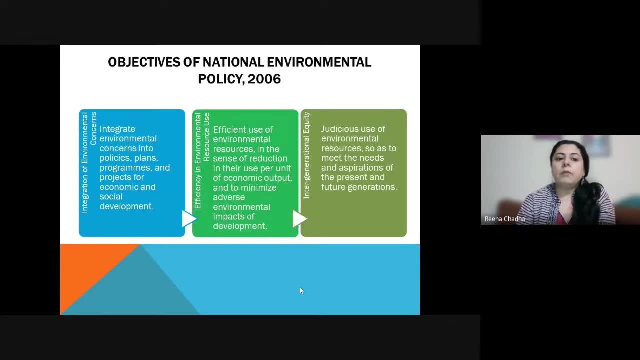 exhausts is exhausting all the resources and those resources are not available. in future, that should not be the case again. integration of environmental concerns- as we have already discussed that was again a part of national environment pollution abatement policy as well then efficiency and environmental resource use should be done. 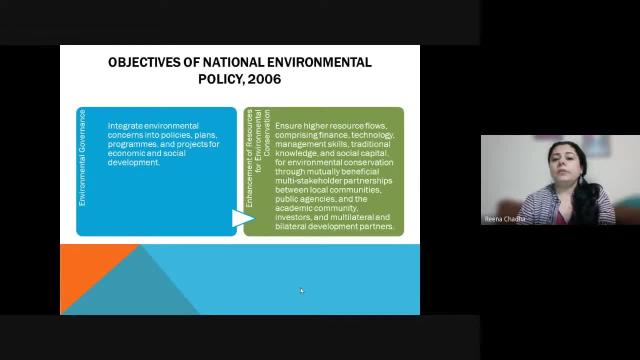 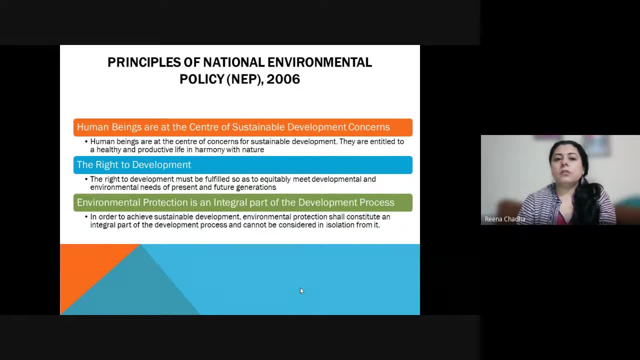 then, uh, environmental governance, enhancement of resources, of environmental conservation. that should be our priority. so what were the principles? principles of National Environment policy: after discussing National Environment policies objectives, we will discuss what are the principles. so there were three main principles that all human beings are the center of sustainable development concerns. so if we think 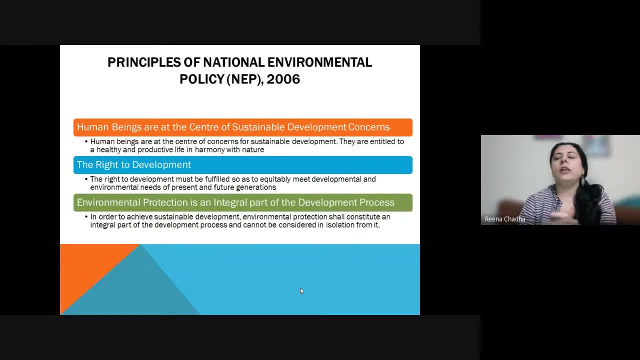 that this SDG goal is something which is just theoretical and which is just defined to uh to reflect that International bodies are taking care of environment. no, that is not the case. so if we, if you have uh listened to the last lecture, where we have studied about the international environment governance, in that also, first sustainable development goal was: 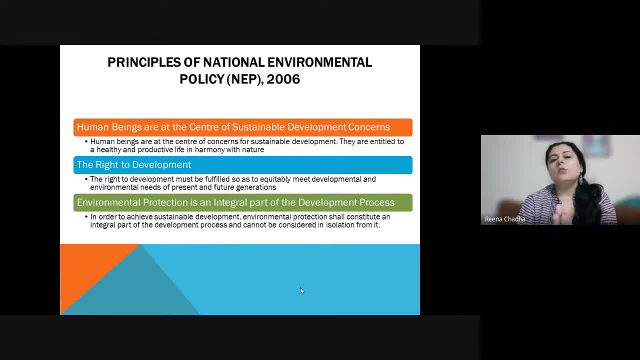 that human beings are at the center. okay, so our National Environment policy again reflected the International principles of environmental governance. so in that case, all human beings should be treated equally, and we should be, and we should ensure that we are, at the center of concern for sustainable development and we should be able to, uh, play our 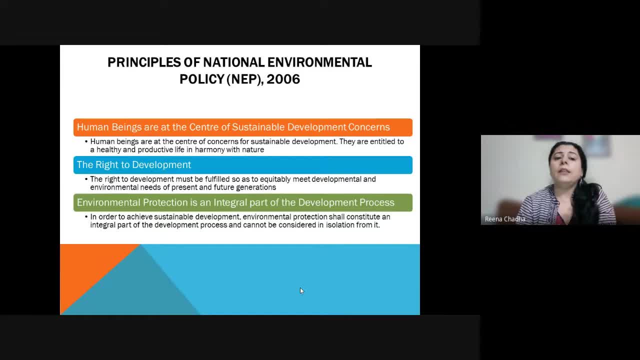 pivotal role in in providing healthy and productive life to everyone, including the natural resources, including our environment, including our flora and fauna. okay, again, we have a right to develop development. we definitely need development. we cannot stop development. so we require to meet uh equal developmental and environmental needs for present and future generations. okay, because future. 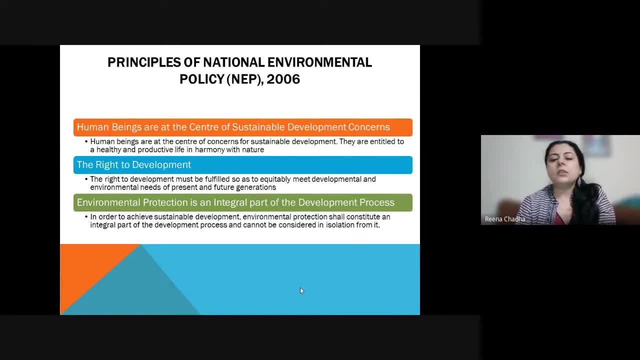 generation also have this right to development, not just the present, and generation has this right to development. everyone should have the right to development, and then environment protection should be part of any kind of developmental activity. so any kind of new project that comes into picture in present times, it has to take care of environment protection. it has to get 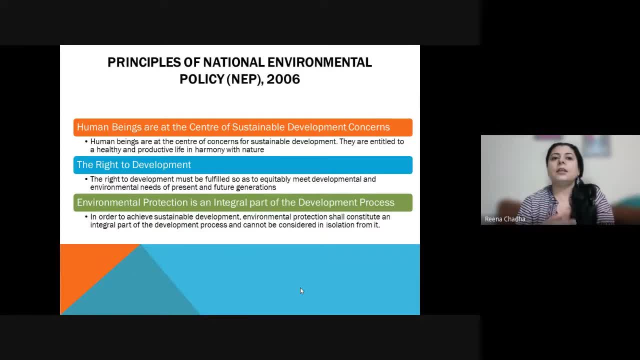 environment clearance if its area is of certain extent. if it is uh requiring consent for uh establishment, consent for operation. if it is utilizing water resources, it has to take consent under water act, otherwise under air act. if it is generating hazardous waste, it has to get authorized under hazardous based apps and rules so that 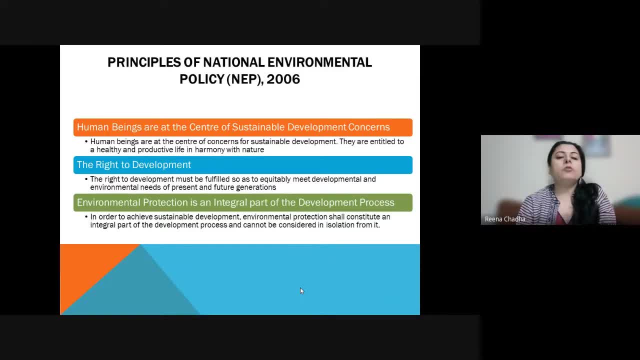 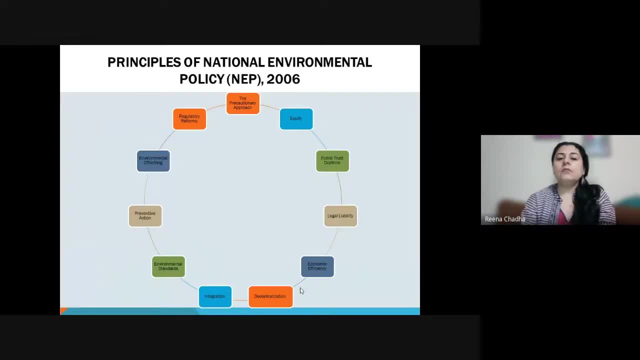 has to be a part of development process. that's why, if those kinds of requirements are there for any kind of development activity in our country. so these were the principles and uh, there are around uh 11 principles. okay, so if you see uh from regulatory reforms, precautionary approach, equity, 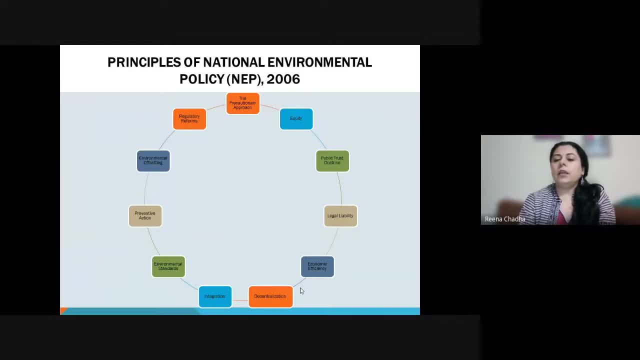 public trust doctrine, legal liability, economic efficiency. so if you have been attending my last two, three lectures, you might must have understood the concept of every uh term which which is written on this slide, aside from the regulatory reforms, the precautionary approach, the equity, the public trust doctrine, because all the international environment 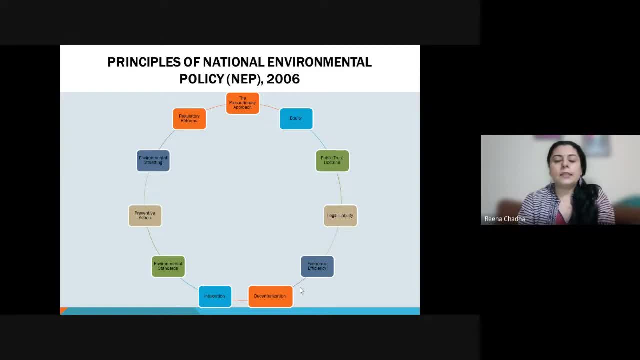 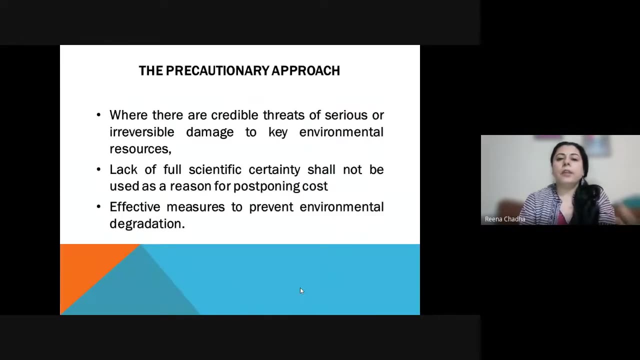 governance related uh guidelines and aims and objectives. they were also framed around these principles so accordingly, in our national government, policy is also framed around each of these principles, but we'll still discuss each of them. so, starting with precautionary approach, precautionary approach basically advocates that there are some credible threats and of serious and irreversible damage, damage which cannot be. 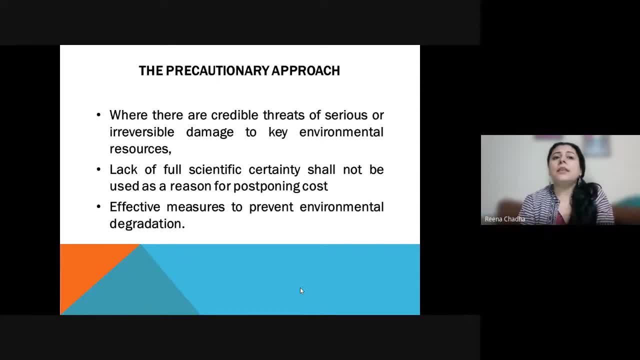 reversed back damage which once caused will stay there forever. so that kind of damage, if it's there, we have to take precautionary approach because before causing that kind of damage, damage okay. before disposing of any nuclear waste, before disposing of any chemical spill, before disposing of any effluent which is high in its recalcitrant compound concentration which is high. 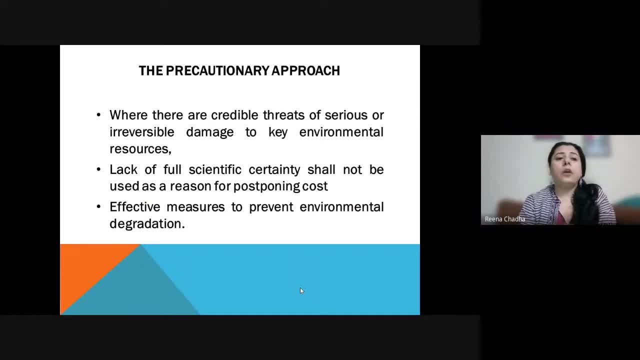 in heavy metals into underground water, into soil dumps. so that kind of irreversible damage should always be avoided and there should be precautionary approach. then lack of full scientific certainty on until and unless you are well aware what kind of impact it will cause to the environment, you should not do that kind of activity. if you are lagging any kind of 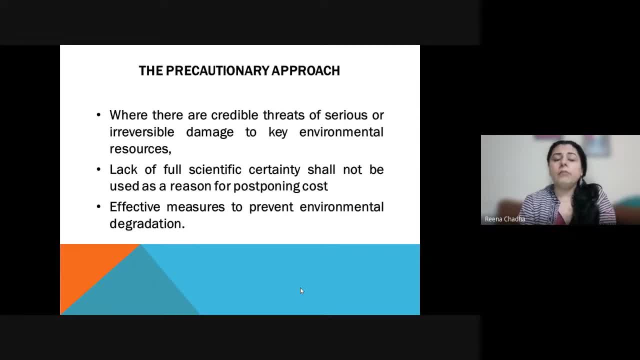 scientific data or information about an activity which you are going to implement. you should always use a reason for postponing: the cost. okay, so the cost of tackling that environmental burden? okay. so you have to have proper scientific knowledge, you have to have proper scientific guidance before implementing any such activity. 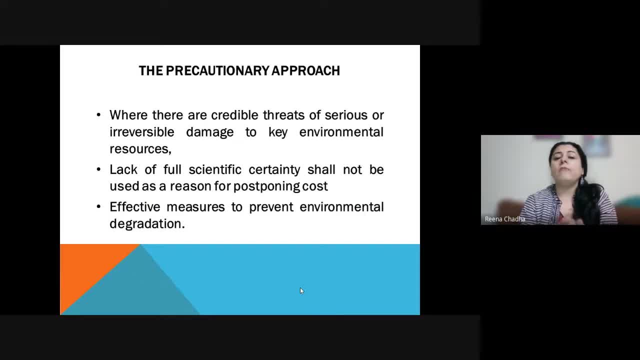 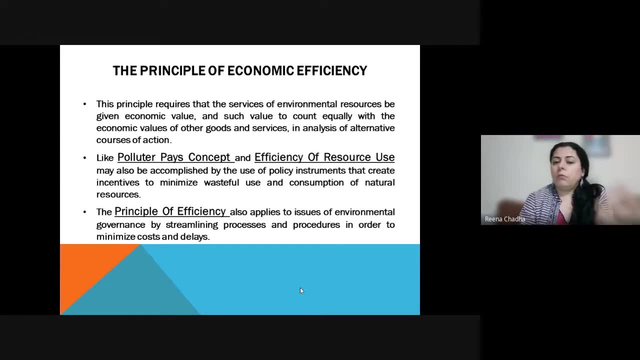 which can cause irreversible damage, and then you have to have proper measures to prevent that environment degradation. second principle: economic efficiency. economic efficiency as you, as the name suggests, you have to utilize Minimum of resources to get maximum of benefits. efficiency is when you are utilizing whatever you your system is designed for to 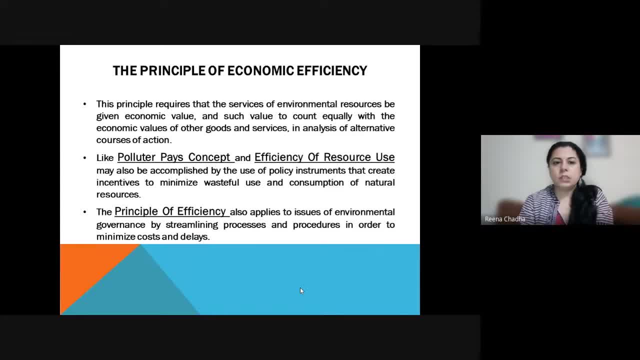 maximum extent. okay, so that is your efficiency. so again, if the principle requires that the services of environmental resources be given economic value, because most of the times our environmental resources are observed to be available free of cost, okay, we all have this idea that we do not have to pay for the air quality, but when we go to a doctor we pay for our medical bills. we do get. 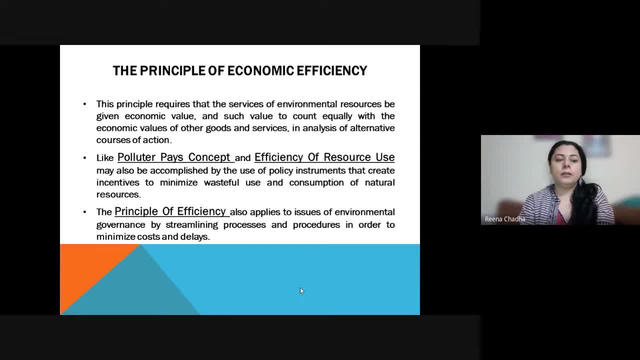 the value of air, air quality, when we buy an inhaler, when we buy an nebulizer, when we buy an air filter or air cleaner in our houses nowadays. earlier we used to hear the name of air conditioner only okay, but now there is a, an air cleaning equipment also that is available in the 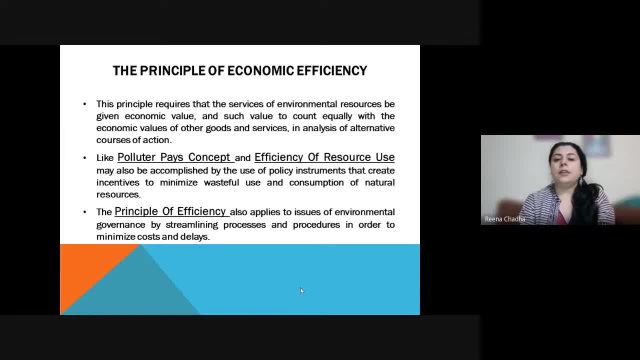 market. so when we go to buy that equipment we understand if we, if we would have been given a good air quality, we should not have been investing in this kind of equipment. so unless there is a value attached to any environmental resource, we cannot advocate protection of that environmental resource. so we have to have polluter-based concept. we have. we 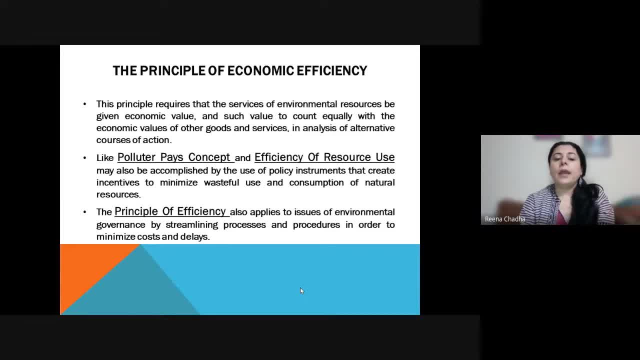 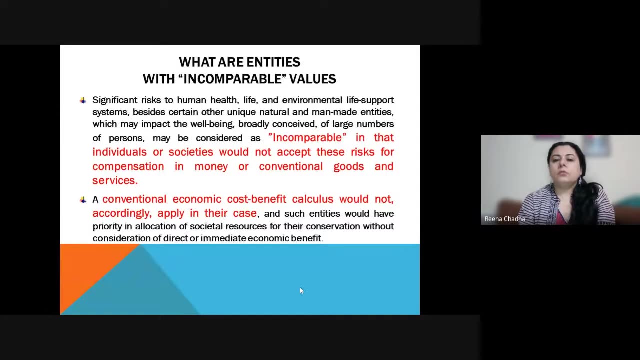 need to ensure efficiency of resource use, and the principle of efficiency should be streamlined in all our processes and procedures so that we can minimize the cost and delays. okay, so again, what are the entities with incomparable values? so, some, there are some values. there are some entities which have a value which cannot be calculated. 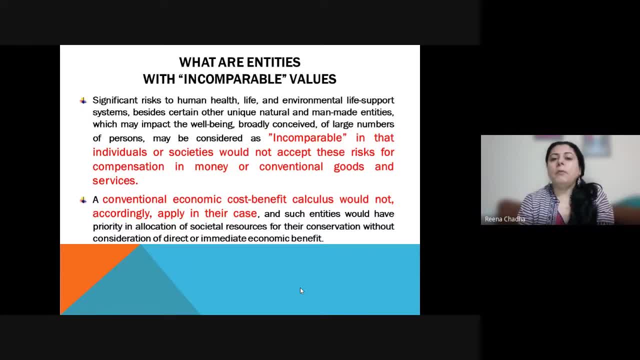 okay. for example, your well-being, the impact of good having good aesthetic scenery, impact of having good aesthetic natural environment, that is incomparable okay. so if you say that, okay, we are having few beautiful tourism sites, we have ecotourism sites, plant sites, you calculate value? 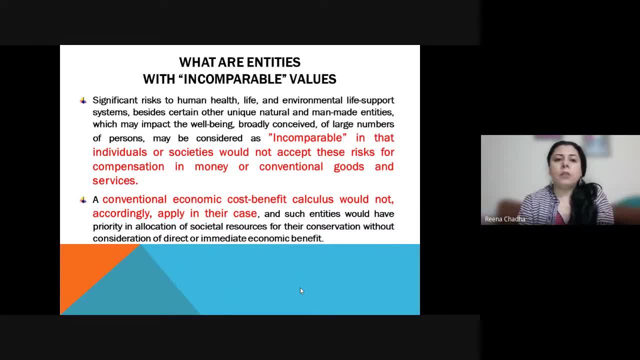 of those resources, though monetarily i'll be able to calculate the value, but otherwise, if you consider their total value in their total lifetime, their value is incomparable. okay, so you should not accept any kind of risk for compensation in money or conventional boards and services to risk those kind of resources which 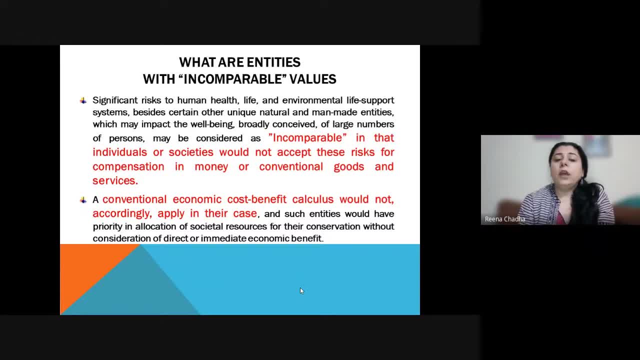 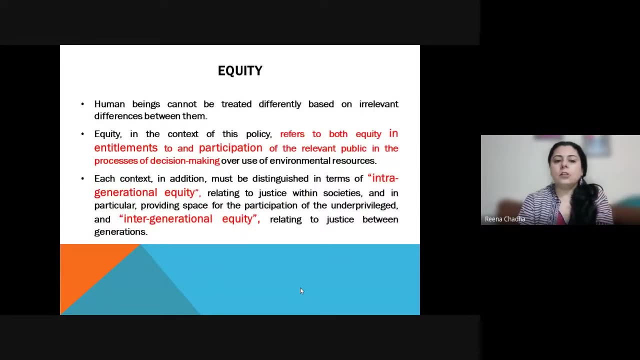 has, which have incomparable values. and then we have to have a conventional economic cost benefit calculation before we have priority and in allocation of societal resources. okay, again, equity equity. we have been, uh, studying again and again intra-generational equity, intergenerational equity. equity is basically equal distribution of resources. okay. 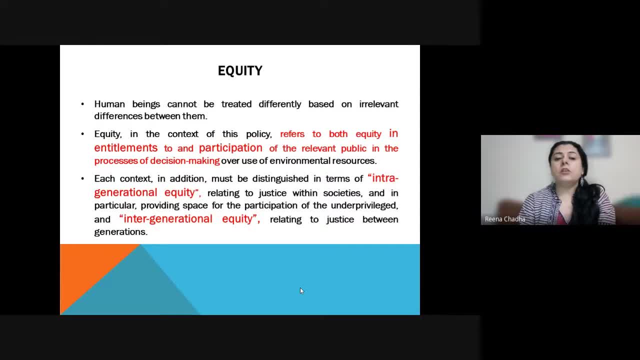 so again, this equity uh plays a very special role in given, giving entitlements to, participation in giving and right to participate in the process of decision making. for example, in all kind of projects which we are implementing today through international funding, there is a process of consultation, public consultation, even in eia process, apart from construction projects, in every 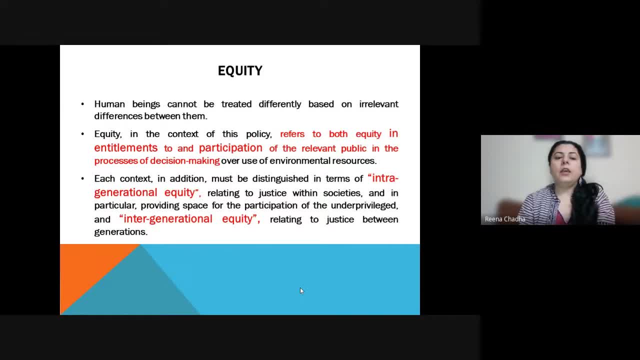 project there is a provision of public consultation, okay, public hearing. so in those processes we are, we are giving, we are being given power to participate in the decision making process, but most of the times we don't even care to look at the notice which comes in a newspaper for any public hearing, and many of you might not be even. 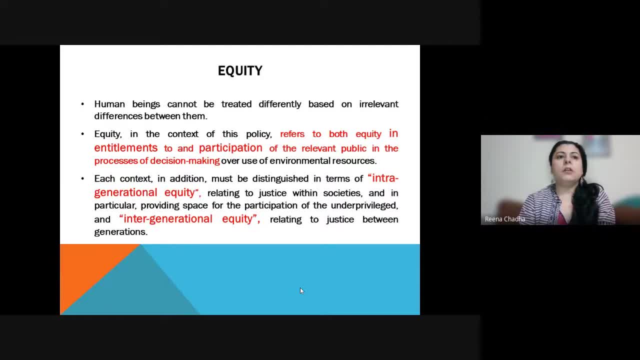 aware that such kind of notice comes in newspapers, in our reputed dailies, so that people are made aware about any new project, activity which is coming in their vicinity? okay, so if we are aware that such decision making processes are existing and we can be a party? 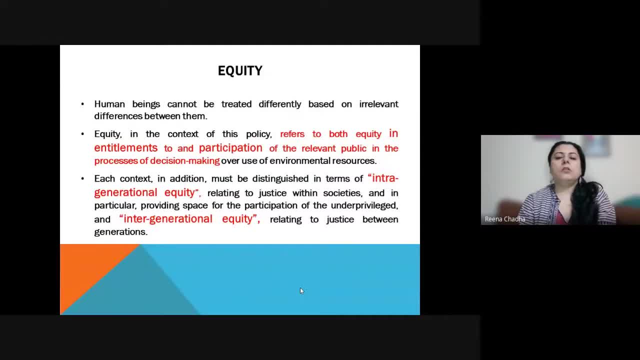 to that we can play a role in uh, those decision making processes, then definitely we'll do that. but if you are lacking awareness and if you are thinking that equity means just distribution of resources, quantity- no, that is not the case. it is again a right to take part in every kind of project activity- then legal liability, so every uh. 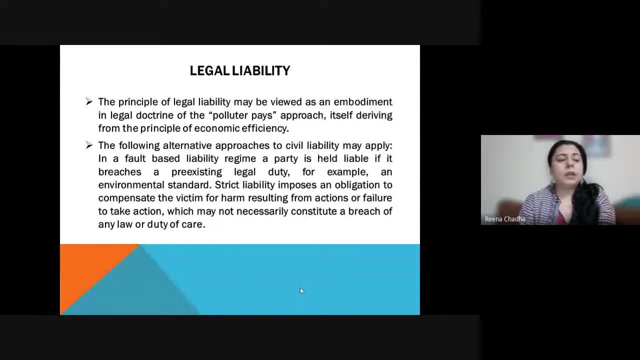 polluter should have a legal liability so that there is no other episode like bhopal- guest tragedy, okay, or there is no fire breaking out in any uh cinema hall, like that happened in delhi years back. so all those uh issue chemical leakages or chemical spills from industry even. 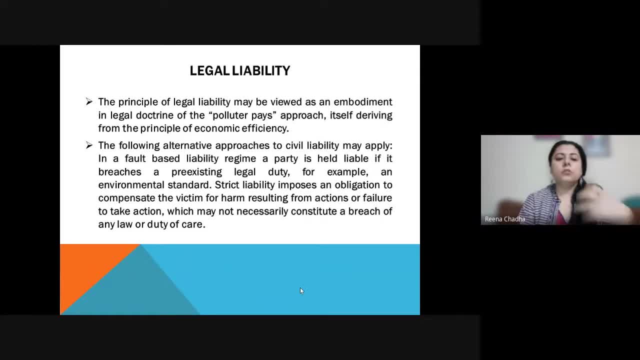 spills and marie uh oceans. uh, due to ships and due to uh, uh like spillage due to ships and due to uh, uh like spillage. uh, due to uh, uh like spillage. uh, due to uh, uh like spillage- spillages from the tankers- oil transporting tankers- in oceans. so all those episodes can be. 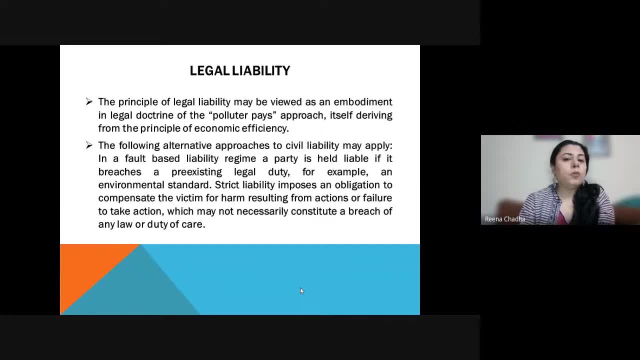 avoided. if everybody knows that, okay, i'm going to pay for this pollution if, if it is caused by me and that paying for pollution uh will be much higher cost, rather than going for a process which gives me minimum risk, which involves minimum risk and minimum damage to the environment. 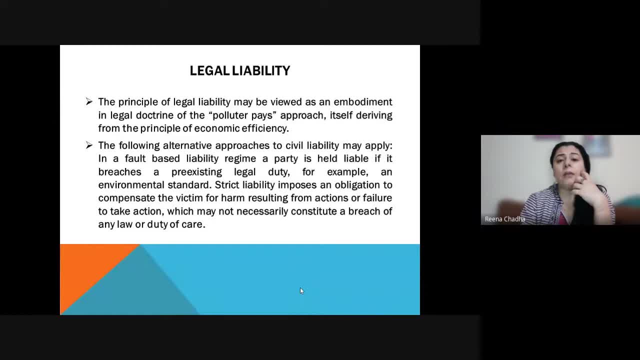 so unless and until we place a legal liability on any or on every polluter, we cannot have this control of environment pollution okay, so there has to be a strict liability that is imposed on obligation to compensate the victim. so if, in present scenario, if even if an educational 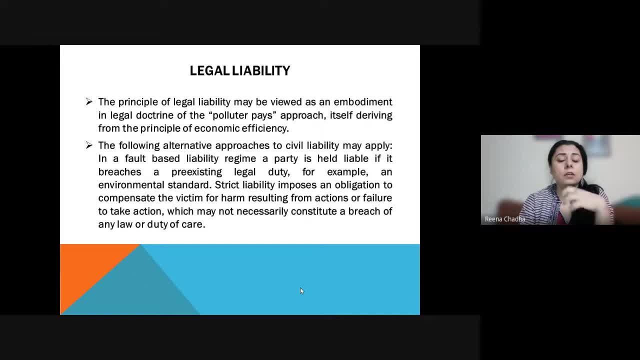 institute does not take environmental clearance, its vc can be directly taken to court or it can be directly imprisoned. okay, he or she can be directly imprisoned. in any other case of any kind of legal laxity there is no such provision. so in environmental guide, rules and regulation there is provision of strict action. okay, so again, public trust doctrine. 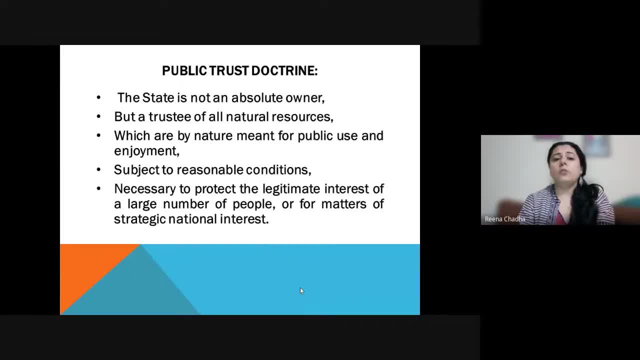 it advocates that state should be an absolute owner, but all the but a trustee, of all natural resources. it is an owner to take care of the natural resources which are meant to be used by public and it is meant for enjoyment of the masses. okay, so we have an legitimate interest in a large number of people's. 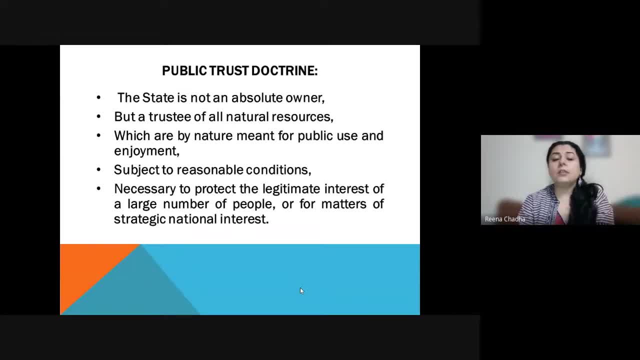 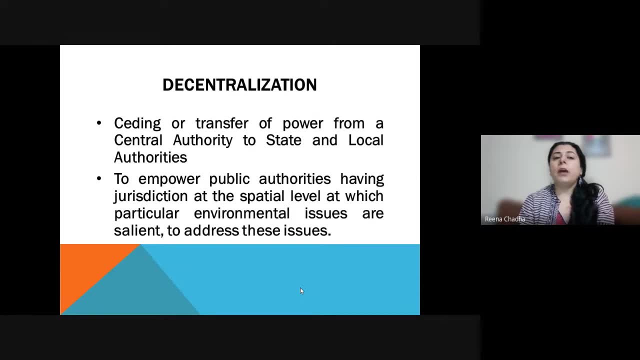 protection. okay, as a matter of national, strategic, national interest. again, decentralization is also a principle, because we want to have power at local level as well. okay, not just at the central level or at the state level. even at the local level, we want to have power at the local level. 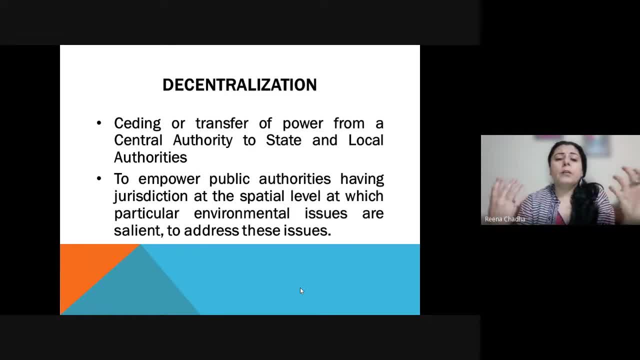 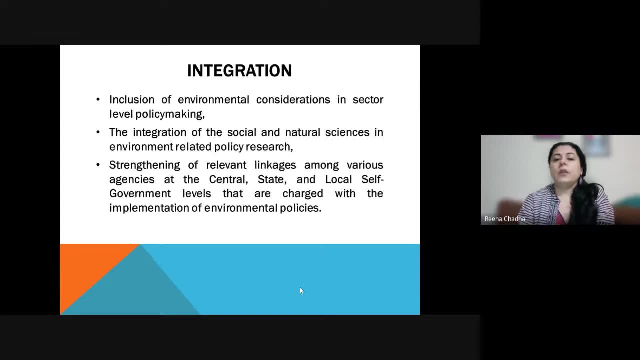 even at the local level. we want to have power at the local level. we want to have power at the local level. even the local public authorities. they should have a power to get themselves involved in protection of environment, to address their local issues. okay, because at local level governance they are better. 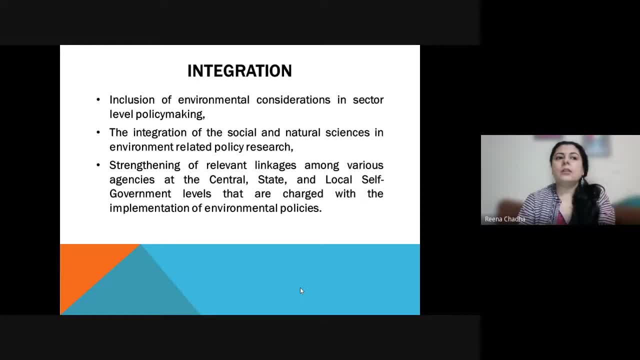 equipped and they are better uh understanding. they have a better idea and data related with the problems- environmental challenges- that are occurring in their area. so that's why decentralization also plays a big role and in the local level, we want to have power at the central level. 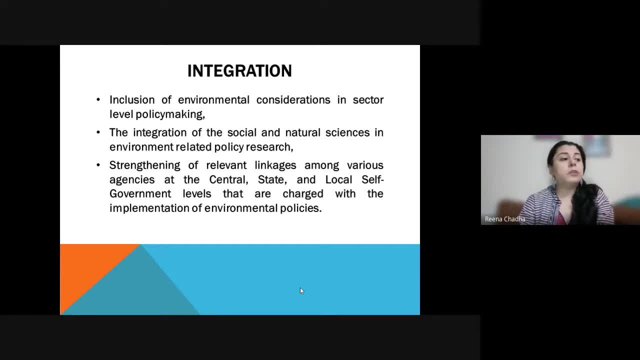 in covid 19 phase also, you must have observed that first uh ban and first uh lockdown was introduced at central level, but after that that central level uh like idea or the central level governance was transferred to the state and local level. so any local uh body who found that okay, my 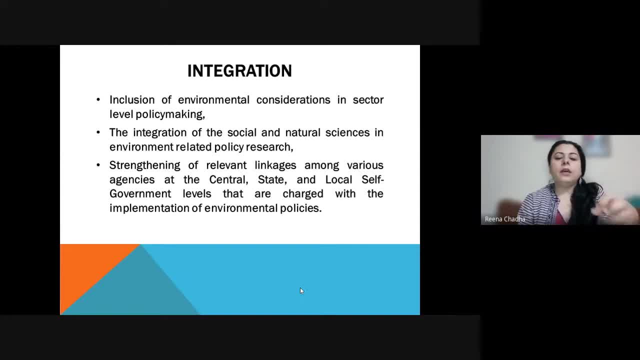 area is having more number of cases. they can implicate a local level lockdown or uh restriction on movement of people in that area, rather than expecting central central guidances or central lockdown. okay, so that was the idea which was also utilized during uh decentralization of processes in coven 19 control, again in integration, is again an inclusion of environmental considerations. 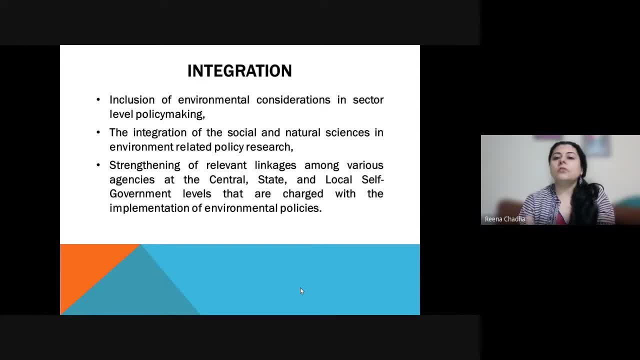 in sector level policy making, so how social and natural Sciences should be integrated together, how society needs to understand more about natural resources and how that can be introduced in policy. research so it did. this involved integration at various levels. now, for example, even Department of Science and Technology tells every research body, every institution who takes up funding for some kind 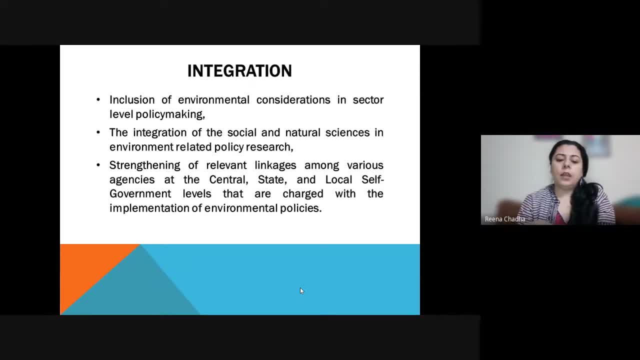 of R&D activity to uh and integrate with them, to associate with them any business organization or any uh organization which is having advancement in development of prototypes. okay, so that after an R&D is being funded by DST and after it is being implemented by a research body, by IIT, by IMS. 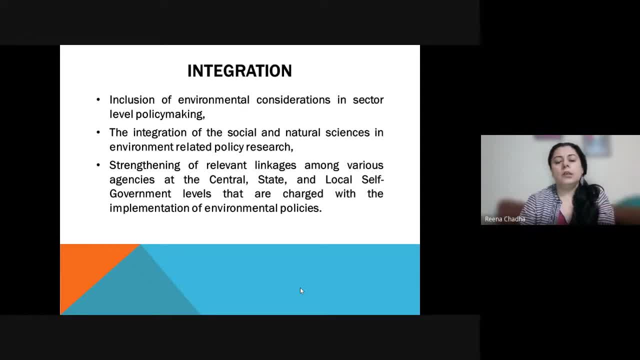 that research just does not lies in their libraries. that research is again utilized to develop some kind of prototypes. it is used to develop some kind of employment. it is used for development of enhancement of environment protection. okay, so that is the idea, while when we go for linkages in 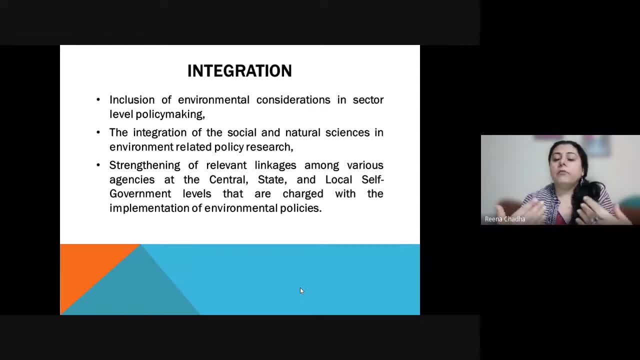 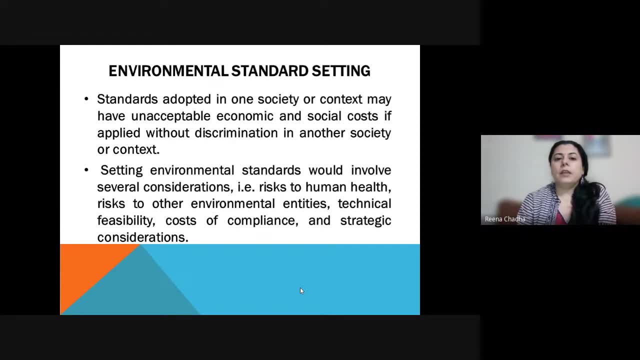 various departments in various agencies and we reflect those. uh. strengthening of relevant linkages in our environmental policies. then environment standard setting, because if there is no standard, okay, this you can just. this is the highest level of pollution that you can create. after this you have to be. 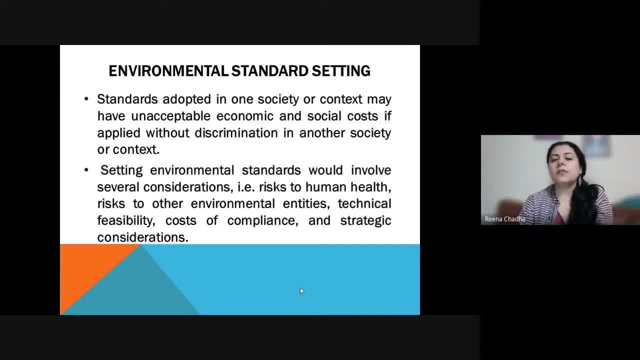 set under pollution based principle. unless such kind of standards are not set, every polluter will keep on polluting the environment because that is not set through any standard and again, that is immeasurable. okay, so we have to have Technologies. we have uh research protocols, we have SOP standard. 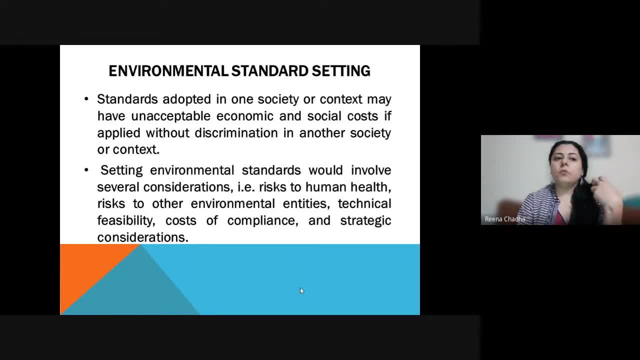 operation protocols where we can uh measure that pollution. we can measure those standards, we can measure those particular parameters which have been identified by central pollution control board and pbcb. so all those things we will be discussing in the next lecture related with EIA also. so in this uh we have to have environmental standards that cause risk to human health. technical: 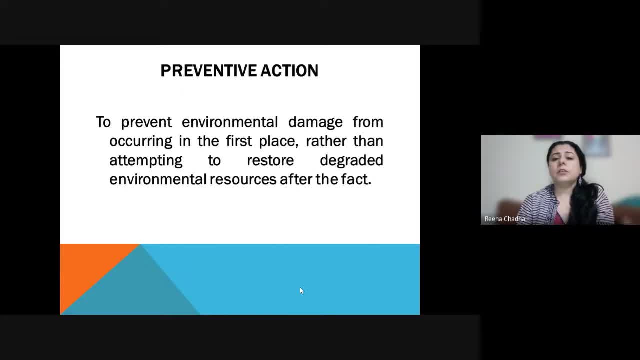 feasibility, cost of compliance strategy considerations- okay, okay, okay. next principle is preventive action, where you have to prevent any kind of environmental damage to come up. policy decision matters at your level is also associated with realization that an environmental hazard monster is 네 any kind of environmental damage to come up in first place itself. okay then, environmental 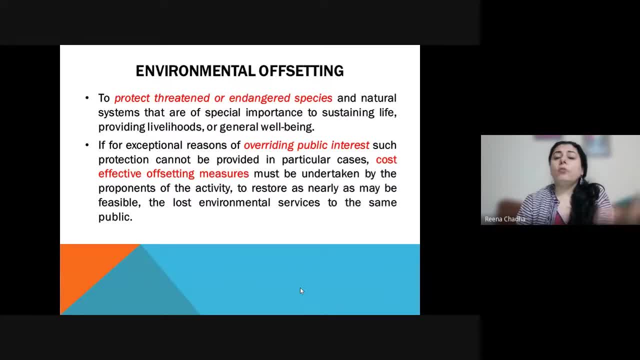 offsetting. offsetting means to protect created or endangered species that are of special importance. okay, so if, for example, exceptional reasons of overriding public interest, such protection cannot be provided in particular cases, so cost effective offsetting measures should be taken up to restore that activity and the lost environmental services to the same public. for example, if some kind of 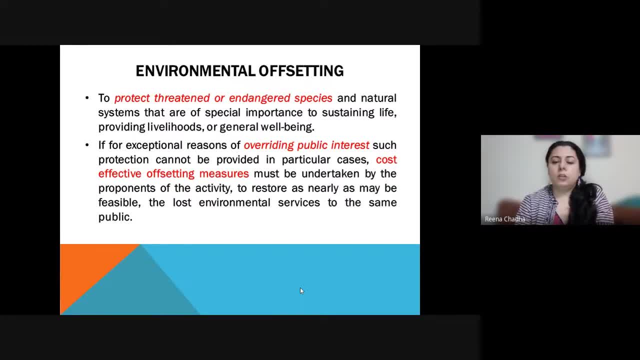 damage has happened which is not under control of any activity or developmental project, for example, due to earthquake only for, even if it is a natural disaster, some kind of damage has happened in some protected biodiversity area. so we should have take a approach to offset that environmental damage and to protect more of the threatened and endangered species. okay, so we can. 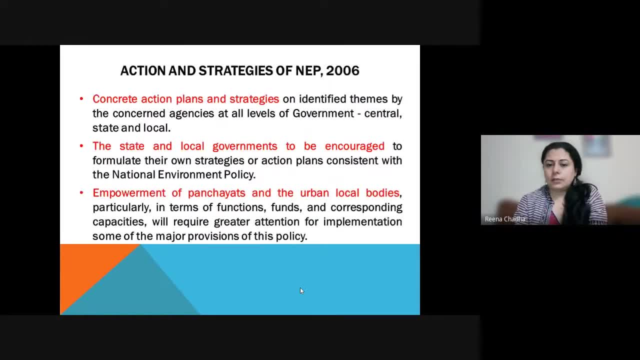 override public interest. in those exceptional cases, then actions and strategies were also planned for national environment policy. we have many action plans and strategies and if you search for specific sectoral action plans and strategies you will find that even for the panchayat and local bodies there has been specific uh invoice centers. environment information centers are there there. 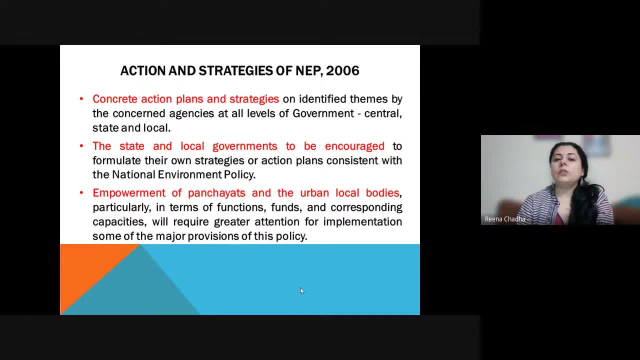 are state and local governments are also introduced in these strategies and action plans. so at every level there have been specific action plans and specific strategies so that no part of the community is left out while implementing these and national environmental policies. then regulatory reforms were introduced, as we discussed in the last 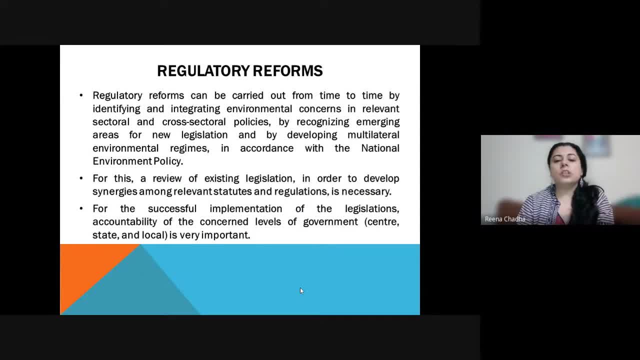 lecture where we have a comprehensive discussion on air act, water act, solid waste act, hazardous waste act. so all those acts and amendments were discussed in our last lecture. so they are, they all form a part of regulatory reforms. okay, so from time to time reform means you have formed something. 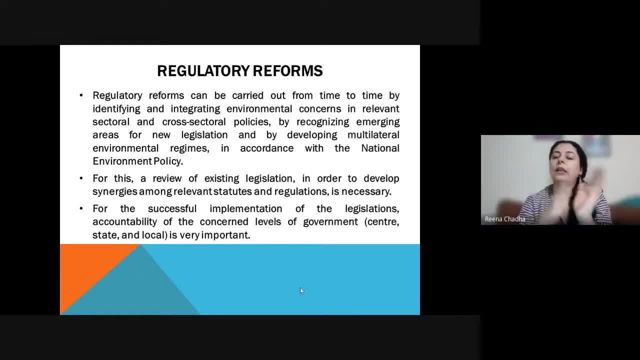 and again you are making some amendment that is reformed. okay, so we have made some regulatory provisions and from time to time we identify: okay, some kind of concern is there, some kind of gap has been left out, there is some cross sectoral policy that needs to be revised. that we can. we have some new technology. 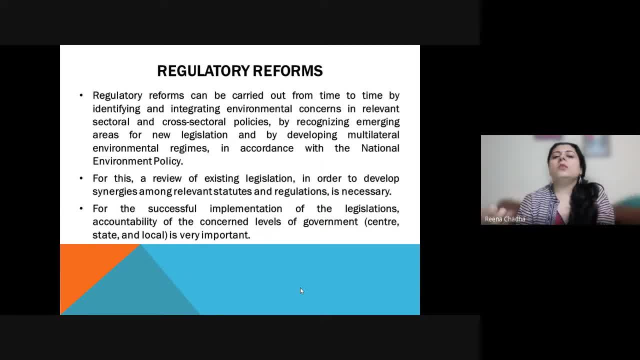 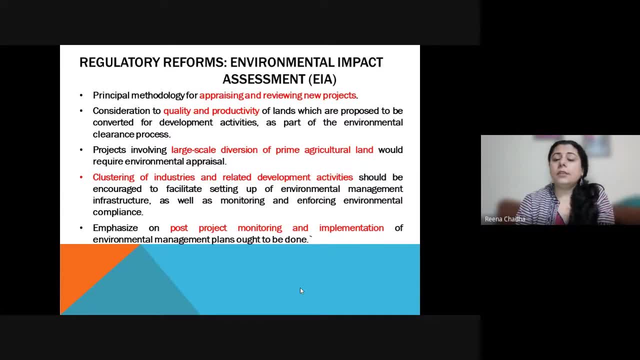 and strategy which can be introduced, so all those measures can be introduced through new reforms and new amendments. then, uh, this latest regulatory reform came up in environmental impact assessment, principal methodology, how new projects are going to be appraised, how they are going to be reviewed, and we are going to discuss this in very detailed manner, uh, in the next lecture. how large-scale. 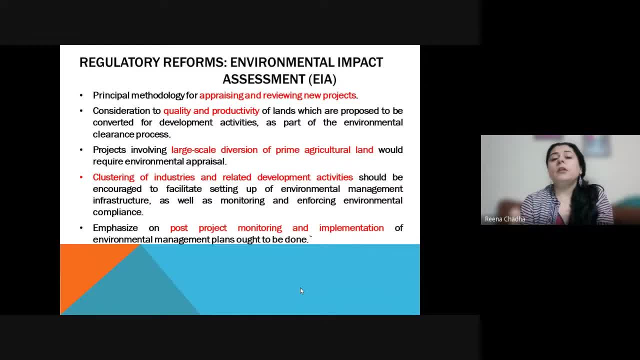 diversion of prime agricultural land requires environment appraisal before going for that diversion, before taking up any change of land, you'll see a use, which I was talking about then- how cluster of Industries related with some specific activities they can, they should be clubbed together in industrial zone, in special economic zones, in IT sector Zone or for some, uh like we. 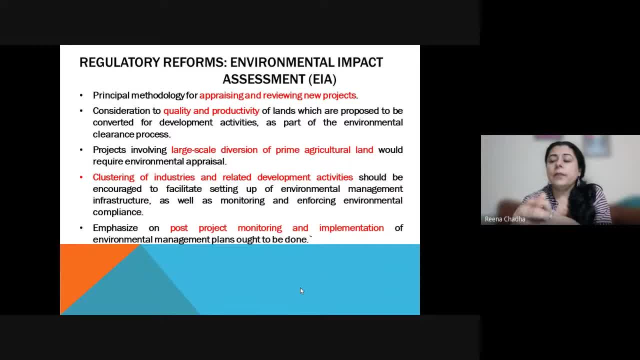 established and a large area development project for cycle industry in Ludhiana. so those kind of clustering of Industries and related development activities helps you to tackle certain uh wastewater issues that is related to that industry through employing a central facility for pollution control for air pollution, for hazardous space. because although Industries are having same 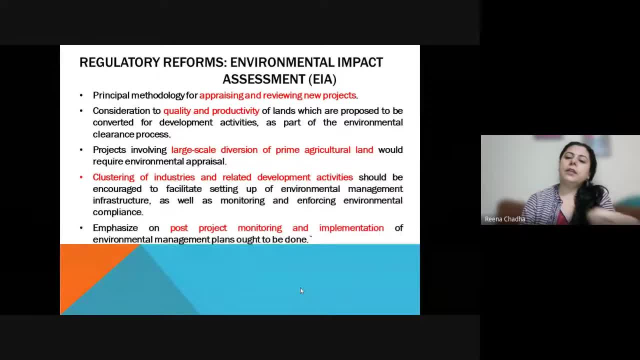 characteristics of their inputs and outputs and they will be generating same kind of wastewater, same kind of air pollution related parameters. so it is better to have Industries clusters, because we are. we will be able to manage the issues, the environmental problems which will be caused by those Industries collectively and it will be beneficial for all the small scale and 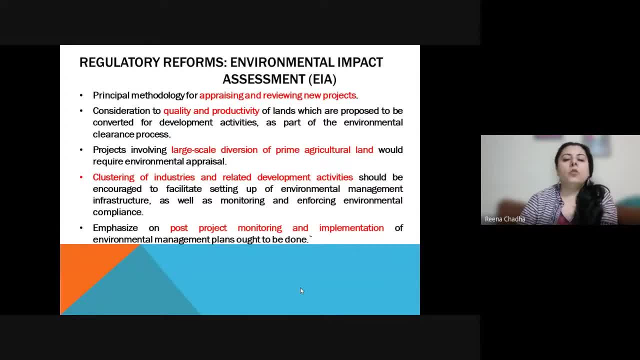 medium scale industry who do not have enough resources to have their independent uh an affluent treatment plant or air pollution control devices. so if they are connected together, if their pollution streams can be connected together and treated together, it will be beneficial to establish that kind of centralized development activity uh area. okay, so again, post project. 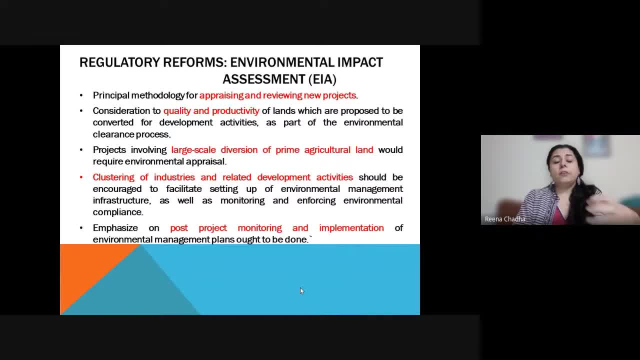 monitoring, for example, in mining, at present, if you, if you go for clearance of mining projects, you have to have a post uh mining plan. okay, that is called reclamation plan. so what kind of reclamation activities which will be done after you leave that mining area? because 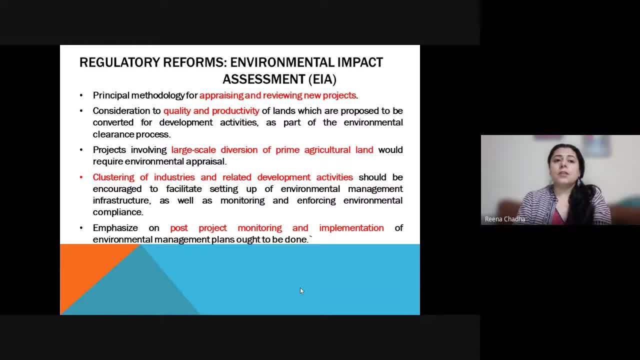 if you leave a mining area after extraction of minor or major minerals it is. it looks like an abundant wasteland. okay, but if you have a reclamation plan you do a forestation activity, like in Delhi also. you must have seen earlier that open landfill site at the Delhi border was. 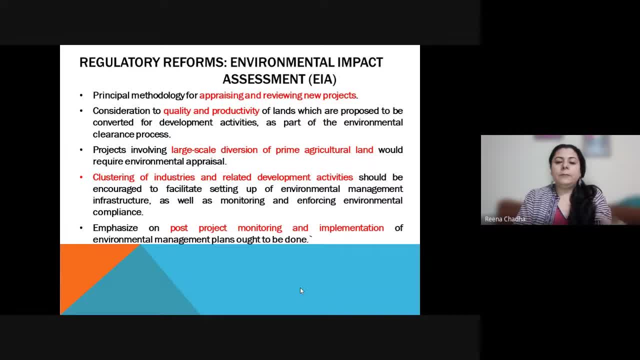 left as it is, but when NGT intervened it has been planted. now it has been covered with different kind of plant species and it looks like a green area and it is now being redeveloped- okay, due to reclamation activities- the kind of damage that was being caused to that land- as an open landfill site. 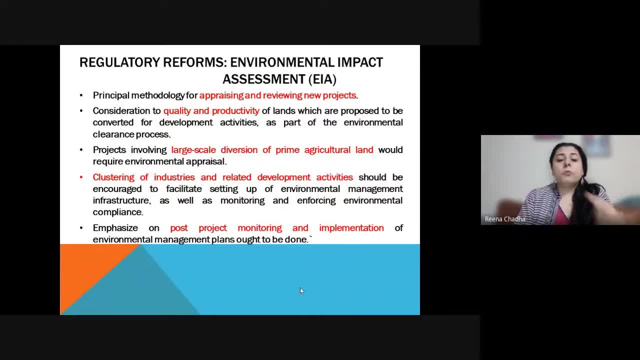 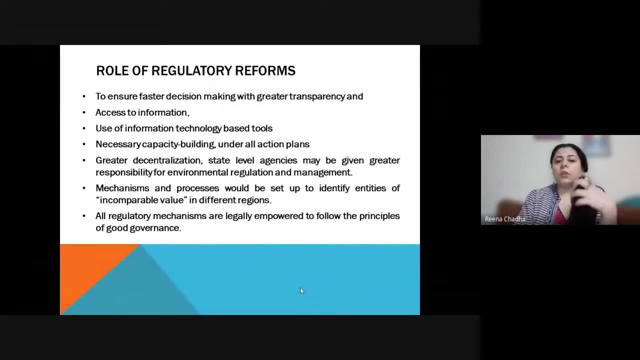 is now recovering. okay. so those post project monitoring activities and implementation of environment management plan was again monitored and again regularized through these regulatory reforms. so what are, what is the role of regulatory reforms? through the examples which I have given to you, you can understand that it helps you in. if some kind of regulatory reform is there, you you might. 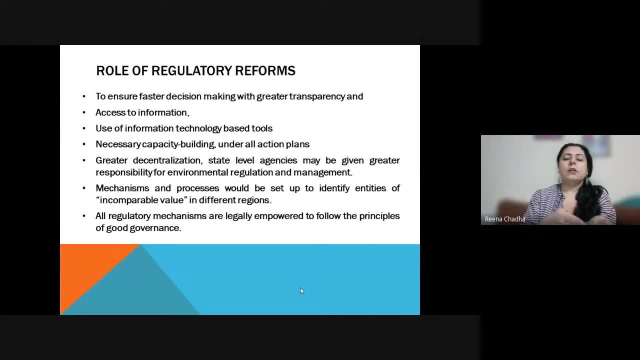 not take any time. okay, what should be done if this problem has occurred because you will just go? okay, that can be done. it can be penalized. this person who is caused pollution has to pay this much for this kind of pollution. so it will help you in a faster decision making and a greater 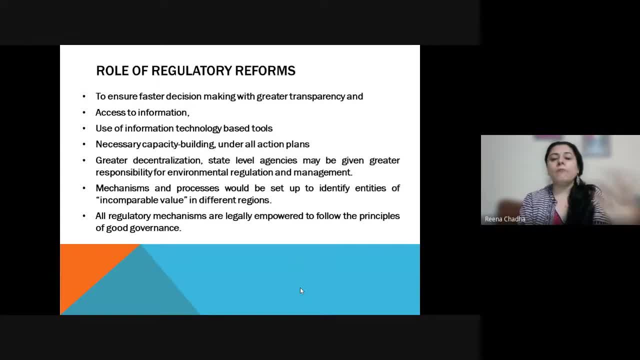 transparency. so that rule will be again, ever same for everyone: no one polluter may not pay more. one polluter may not pay less. if it is, if it has caused a damage which has which can be measured through standard it get, which is there in the regulatory reforms you, you also need to consider industry, etc. for the rest, yeah, that has to be taken into account during theavoiratch' operation pozyntz, the very first deficit-seeking main infrastructure group, the very second deficit sector that does not result in the climbed rates those تeding sector crisis in this budget. 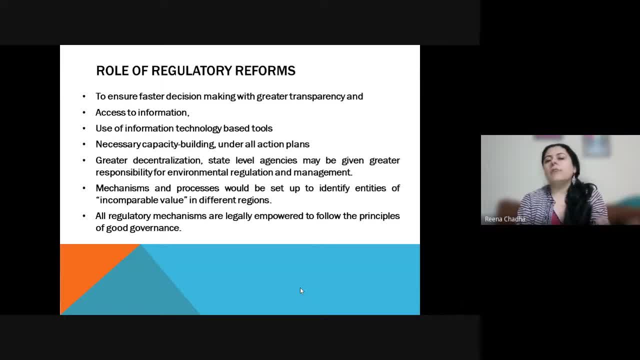 peer and the people handling the activity. So if for whether everybody else, they are planning for the carbon dé sentex diagram to have a faster decision making, then you have access to information, you have use of information technology based tools, you have capacity building. you have all the data related with air quality is. 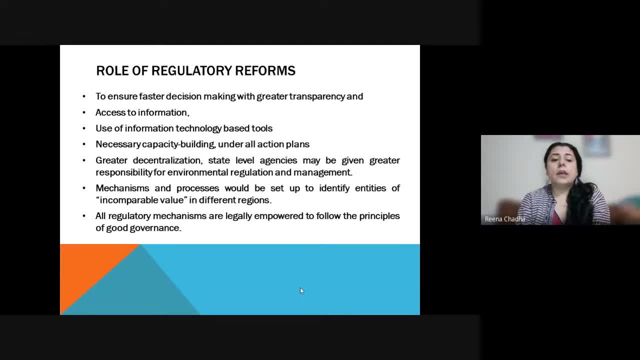 now available on center pollution control- both sides, okay, your ground action, groundwater uh monitoring plans and groundwater level uh plans. they are also available on central groundwater body websites. so all those gis tools and all those- even in google you have uh tools wherein you can see how that land used to look 10 years back and what kind of devastation has been caused after an. 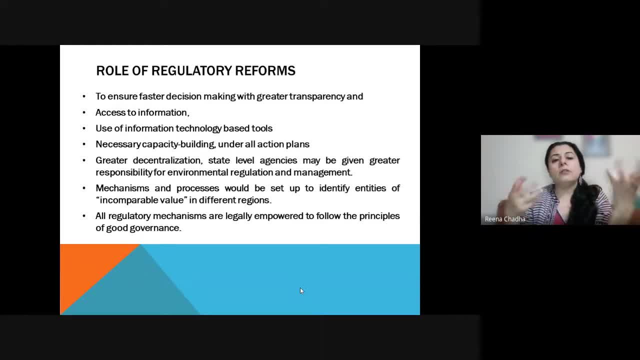 industry has been set up, or even a project which is uh implemented for the conservation of that area, how that a project has changed the overall scenario, overall spatial uh view of that area. even google earth can help you in giving such kind of tools, so it helps you in greater decentralization in 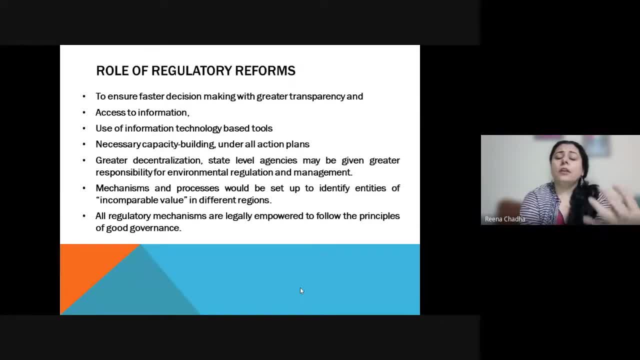 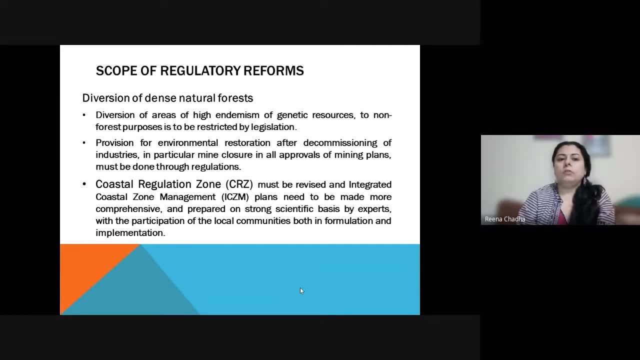 greater regulatory mechanisms. it makes you, it gives you power to follow the principles of good governance. so what is the scope? so these uh regulatory reforms? they vary from diversion of dense natural forest there to coastal regulation zone. even for coastal regulation zone we will be studying a more in. 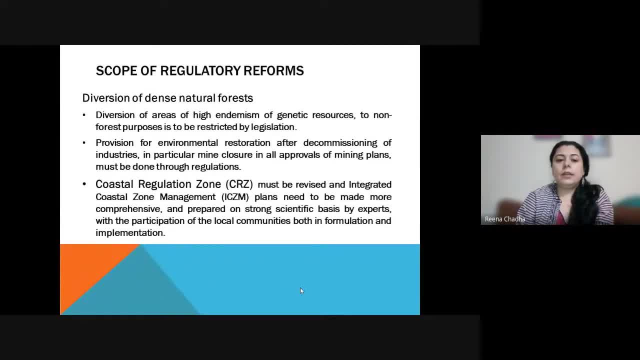 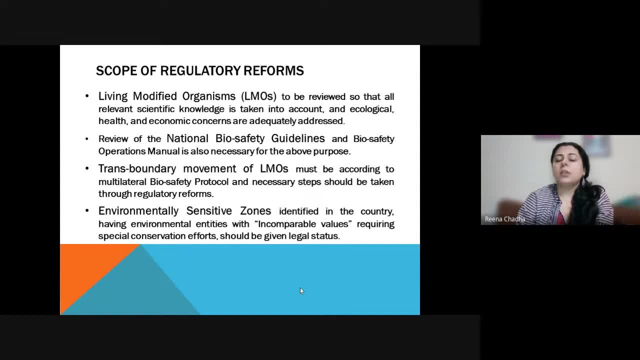 detail, along with eia in the next lecture again, living modified organisms which can be reviewed so that relevant scientific knowledge is taken into account and how national biosafety guidelines can be implemented so that no live uh biomaterial is taken uh away from our country or is taken. 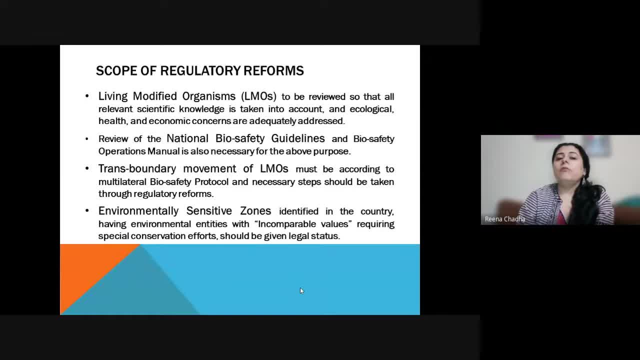 outside our country. okay then, trans boundary movement of, uh, living modified organisms, some systems which are working on the environment, uh, in nature. so, so everybody can not just introduce a kind of some virus or some biologically damaging variety of some plant or animal or algae or fungi species in our water bodies. so all those regulations are there. trans boundary moment of. 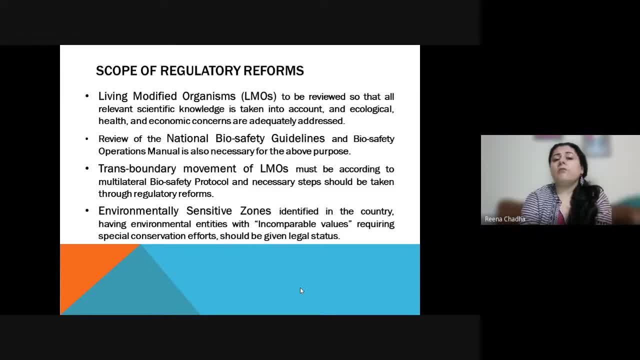 living modified organisms gives you a multilateral biosafety protocol. okay then, environmentally sensitive zones have been identified, where which are having incomparable values. where values are, They are having irreplaceable values which cannot be replaced by any kind of costing or evaluation method. So they have been given legal status of environmentally sensitive zones. 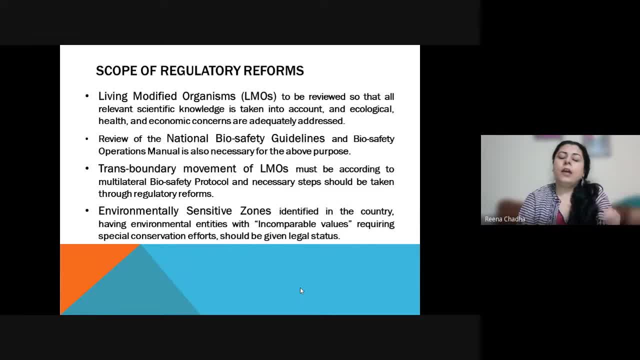 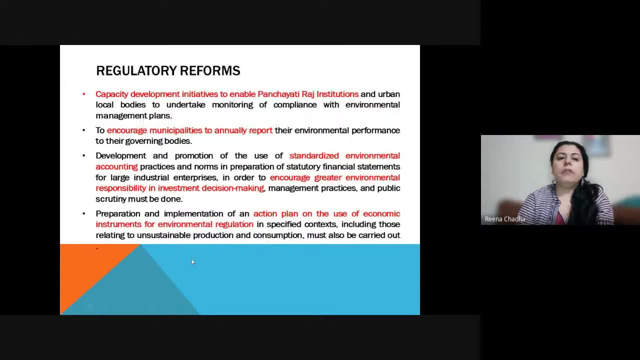 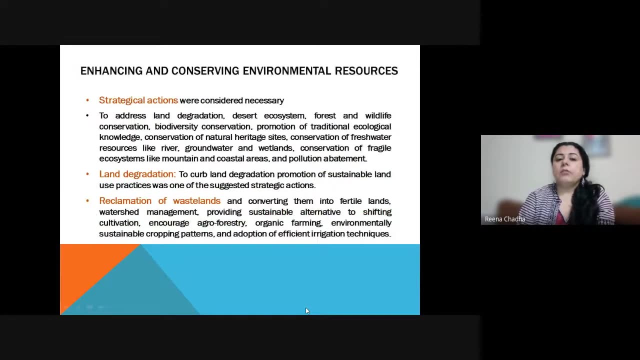 So that and sensitive zones are again considered while going for any environment impact assessment notification related clearance. So then we have regulatory reforms for capacity development initiatives and enhancing and conserving of environmental resources related with land degradation, reclamation of wastelands, forest and wildlife. 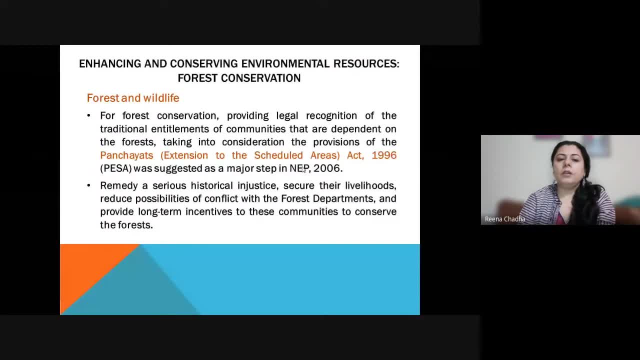 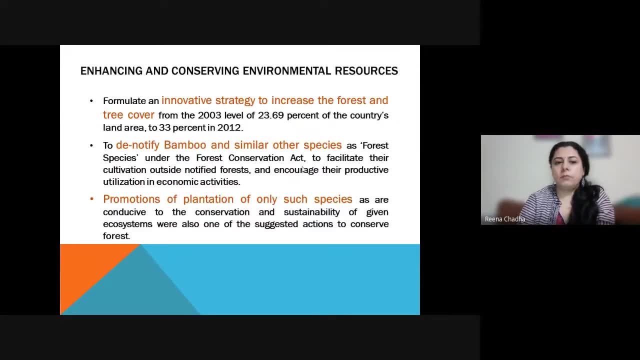 Then forest, and forest and wildlife, and there has to be a remedy to any serious historical injustice that is being caused in conflict with forest departments And there has to be an innovative strategy to increase the forest and tree cover from the level which existed in 2003.. 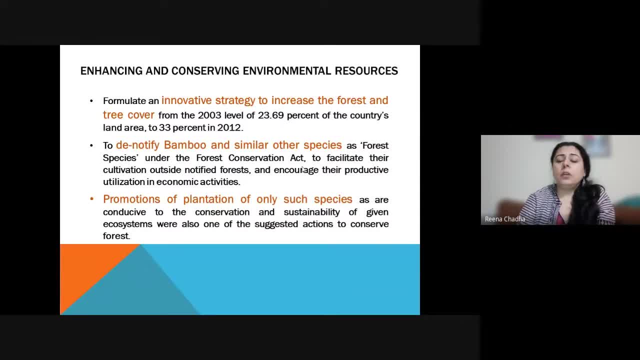 That was just 23.69%. So it was policy reformulation which was introduced that we should go for At least 33% percent by 2012. okay, so again, uh, now we have to conserve that level. uh, if, if we do, if we cannot. 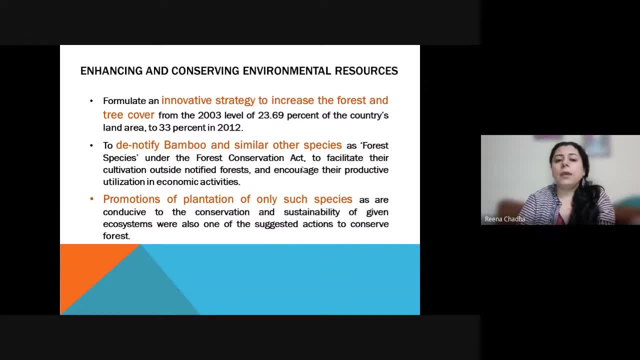 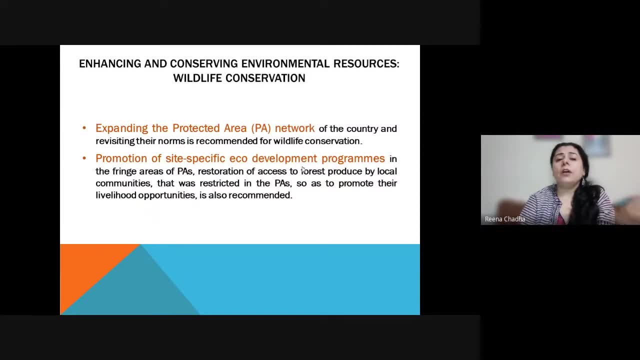 enhance that level. we have to conserve that level. then bamboo and similar other species were denotified under forest conservation act and we have to also expand the protected area network and site-specific eco-development programs were introduced, for example wetland programs were introduced, baseline programs were introduced and specific programs for mangroves and other. 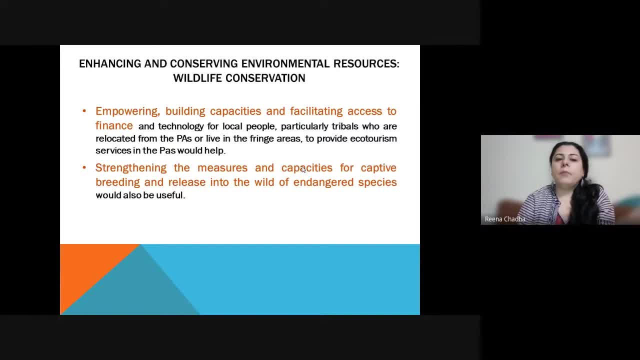 uh, biosensitive zones were introduced then empowering building capacities and facilitating access to finance that, for example, local people and tribals- they were not having enough capacities to have access to finance. and then strengthening and their capacities and measures for captive breathing, breeding okay and release into the wild of endangered species, for example. 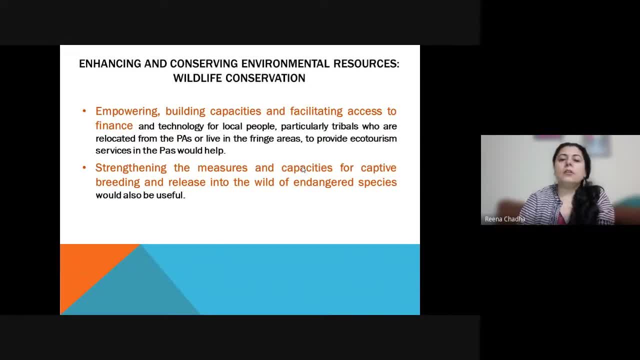 recently our prime minister modi has uh released uh tiger species in our country. so uh on on his birthday. so those kind of activities can be done only if we have national policy which goes in hand with those kind of action plans at ground. okay, so again, explicit attention has to be given on 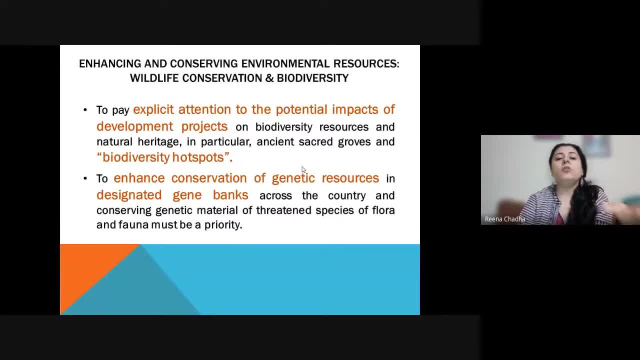 potential impacts on development project. for example, whenever you are doing any kind of activities, you have to see within 500 meter radius which biodiversity hot spots are coming, which green areas are coming, if there is any protected zone which is coming. if it is coming, you have to go to the relevant department. if it is a protected forest or reserve forest, then you have 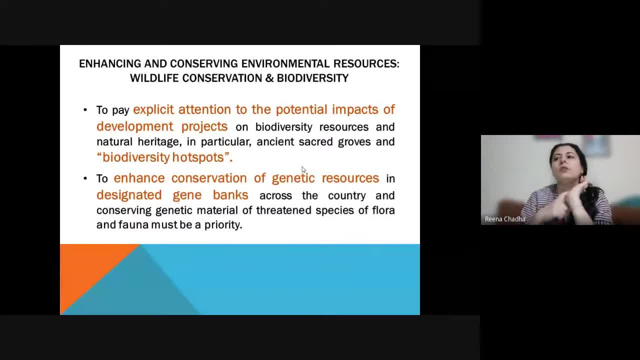 to go to the forest department. you have to take their permission, you have to submit the drawings which shows the distance in google image and then they will actually calculate how much distance is there and, as per the notification of that reserved forest, how much distance is allowed for that construction activity. 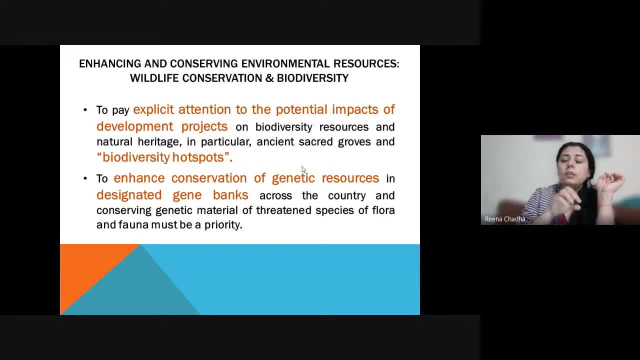 to actually take place or not. and if it is not allowed within the distance that has been given in the notification for that reserved forest, it will not be allowed. so we have uh clients who, which we regularly suggest, okay now, if there is a distance from this lake, sukna lake, or this uh. 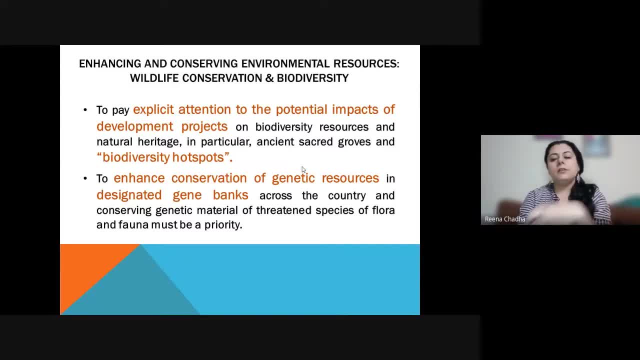 protected forest, then you have to go to this department submit the type of the information that they need to clear the document. okay, so they say that your improvement work is right. okay, then you will take this kind of document and you will take it will take around 15. 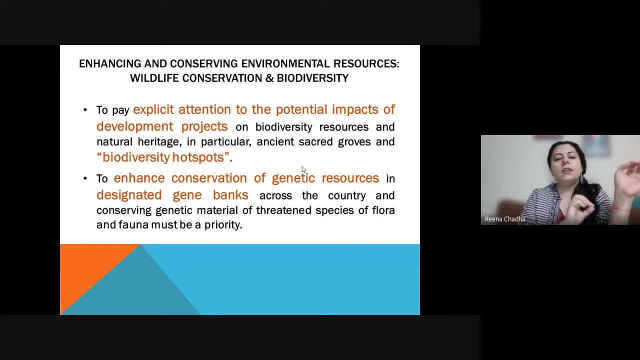 to 20 days, then only you will be given clearance. you will be given actual distance, which is uh for with- from the location of your project to the protected site, and whether it is safe or unsafe. so if it is written safe, then only they can go for environment clearance. okay, so before environment. 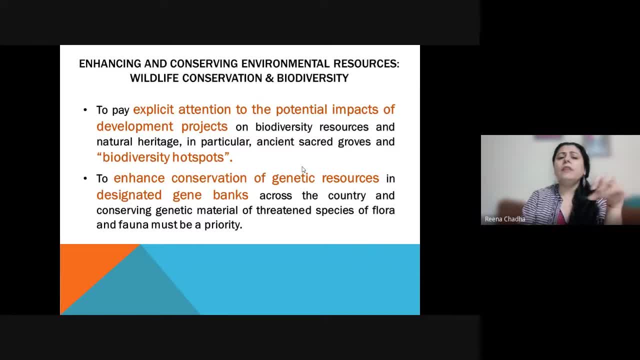 protected forests. okay then, this is again in line with our national policies and national principles under wildlife conservation and biodiversity. okay, then, you have to enhance conservation of genetic resources. you have to conserve genetic material of threatened species of flora and fauna in designated gene banks. so those gene banks have already been identified. 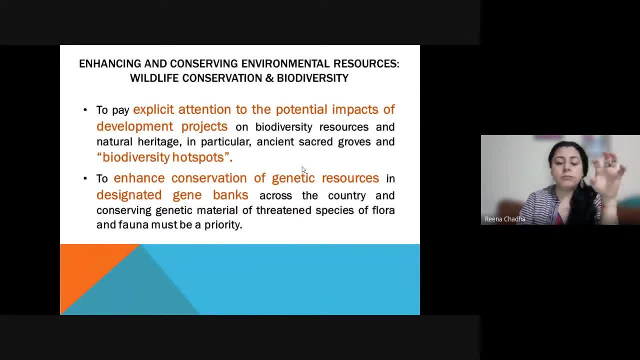 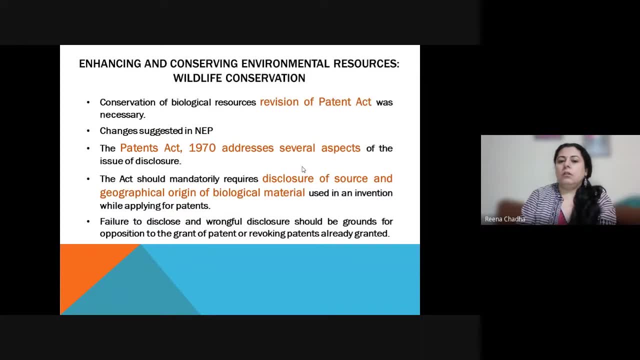 they have already been established for different kind of species in different parts of our country. so then you have division of patent act, how these uh, disclosure of source and geographical origin of biological material- can be controlled. this is again laid down in elaborately manner in under wildlife conservation act. 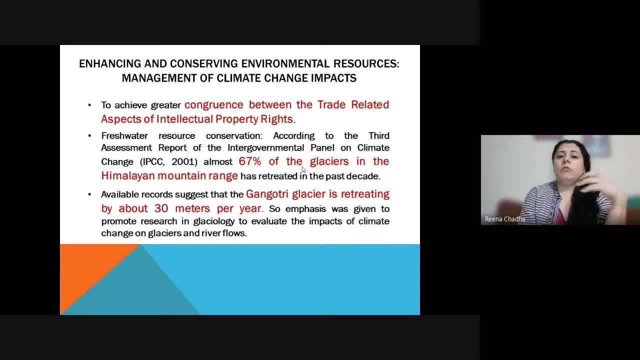 so, when we see about how we can conserve environmental resources, there is a very pertinent issue of climate change impact- so all our activities, they should be in congruence with intellectual property rights. also, then we have to take care of the himalayan mountain range in terms of the, in terms of the threats, which is, which are there for. 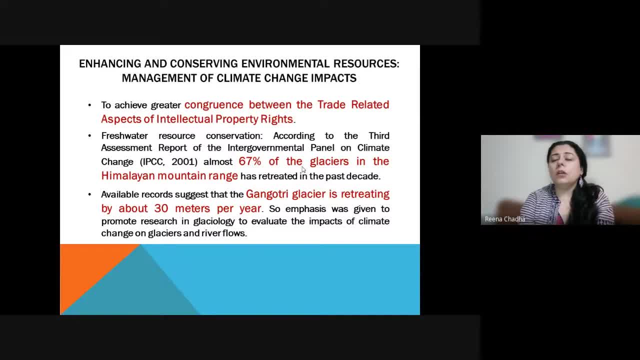 through climatic change effects. so, according to the third assessment report of the ipcc intergovernmental panel on climate change, almost 67 percent of the glaciers in the himalayan mountain range they have retreated in the past 10 years. okay, so that past decade has shown. 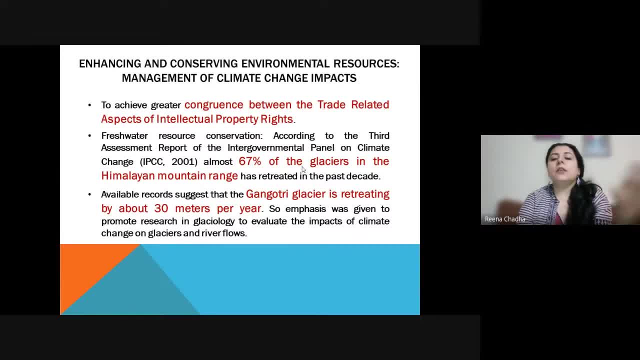 actual data on how this these glaciers have are being are retreating themselves. so for that purpose, we have to ensure the protection of these areas and how we can reduce the impact that is being caused due to climate change, even if we cannot reduce, how to mitigate those impacts. 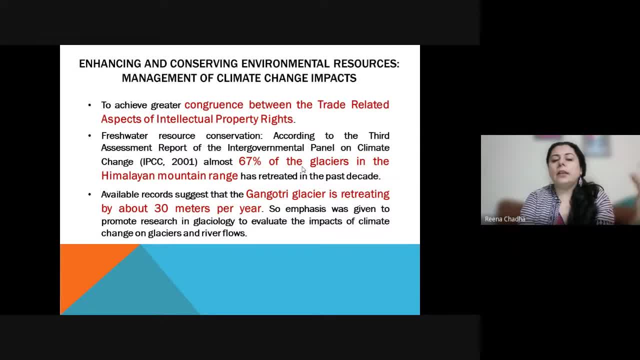 so, for example, gangotri glacier is again retreating by 30 meters per year. so we are doing a lot of research activities. lot of r&d projects are going on to promote research in glaciology and to evaluate the impacts of climate change on glaciers and river flows, so that we can 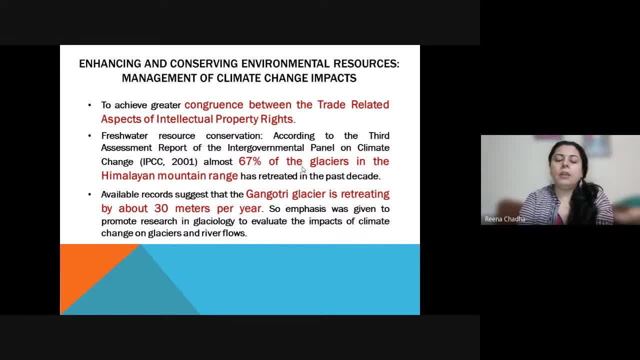 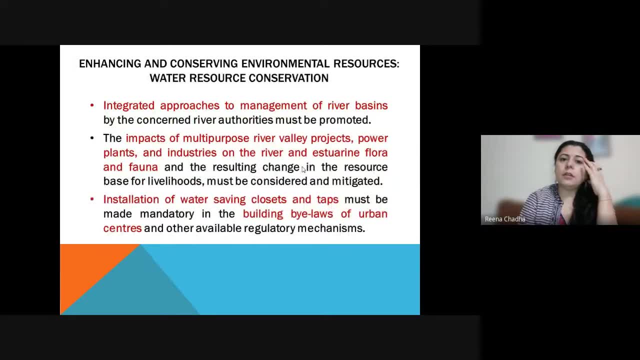 in uh, we can evolve strategies and tools to control those impacts. okay, so again in and have a look at the next slide, please. okay, so one of the things that we have been doing is we have been expanding the conservation of environmental resources. water resources is a prime resource and we have many uh integrated approaches. 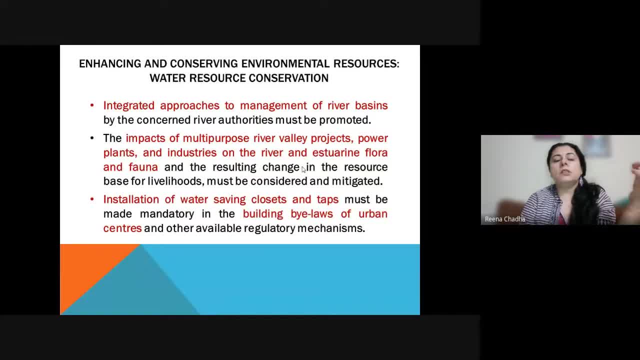 for management of river basins. like wetland management is a part of river basin strategy. then we have a multi-purpose river valley: dams, power plants, industries, estuarine, flora and fauna, watershed management projects, then installation of water saving closets and taps in houses. so in in building bylaws also. if you see our national building bylaws, again those bylaws have been. 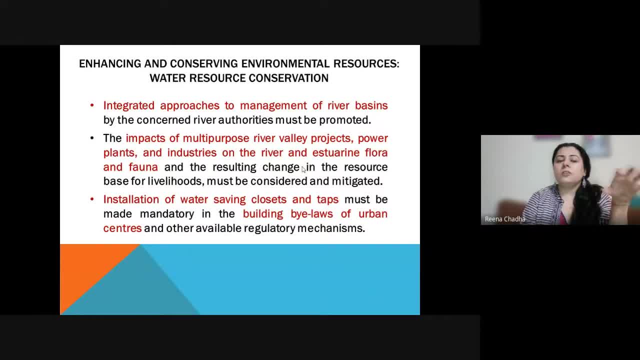 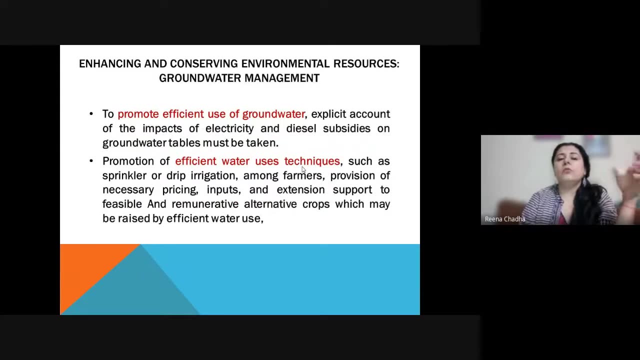 revised and they have specific measures to control water: industry level, at local level, at household level, at agricultural level. so there are many strategies uh to for efficient water use, for promoting efficient use of groundwater as well. for example, nowadays if you want to take permission for groundwater extraction, you have to submit impact assessment report for groundwater. 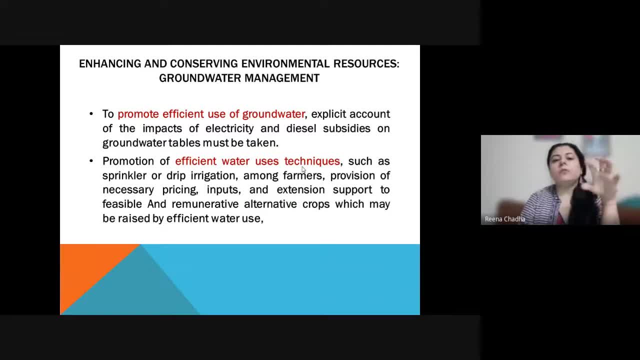 exploitation. okay, so earlier that kind of report was not submitted, so i have already uh made 50 such reports, maybe more than that. so, for in that report you have to give the complete area around your project site, you have to identify what are the threats which can. 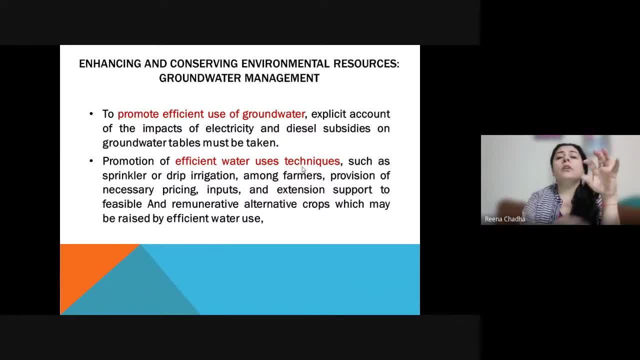 be there from to the groundwater levels? what are the different kind of industries which are existing around your project area? what can be the cumulative impact of water groundwater extraction in that area? then? what are you? what are uh different strategies and industries using specifically in-house for controlling of their uh water extraction, for whether they have installed? 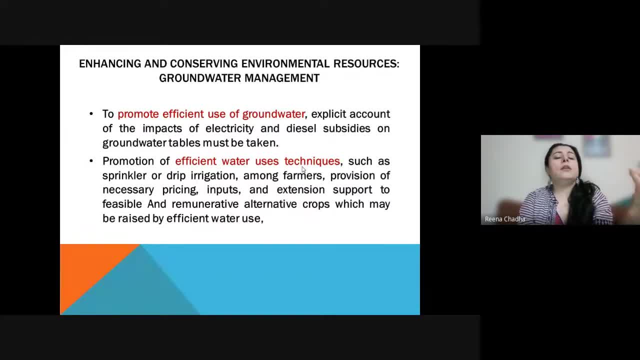 groundwater meters, whether they are doing recycling of groundwater, whether they are minimizing the use of groundwater then whether they are adopting rainwater harvesting techniques, whether they have adopted any ponds. and if they are utilizing more groundwater- then they can recharge or restore- then they have to levy some taxes, they have to pay some cess for groundwater as well. 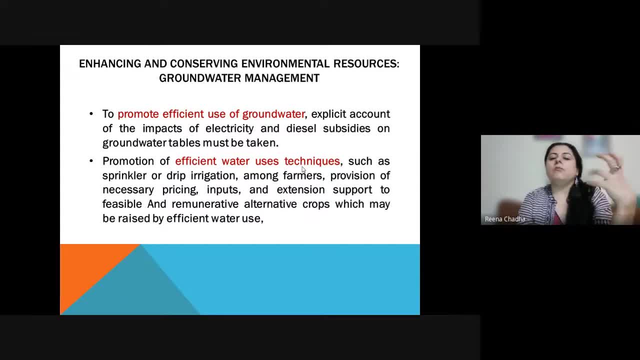 okay again, they are promoting efficient water use techniques like drip irrigation among farmers and they are derivative and alternative crops which are being introduced in himachal also, japan international corporation agency. they have introduced a project for alternative crops for giving knowledge up to the local masses and 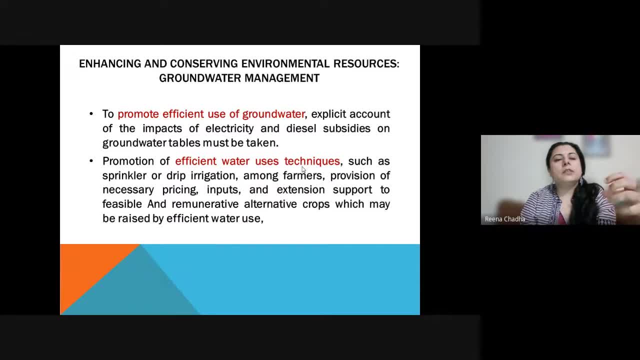 communities who are involved in agricultural business and who are doing agriculture from ages through cash cropping. okay, so they have been. they have been introduced to other which are utilizing less of water and giving more uh nutrition and giving more economic benefit to them. okay, so many uh exotic vegetables like capsicum and broccoli and mushrooms, which were 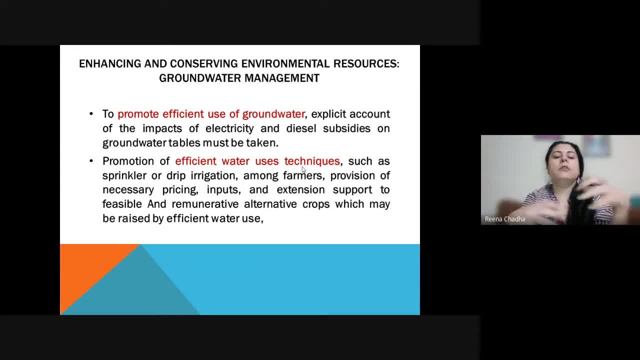 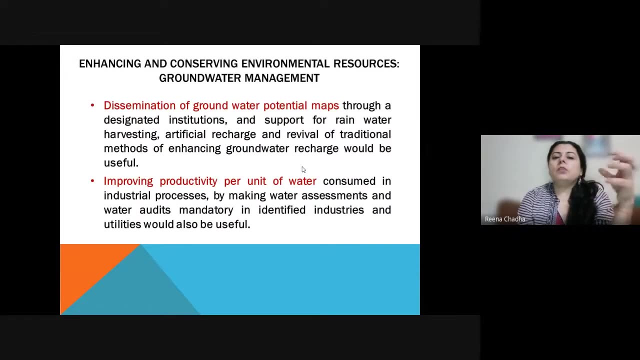 unknown to himalayan regions and to people in himachal pradesh. so those kind of trainings are being given to these people and how they can reduce water consumption in their agricultural fields and farms, and then dissemination of groundwater potential maps. like i have already, 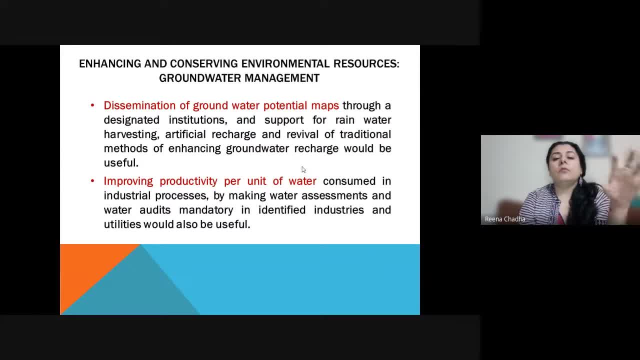 discussed. there is a specific website on central groundwater board main portal and through that site you can identify what kind of areas a new project is coming up, whether it is under exploited zone or safe zone, whether it can be given clearance for groundwater. what are the different kind of pollutants that are there. if there is any threat of cadmium introduction in, 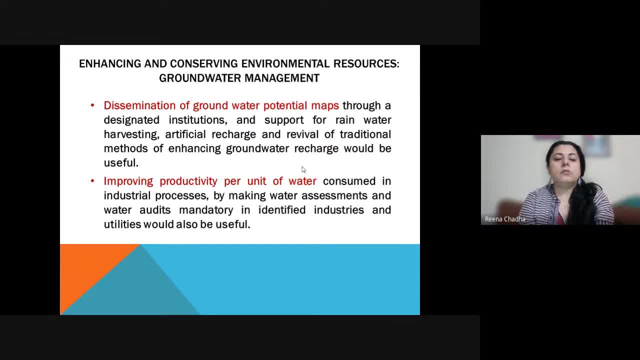 groundwater. if there is any specific heavy metal high level in that area, then improving productivity per unit of water, which we have again discussed before about the specific consumption of resources. so, for per unit of water, what is your productivity? what is your level of per unit production? okay, so what? those kind of assessments are now required through water audits. 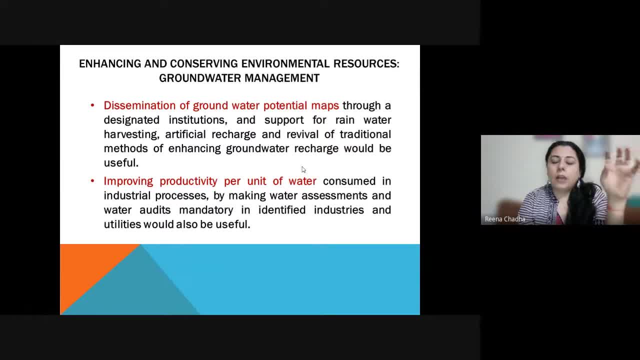 i have already done water audits for uh and housing complex, for a mall, okay, for an institution, and those kind of water audits are being are mandatory. if some industry is utilizing excessive use of water, is doing excessive use of water, then central pollution control board or state pollution control board can demand. 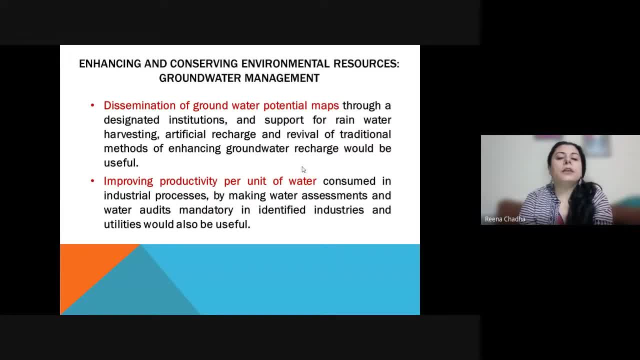 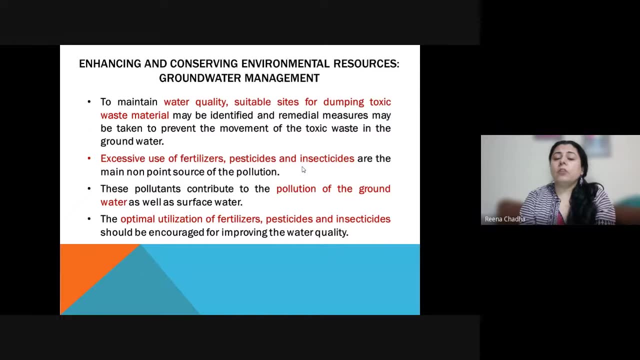 that industry to make their water audit report so that they assess what kind of uh leakages and what of issues are there which is causing wastages in that industry. then, uh, what for groundwater management? also, you have to have specific water quality parameters to be monitored. you have to. 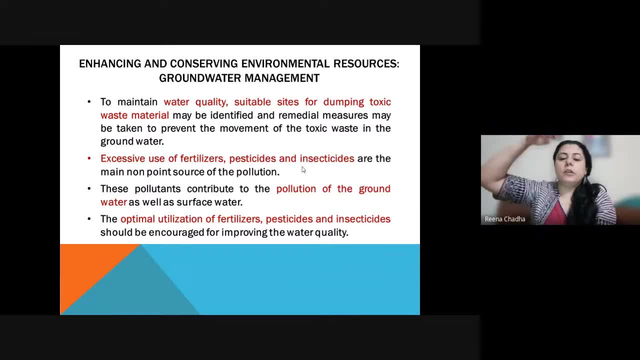 have piezometers. so basically piezometers are introduced along with uh in a similar mechanism, like we introduced your two well pumping machines, so in that piezometer you can get uh take water sample. there is a provision of taking water sample from groundwater through those. 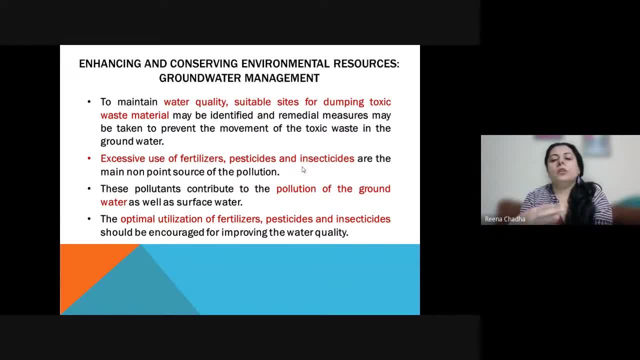 piezometers and monitor the level of groundwater in those areas so that whenever there is an issue, that when, whenever the groundwater level is going down too much, what kind of recharging activities should be introduced can be identified and, if the the industry has to pay for the damage, call. 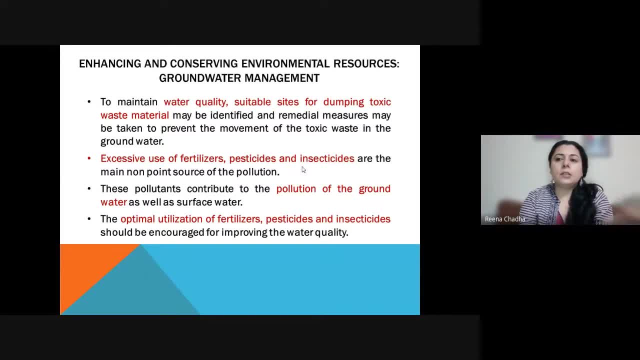 then also it can be identified. so the latest uh, common total solid facility sites or common hazardous waste facility sites, they all are having these piezometers so that they can monitor whether any kind of leachate is polluting the groundwater or not. okay then, wetland conservation is very important because these are some of the 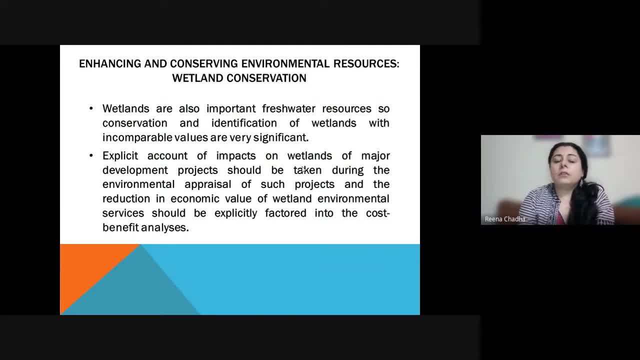 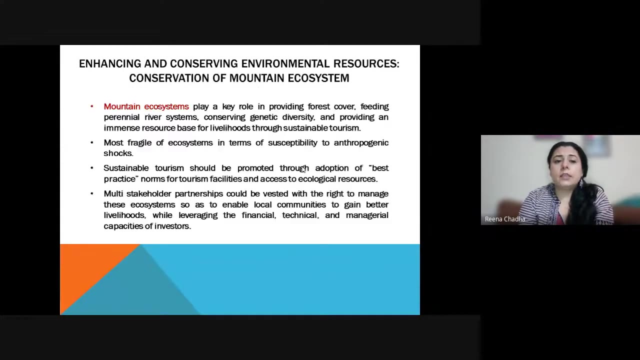 important freshwater resources and they the explicit account of impacts on wetlands under major development project has happened, okay. so to ensure that these wetlands are conserved, we have very strict guidelines nowadays uh. so, especially in punjab, where there are more than five uh wetland areas who are of very national and international significance. 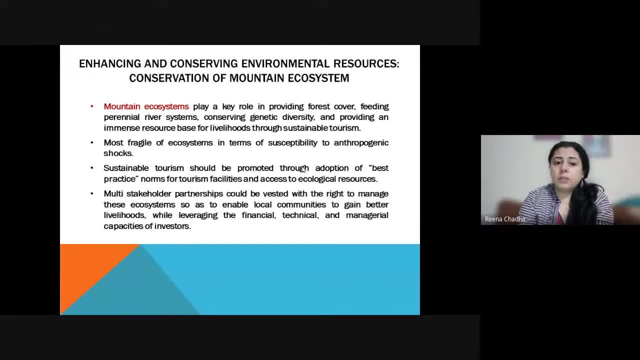 then in mountain ecosystems also, we have specific guidelines and reforms that have been introduced related with sustainable tourism, eco tourism, and what are the best practices where tourism can take place according, in line with protection of ecosystems of environment. so there have been specific guidelines for tourists who are going 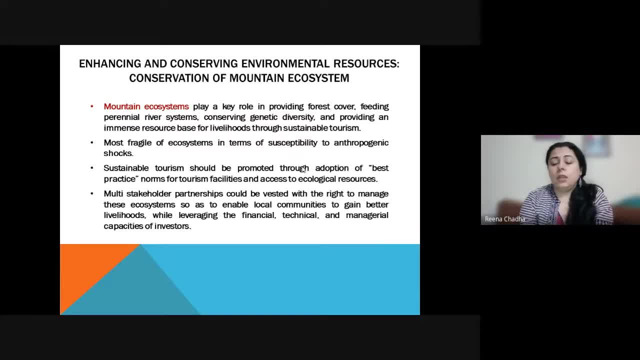 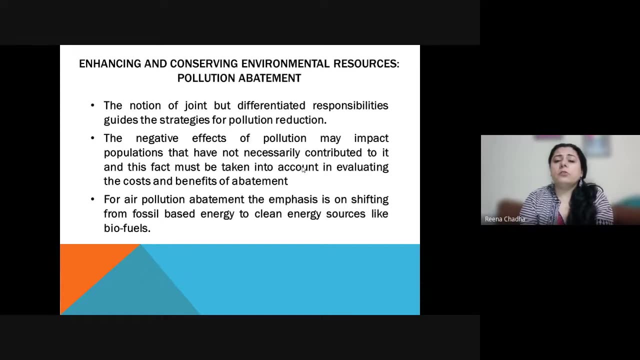 to mountain areas, who are very virgin mountain areas, to ensure that they do not cause any kind of solid waste issue. any kind of plastic waste cannot be just littered anywhere in those areas. then for pollution abatement also, there are specific policies related with clean energy sources like biofuels. so 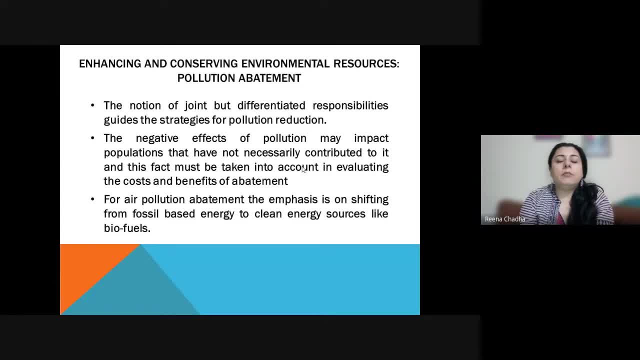 we have also implemented a project with iit monday where they they were given funding for a project where sewage treatment uh plant was used to identify a biofuel. okay, so how a biofuel can be created from sewage? that was their conceptual plan and r? d idea. so those kind of 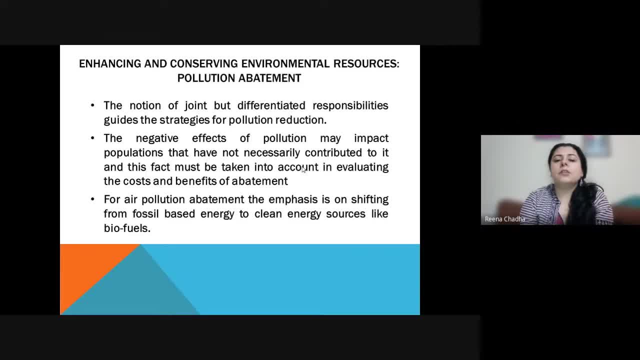 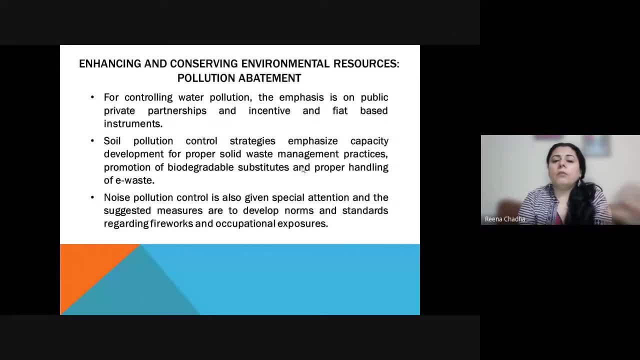 technologies, those kind of advancement and researches are being uh supported through our environment policies. so for controlling water and whatever examples i am giving you are just one or two examples. and many other projects and many other studies are also going on. innumerable number of studies are going on. so i'm just 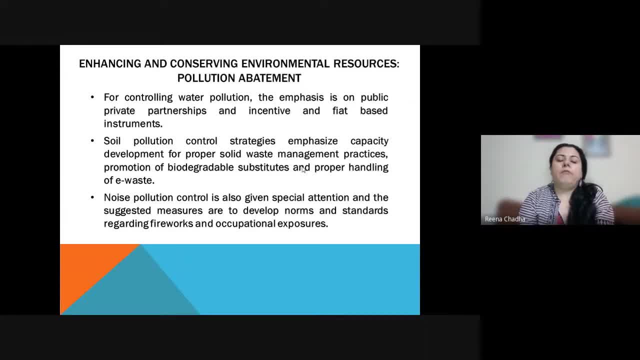 giving you an example, to give you an idea whether such philosophies, whether such principles, which we they have any meaning in ground- so they do have a meaning, they do- are being implemented, implemented practically on ground, and i have myself been in involved in such kind of projects. so again, soil. 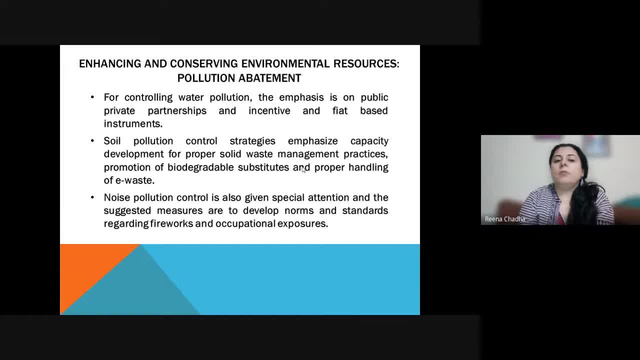 pollution control strategies emphasize capacity development for proper solid waste management practices. that's why, to control soil pollution nowadays we have to take environment clearance even for a solid waste management plan or for a net, as well as for a solid disposal facility or even for a scientific, scientifically designed. 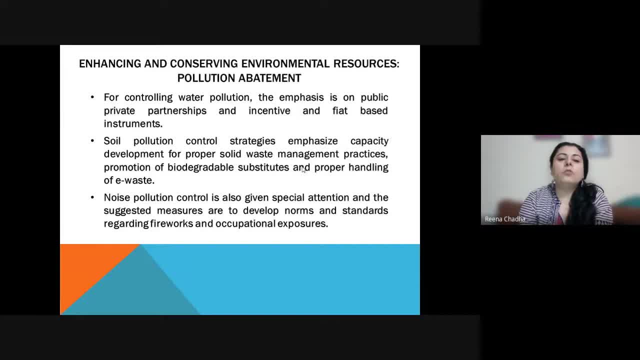 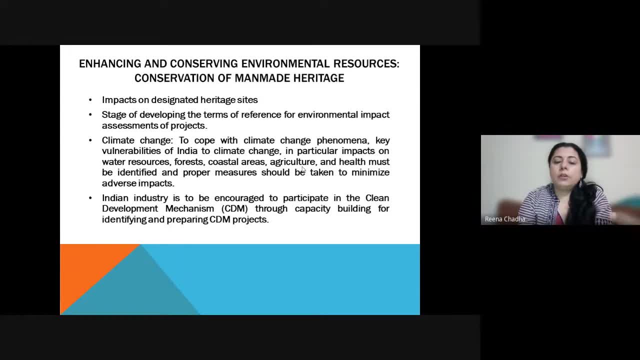 landfill. also, you have to take environment clearance so that you do not cause any soil pollution, groundwater pollution, air pollution or noise pollution. and again for conservation of heritage sites. for example, if if i am going to develop any kind of heritage site and convert it into a museum or convert it into any hotel, i have to conserve the 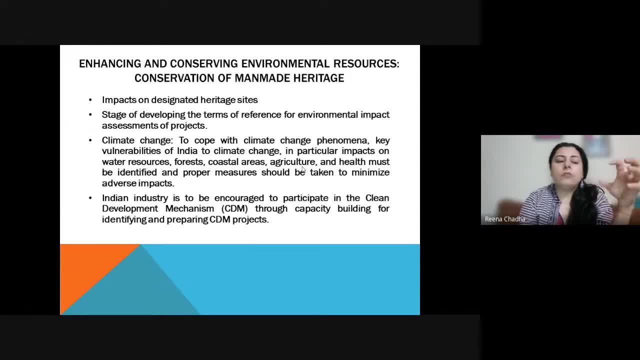 additional uh construction activities or i have to conserve the original construction materials which were utilized, like uh. in punjab there is an extensive use of shahi bricks. these are thin, uh sized small bricks and these bricks are made from clay material through uh indigenous techniques of mortar and through indigenous techniques of like uh. we have a smaller version of those. 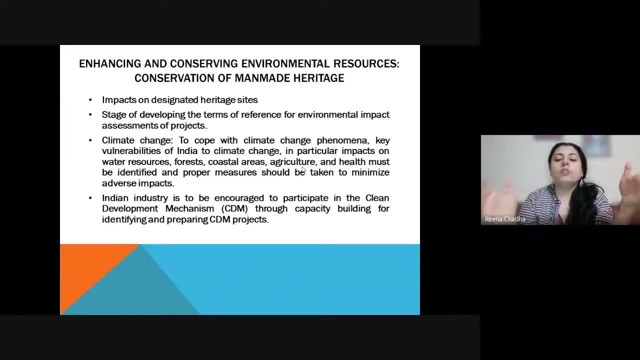 techniques like we ground wheat into floor through chukkis. so those kind of big chukkis were used for developing construction material in those days in uh for for our heritage sites. so nowadays if you are doing conservation activities in these heritage sites you have to conserve the original construction. 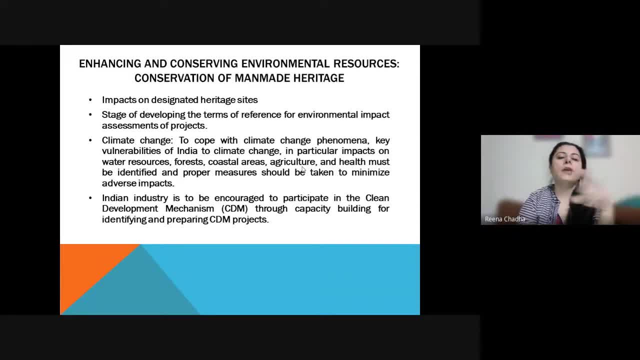 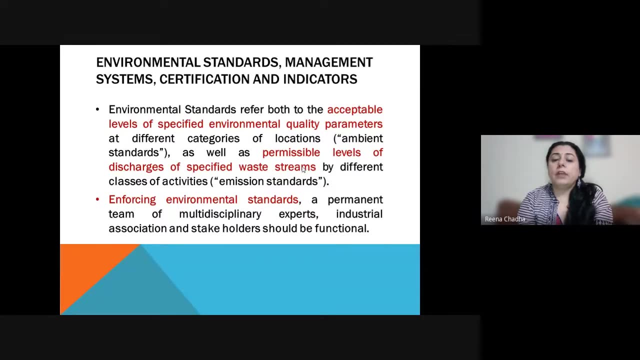 material. you have to again conserve those shahi bricks and utilize them again to refurbish or re reconstruction of those kind of heritage sites again. uh, for certifications indicators, we have environmental standards which refer to both acceptable levels of specified environmental quality parameters and which also specify permissible levels of discharges. okay, so these environmental standards are being implemented. 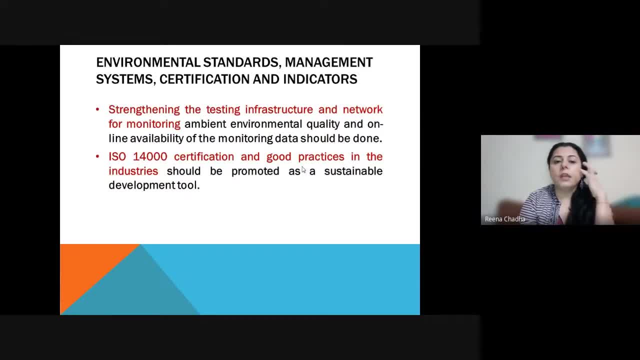 through the apps and guidelines which we have already gone through in the last lecture and i suppose that they help the Erin Lohse question as well. sorry for not being able to hear as quickly as possible now how we try to define these environment standards is given later and said: 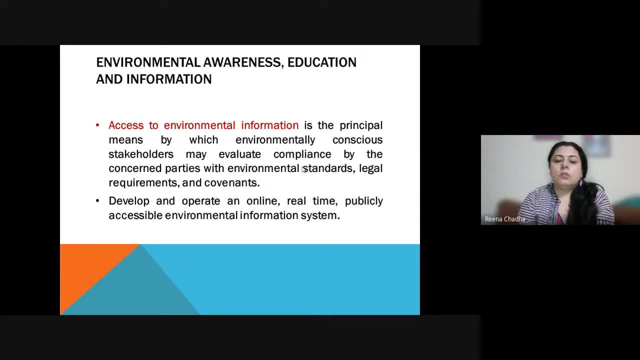 so these are, according to the 아나젠다 and the AUA statistics of this we also use really well under stepped magazines, basically where click among within comigo. we really try to distinguish between the requirements of this in a way that is like less of a. 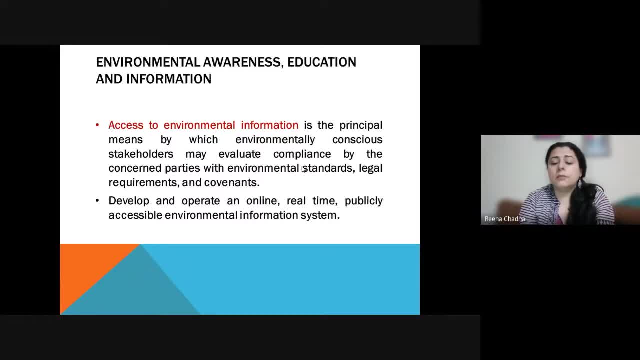 integrative. really good at explaining what's going on in these outcomes is in these activities, so so, so yeah, they tastesh Producer So that all the school children they are having important information about environmental protection, about the requirements, why there are so much environment related problems, about climate change, And there is a real time online information system. All the STPs- sewage treatment plants, effluent treatment plants. they are connected with the continuous environment monitoring system, CEMS. 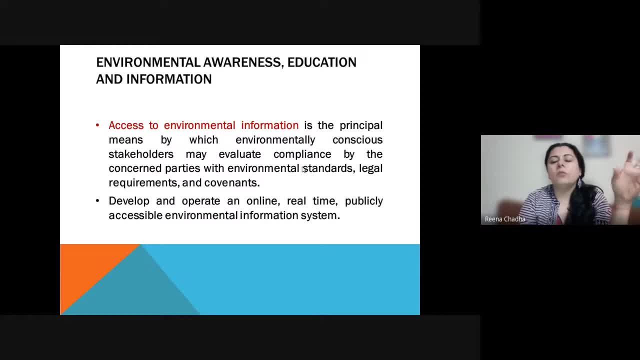 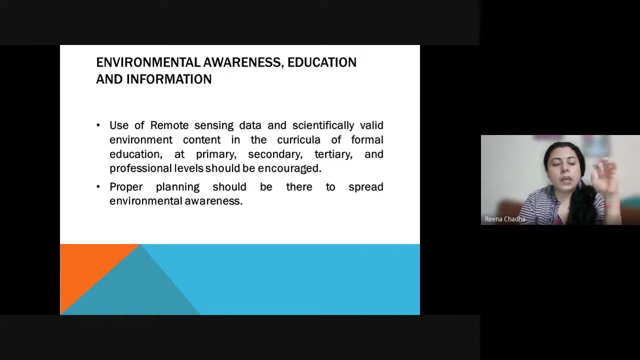 So these are also again in central pollution control boards- guidelines And all those parameters which are being monitored in those centralized environment monitoring systems. they are being transferred to their local pollution control boards through online access. Okay, so there is a continuous transfer of data from industries which are having higher risk of causing pollution directly to the pollution control board, so that there is any ambiguity. 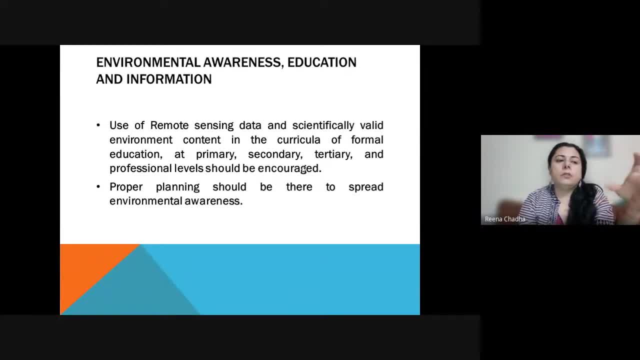 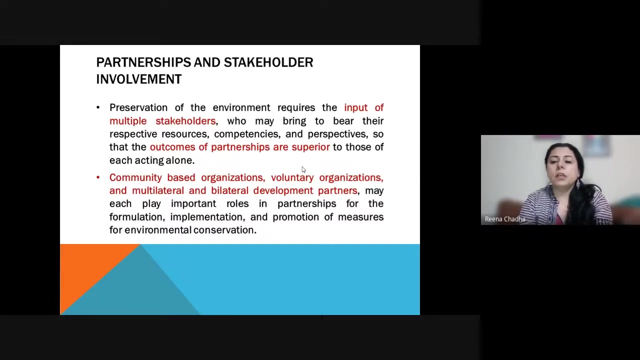 Okay, so there is a continuous transfer of data from industries which are having higher risk of causing pollution directly to the pollution control board, so that there is any ambiguity. Okay, so there is a continuous transfer of data from industries which are having higher risk of causing pollution directly to the pollution control board, so that there is any ambiguity. 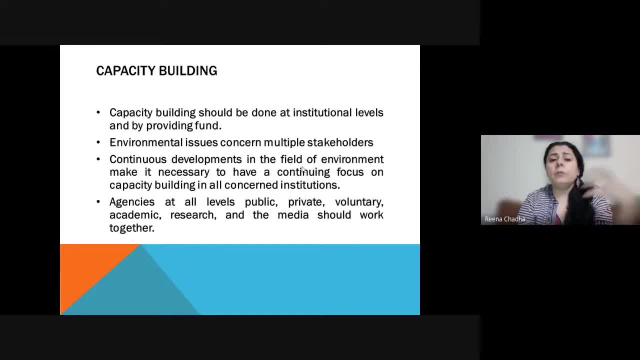 Okay, so there is a continuous transfer of data from industries which are having higher risk of causing pollution directly to the pollution control board, so that there is any ambiguity. Okay, so there is a continuous transfer of data from industries which are having higher risk of causing pollution directly to the pollution control board, so that there is any ambiguity. 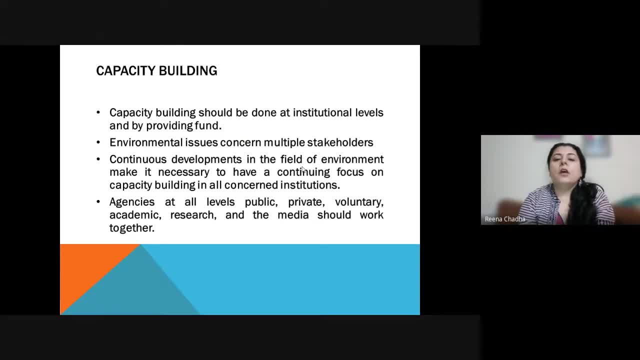 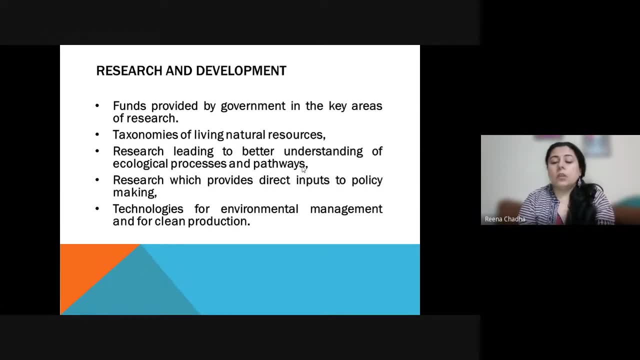 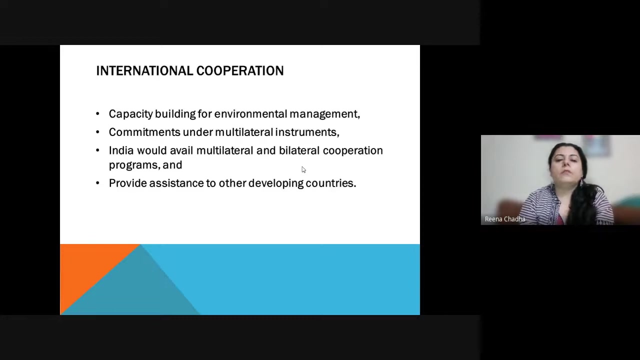 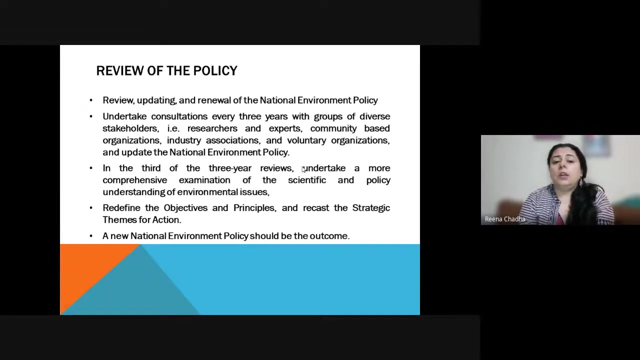 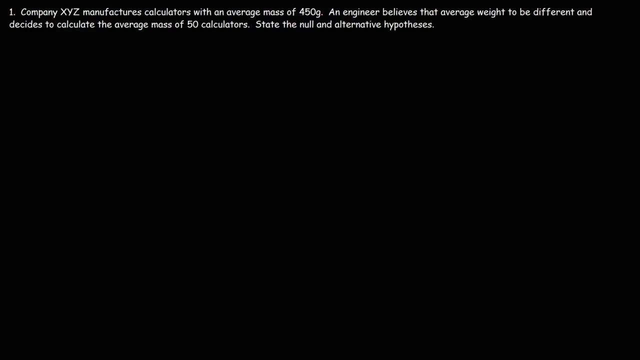 In this video we're going to do a brief introduction into hypothesis testing, but specifically on how to state the null and alternative hypotheses. So let's start with this problem. Number one company, XYZ, manufactures calculators with an average mass of 450 grams. An engineer believes that average weight to be different. 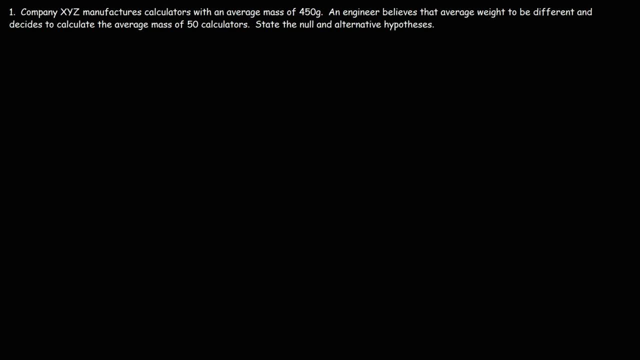 and decides to calculate the average mass of 50 calculators State the null and alternative hypotheses. So let's start with the null hypothesis. The symbol that corresponds to the null hypothesis is H sub zero. Now the null hypothesis is basically the status quo. It's the claim. 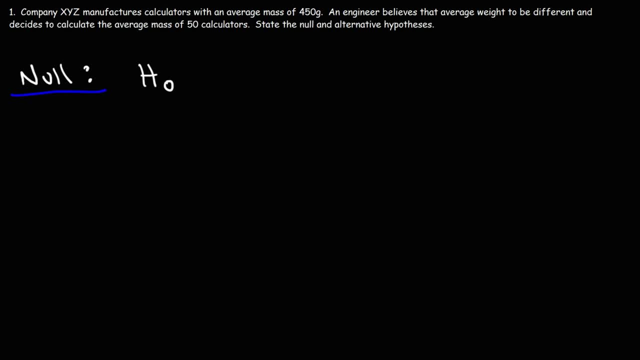 It's the current accepted value that the null hypothesis is the status quo. It's the claim, It's the current accepted value that the majority of people holds to be true. Now the alternative hypothesis is basically the contender. It's contradictory to the null hypothesis. It has a symbol: H sub eight.